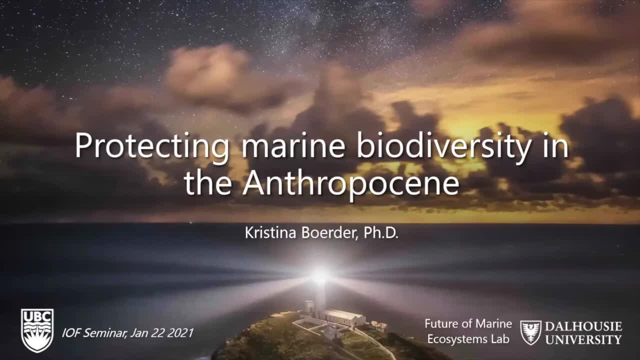 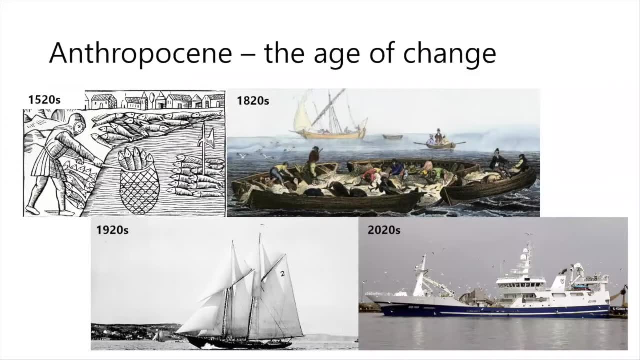 much looking forward to hearing your thoughts and the discussion afterwards. So I'm really preaching to the choir. Thank you so much for being here, because there's a lot of amazing research and knowledge coming out of UBC on that end. But I would like to start very broadly with some thoughts. 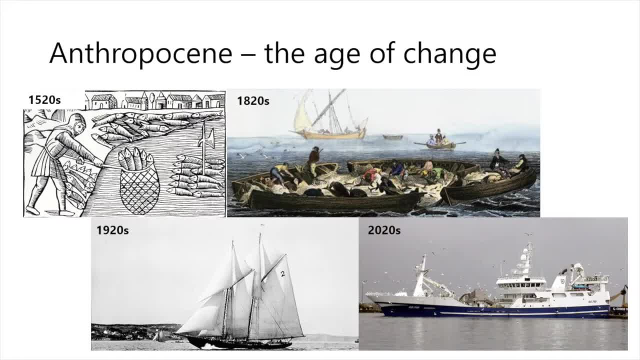 on the Anthropocene as the age of change and the age, especially, of rapid change, Illustrated here with different fishing techniques over the centuries, starting in the 1500s or 1520s, very manual labor, intense and, yeah, of course, very different styles. I don't know what the 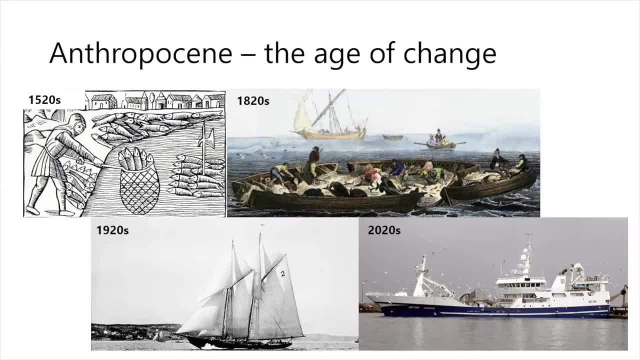 pike in the middle of the fish in the right of the picture is doing, but I'm pretty sure it had its reason: Two more boat based fisheries, all under sail and manpower in the 1820s. In this case the depiction is with dip nets fishing for tuna. And I'd also like you to. 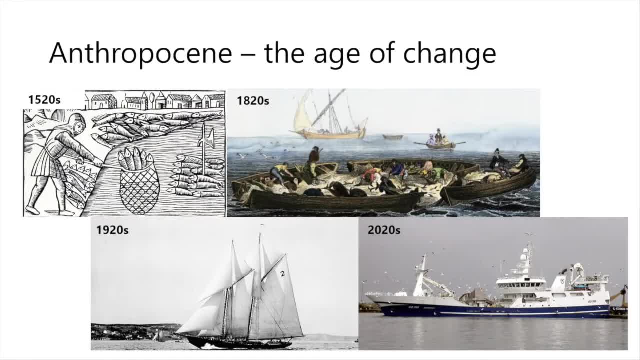 know what, the fancy ladies in the background watching the fisheries To the 1920s, where still a lot of the fishing really happened from bigger schooners under sail. And then, as a little trivia bit here, if this boat somewhat looks familiar, you may have another. 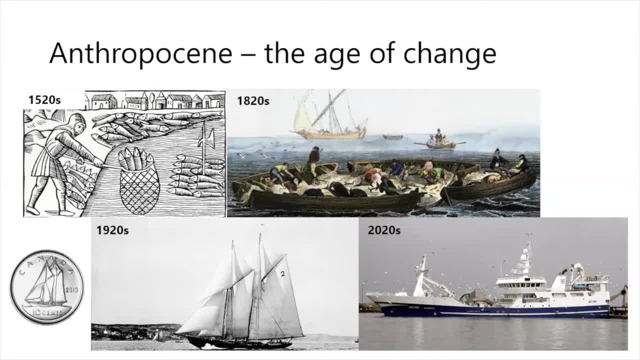 look at your 10 cents coins, the Canadians at least. This is the Nova Scotian Blue Nose. At that point, the fastest sailing schooner that won several noted races and a rebuild can still be seen in Nova Scotia sailing up and down. Highly recommend when travel is. 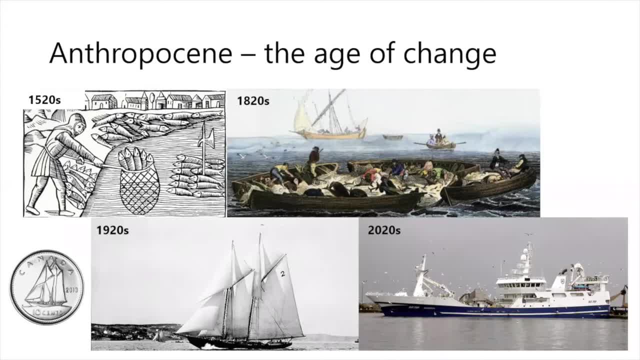 possible again To, of course, the 1920s- 2020s. now we have the industrialized fishing, Which really is quite decoupled from this history, with high tech equipment, fish finders making use of helicopters, satellites and, of course, under enough power to go as long. 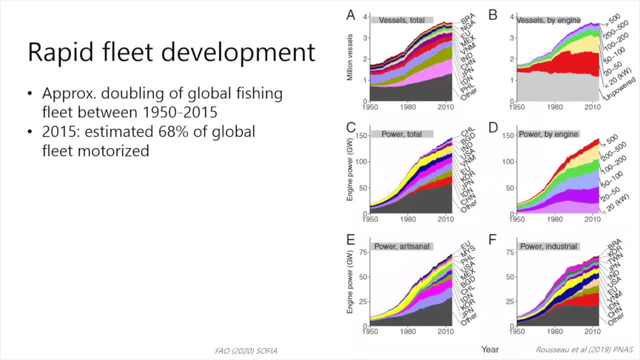 as and as far as needed, And that really is illustrated by this work by Rousseau et al- from 2019, who looked at the rapid fleet developments and found that the global fishing fleet's roughly doubled between 1950 and 2015,. as you can see in panel A, And most of these 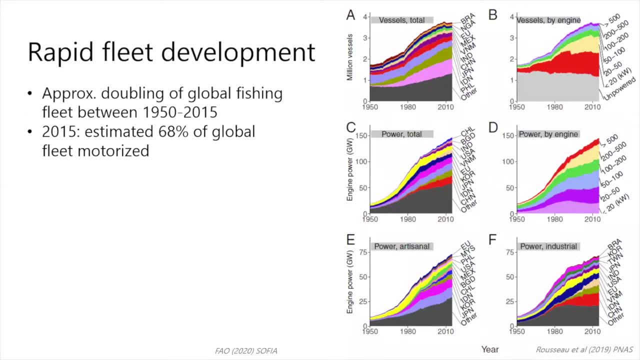 actually by 2015 have been motorized not quite 70%, which still leaves a quite a significant amount of vessels that are not under power. But you can see how quickly the uptake of motorization of different powers- power- yeah amounts- have been going in panel C and 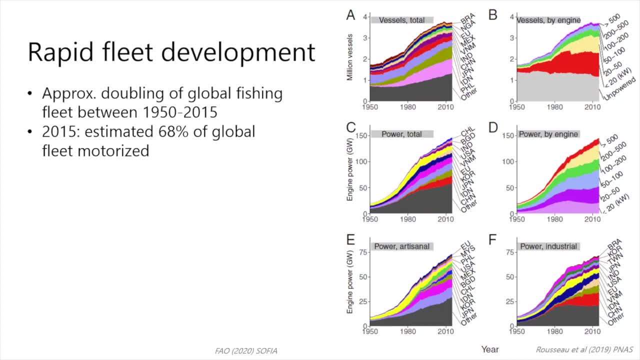 further on between industrial and artisanal fleets, And this is probably some a graph that all of you have seen, once or twice at least. So this motorization really has enabled the vessels to go further, to fish longer and to access fishing grounds that were not as 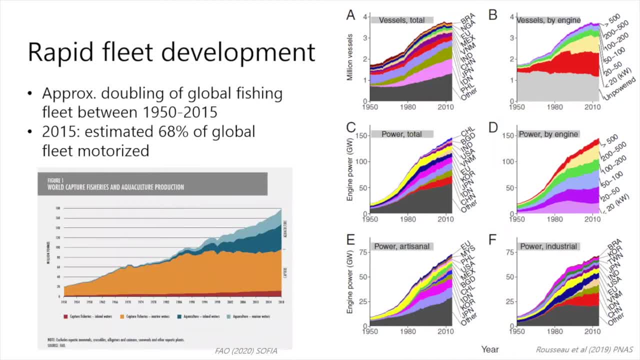 easily accessible before. However, after quite a noticeable increase of catches since about the 1990s, catches are stagnating. This is the orange curve shown shown here. This is the yellowish curve shown. So, despite fishing further, fishing in new places and fishing, 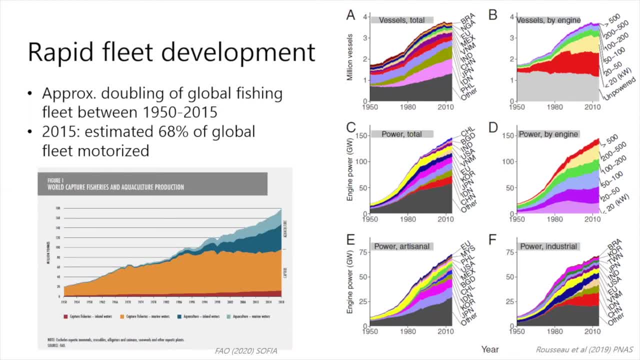 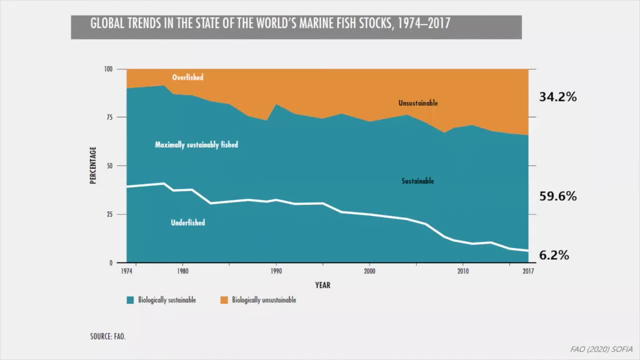 harder, not more. the vessels are not catching more, So this, of course, comes on the background of increasing overfishing, And, no matter how you name it, about a bit more than one third of the fish stocks are unsustainably fished and classified as overfished, whereas about 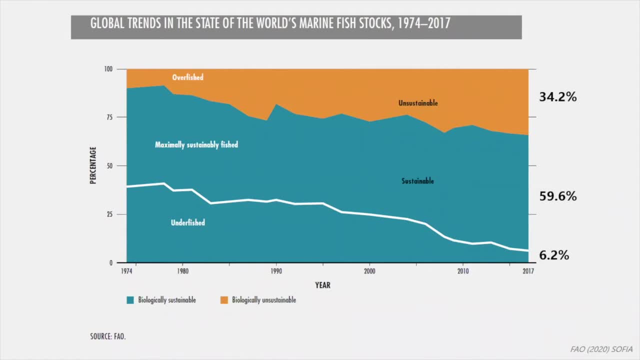 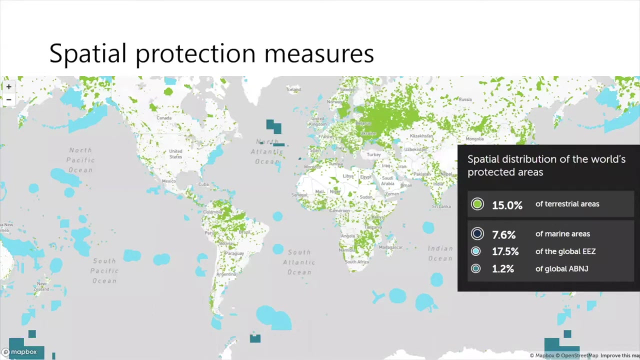 60% are overfished. And also, the other thing that is not really clear is that the number of fish stocks that are massively, sustainably fished and a steadily decreasing amount, can be classified as underfished, which is just above 6% currently. So, on this scenario, of course, spatial protection measures. 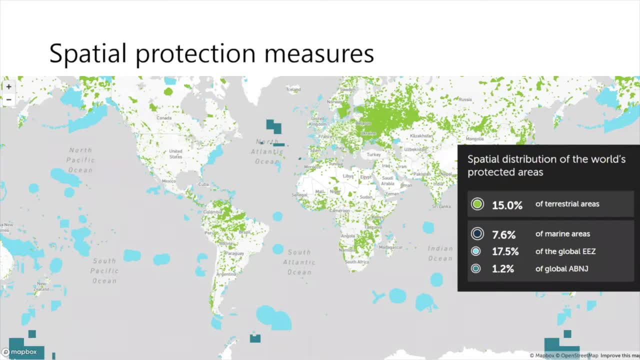 are coming into this discussion and have been more and more a broad feature of the discussion around management, sustainability and conservation. of course, This screen grab was taken from the latest World Database on Protected Areas and shows that we on land have currently about 15% protected and for the oceans we are around 7.6%. That 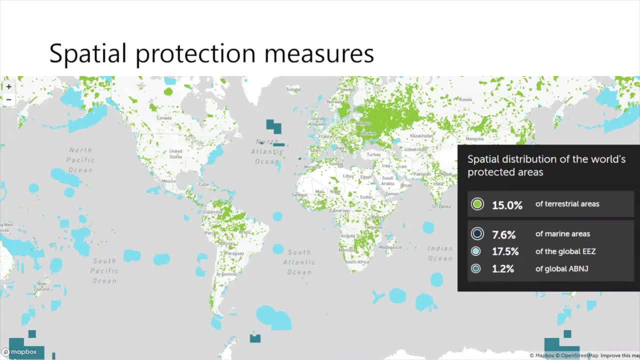 number, of course, is open to a certain amount of debate regarding what one considers protection, But regardless, most of it is focused on the exclusive economic zones of countries and the high seas, the global here, areas beyond national jurisdiction, ABVs and so on. So 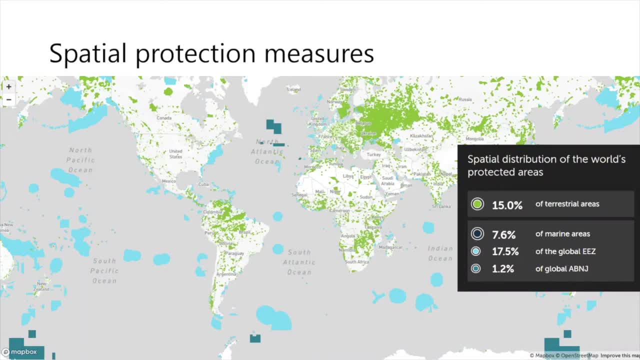 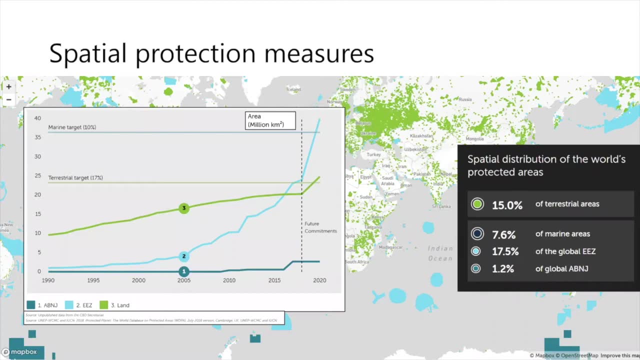 this is a pretty recent trend, as you can see here over time, especially denoted by the light blue curve and, to a certain degree, by the darker blue one. The marine protection really has been pushed forward about the last two decades. So this is a good development, definitely, but if we look at how biodiversity is doing, 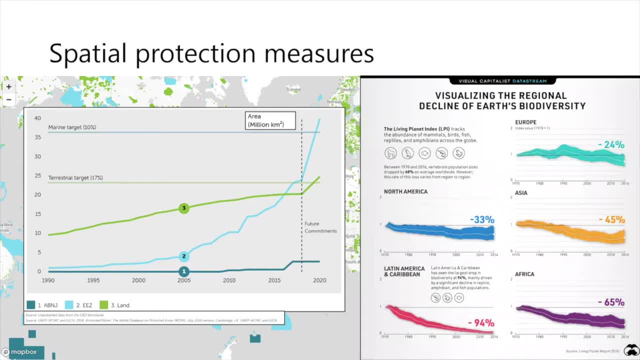 and this is a more overall trend, of course, including terrestrial. despite more protected areas, we continue to lose biodiversity at rapid rates, And here you can see some of the rates are really concerning, as presented by continent, And right now, these features. 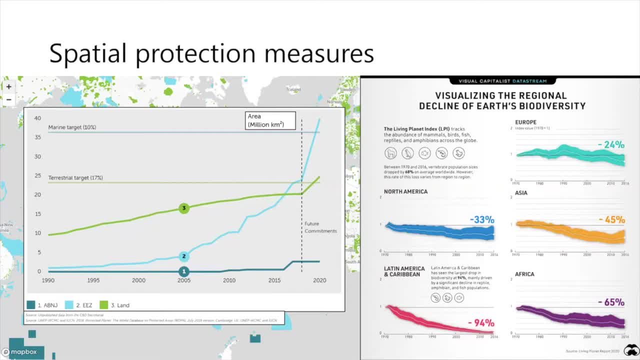 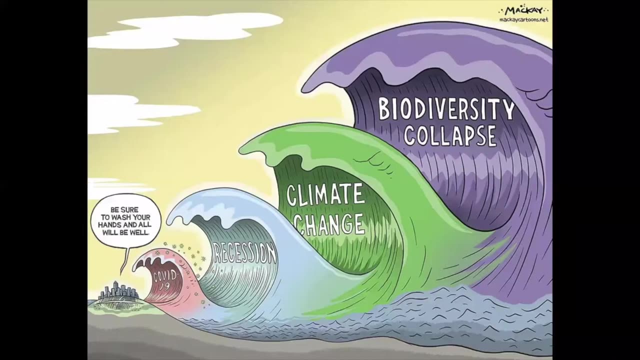 the conservation as we've been doing it and seeing it has been largely reactive and aimed at really slowing down this decline, so focused at losing less, And I find, on this background, this comic or cartoon really hits home, especially regarding now. So we are facing oncoming waves. 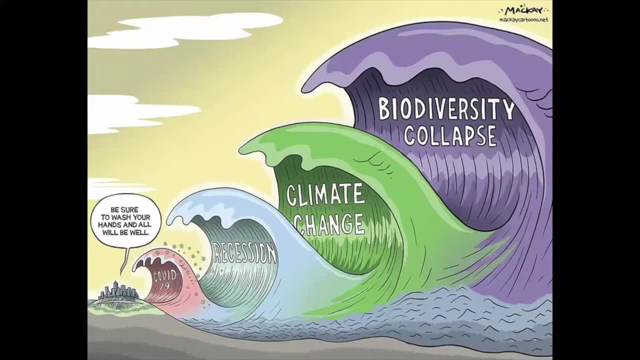 and we are right in the middle of the COVID wave, of course, but there's more coming, and climate change and biodiversity collapse are really the looming waves on the horizon, And so I think we really need to be thinking about how we're going to face these waves and with what attitude, which hopefully goes beyond. 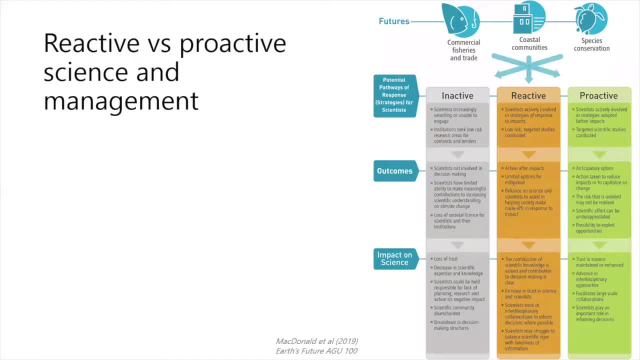 hand washing and all will be well. So I'd like to spend a short time on talking about how we approach this kind of science before jumping into some novel and ongoing science, And I really like this publication by McDonald et al from 2019, with thoughts on different. 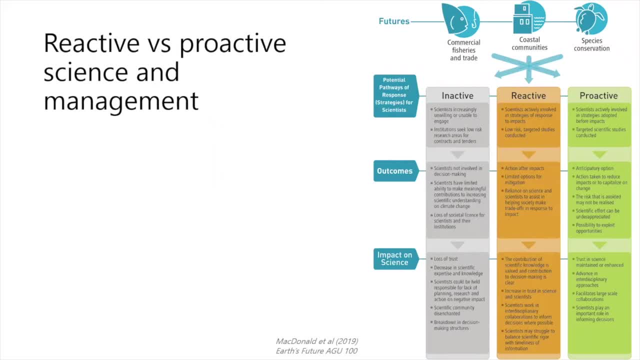 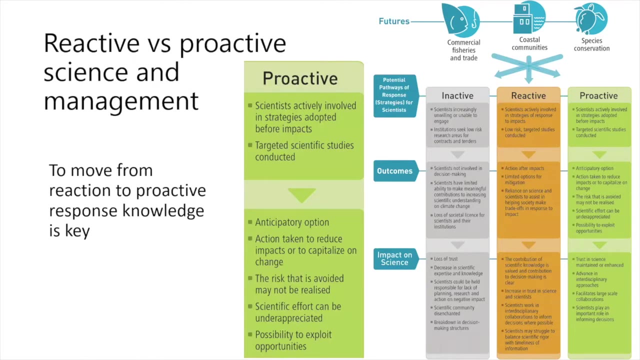 types of approaches for science and fisheries management, From inactive approaches to very reactive management and science to the proactive approaches. and realizing that this might be a bit small on your screens, I would like to highlight the proactive approach they have phrased here, which is really scientists. 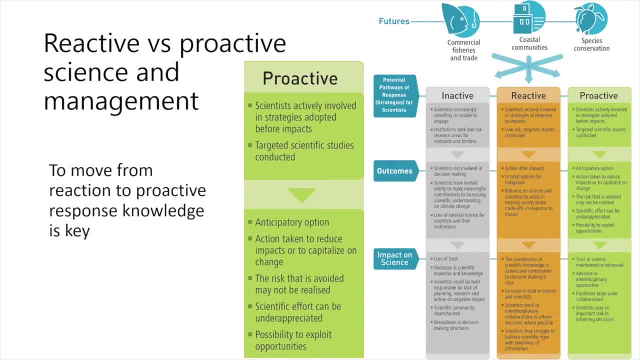 actively participating in decision making and actively targeting studies to provide data and knowledge That can be applied And really supporting the anticipatory option so that actions can be taken to mitigate any negative impacts or even, as they say here, capitalize on change in in a wise way. 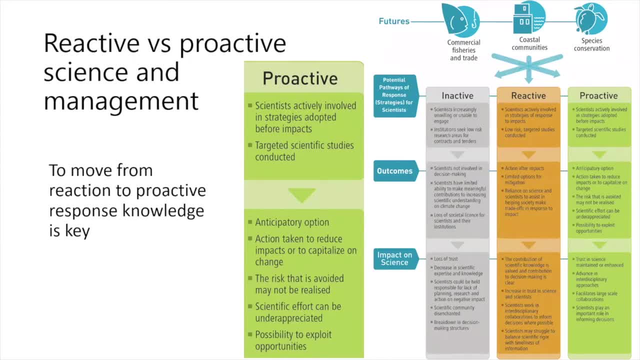 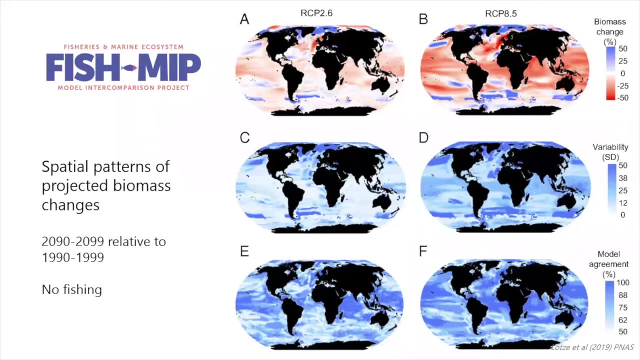 So really, what I want to stress here is to move from a reaction to a proactive, wise response. knowledge is key, And there's been a lot of good knowledge looking ahead regarding what is to come for the aspect of climate change and this. that would definitely be too much. 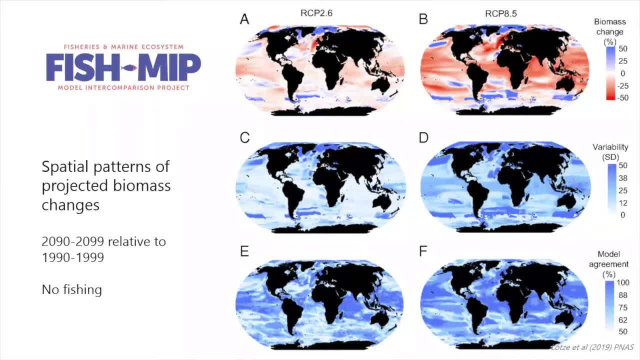 to be talking about all of this. so just an example from the fishermen project, the fisheries and marine ecosystem model into comparison project here, taken from lots at all 2019, presenting two different scenarios for two different climate change scenario, so 2.6 and 8.5, the 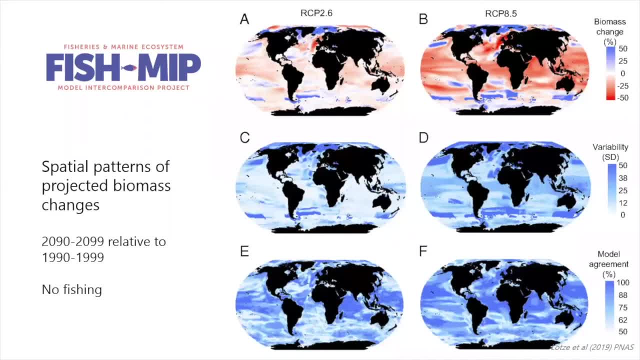 spatial patterns of projected biomass change. So this is 2090 to 2099, relative to 1990 to 1999 and does not consider fishing. but especially if you look at the upper row panel panels a and b, You can see that the biomass change is obvious for both scenarios and will mostly impact. 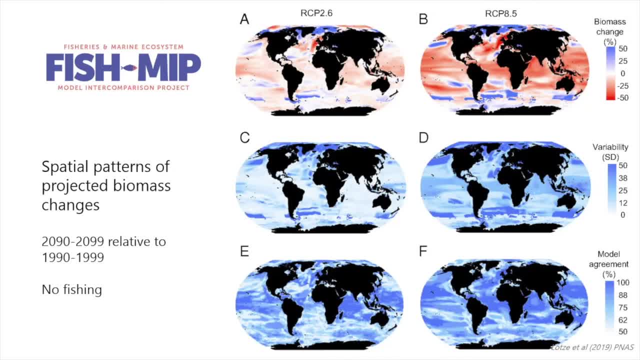 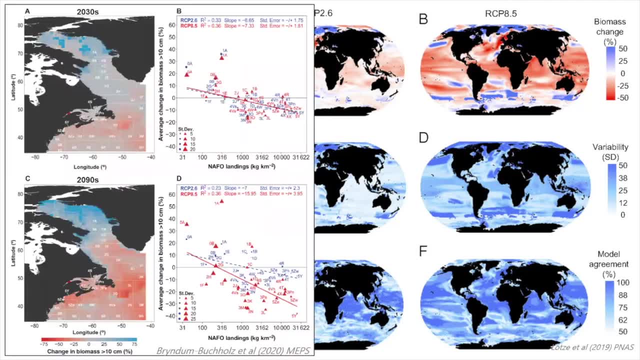 of course, the equatorial and temperate areas, whereas an increase of biomass is expected for the polls. And if you take this a step further, As was recently mentioned, It was recently published last year by Brennan Buchholz at all- to really look at what does. 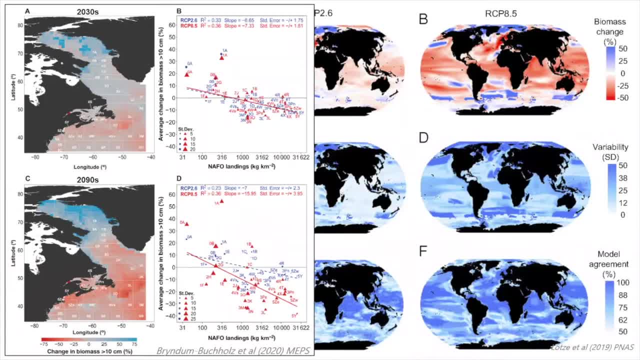 this mean for, for example, fish catch. so this is a study looking at changes of fish catch for the 2030s and 2090s for the now for area. so North Atlantic, here around Atlantic Canada and Greenland- you can see that a lot of different areas are expected to have declining. 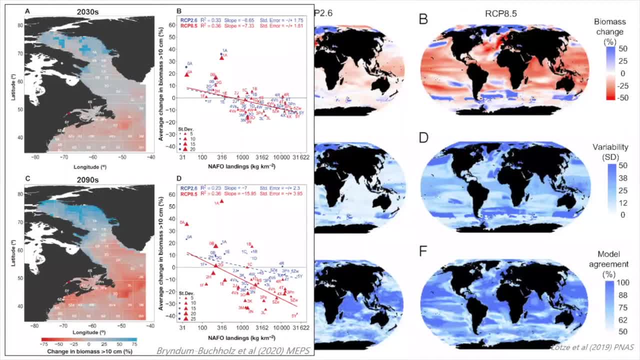 catches, especially focusing on the traditional areas Here around the Grand Isle, Here around the Grand Isle, Here around the Grand Banks, which is the dark red in the 2090s area. so and of course, developing fishing grounds for the Arctic and high Arctic, which is currently under. 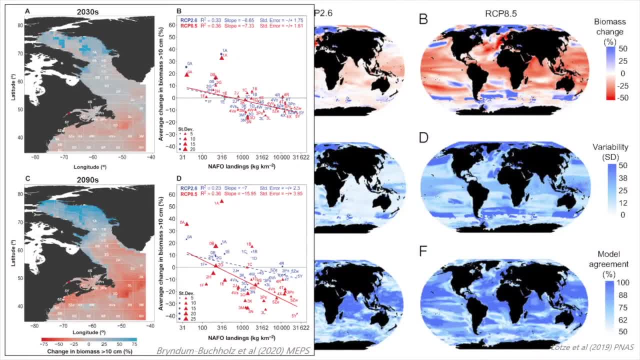 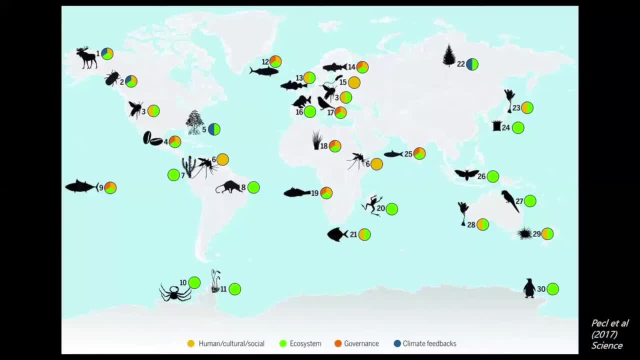 protection, but this needs to be considered if we talk about further protection for the Arctic areas, And this, of course, correct directly correlates to species being on the move. So this is just a rough example of some terrestrial And marine species that have been found to shift and have either moved for the north. 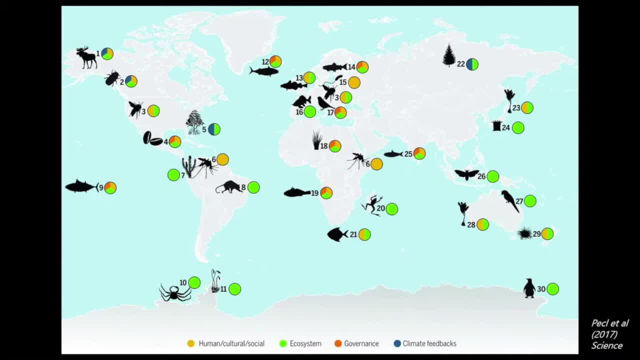 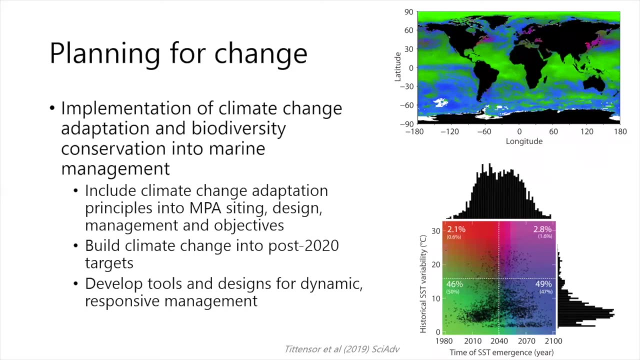 or further, to further down for marine areas of further up into cooler climates for terrestrial. And knowing this, we need to figure this in because we need to start planning for change if we want to move from the reactionary approach to a response, responsive, wisely responsive approach. 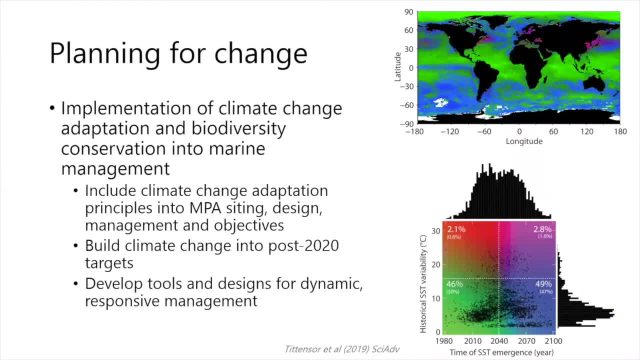 And we've been considering, we've been had, We've been considering, We've been considering. It was considered a very interesting workshop a couple of years ago, with some people also from us present, and we discussed how this can be approached for marine conservation. 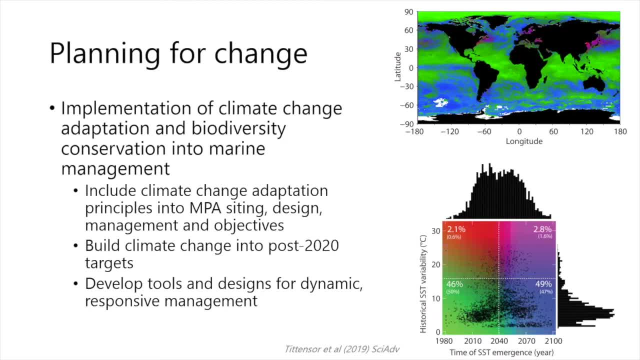 and in the upper map here you can see here a map. here you can see the colors representing historical sea surface temperature variability and time of sea surface temperature emergence diverging from pre industrial levels. so the colors correspond to the lower graph And you can see that there's a fairly good spread. 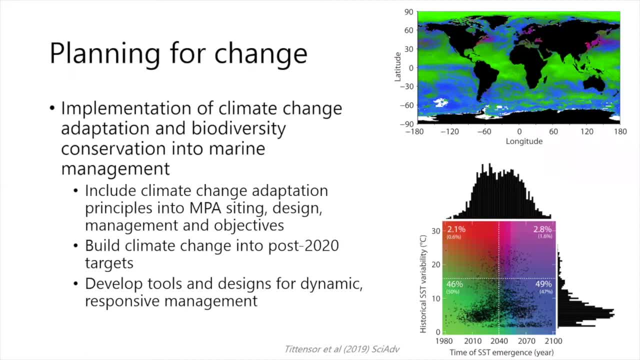 regarding when sea surface temperature is expected to diverge, but also- and that is referring to the lower panel- the locations of marine protected areas across the spread. So this is depicted by the dots in the box itself, but also represented by the histogram on the outside. 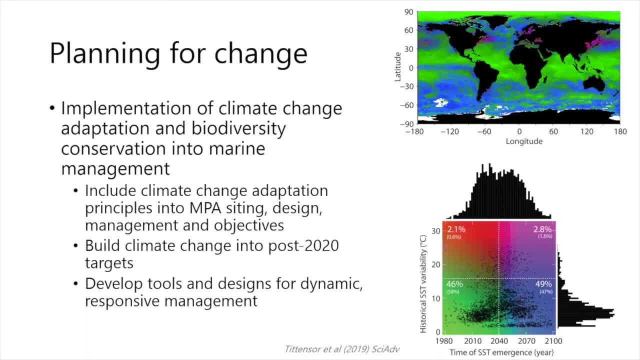 And, as you can see, especially regarding historic sea surface temperature variability of the areas, we've got a pretty big skewed data regarding- or not skewed data- skewed locations of marine protected areas regarding historical variability. So this can have direct implications, of course. 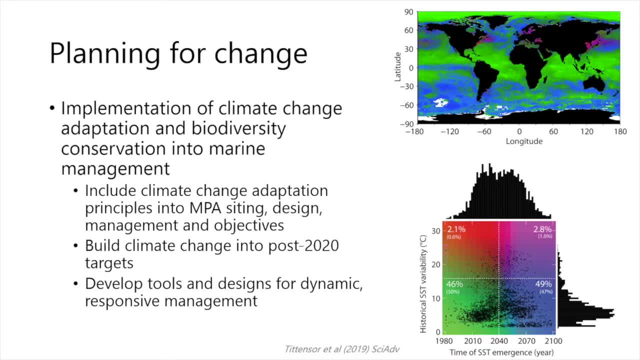 how stable and how vulnerable ecosystems might be regarding changes of temperatures to come. So knowing these kinds of things really helps us to implement climate change adaptation and biodiversity conservation in marine management and especially include climate change adaptation principles into not only the MPA siting, which is addressed here. 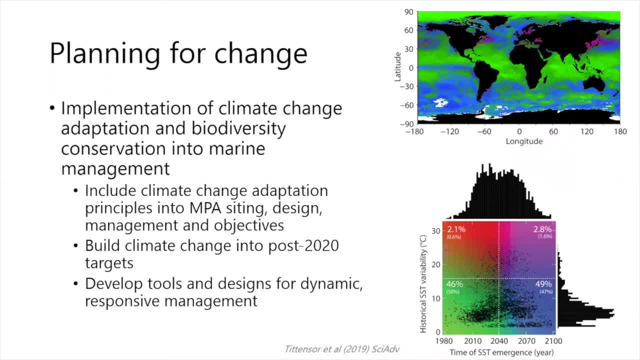 but also the design, the management and, of course, the objectives, And we're really at the start of this. We've done a quick overview or a survey of how many protected areas really incorporate climate change into their management plan, And we've come up with only a handful. 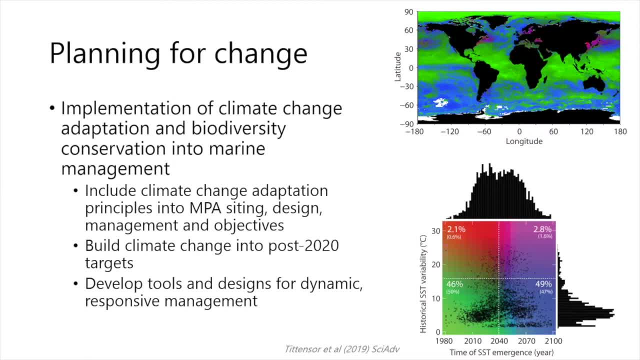 of examples. So this is really at the start, right now. Then also to build climate change into post 2020 targets. with the period we've just started, and having participated in a couple of international meetings, I was personally fairly disappointed how little climate change really is taken into account. 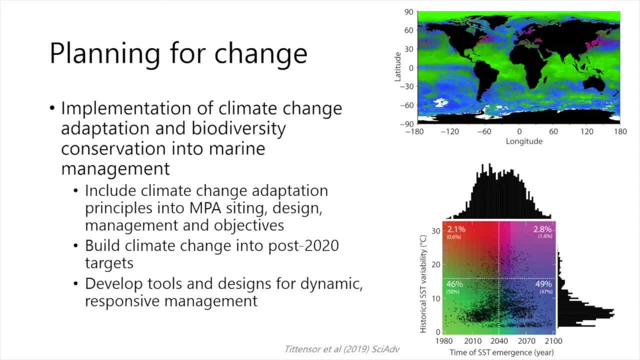 So it's the elephant in the room that no one really wants to talk about because it's so hard to address and there's no good guidelines on how to do this. So we really need to work to develop the tools and the designs for dynamic and responsive management. 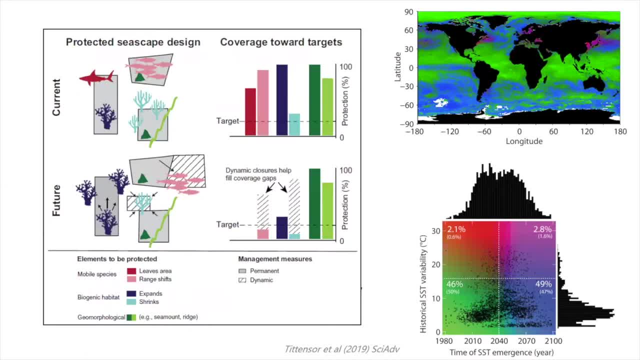 And coming out of that same publication, we're making a couple of recommendations how this can be done, of course also considering policy and legal anchors, and suggest a couple of ideas how, for example, dynamic management can be used to supplement and expand the current static marine. 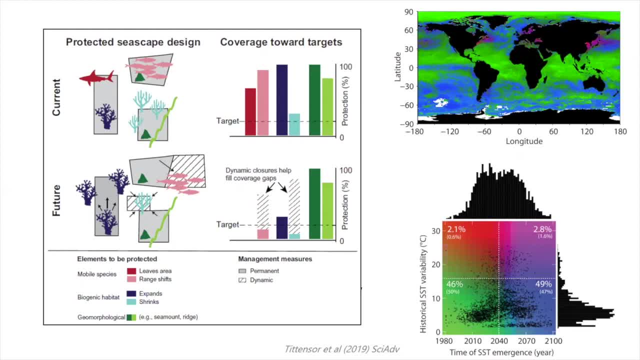 protected area feature Because, as you can see in the upper lines, the current the network of course has its targets and covers these targets to a certain percentage, as shown in the bar graph. But if some of these species or ecosystems move, 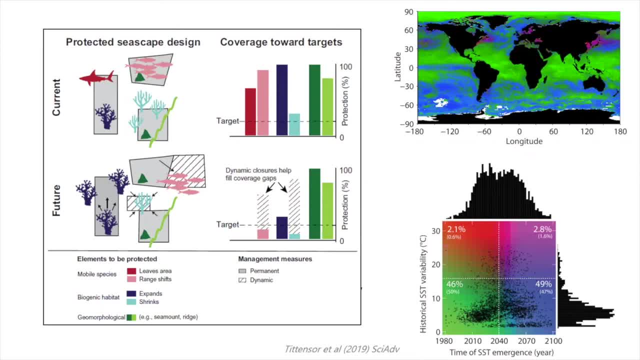 these targets will fall short. So we have a suggestion on dynamic ocean management areas that might be used to expand this network. So similarly has already been done, for example here on the Canadian East Coast with the North Atlantic right whale closures. So this would be more seasonal to what 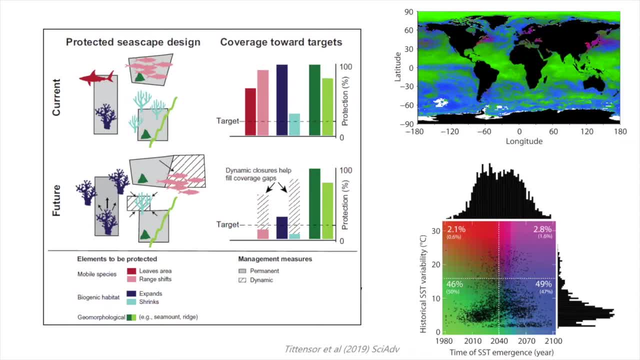 we call climate responsive biodiversity closures, which would be a hybrid between a seasonal and an MPA that can be put in place for certain amounts of time until objectives are being re-evaluated and re-measured, for example, to track ecosystems on the move. 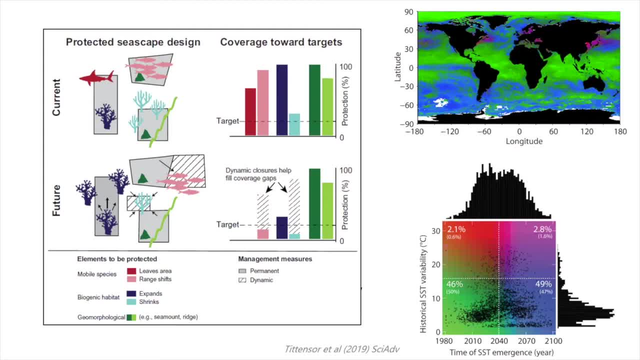 or species on the move. So if you're interested in that, this is the current focus of the work of our lab here at Delahunty. Thank you, Delahunty. So I'd like to switch gear a bit from looking into the future. 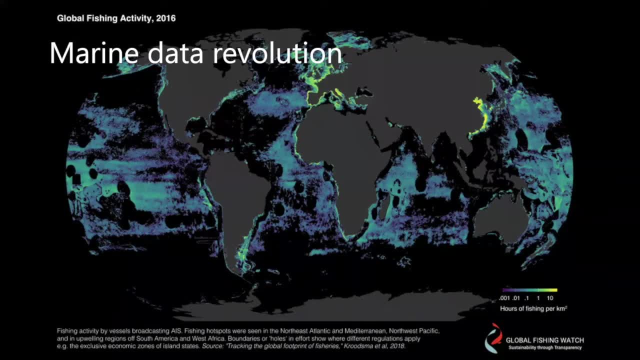 to looking at the human impacts we have right now, which is right in front of our noses, and talk a bit about the marine data revolution, as I'd like to call it, that the AIS data has brought. So in the background, you see a map of global fishing effort. 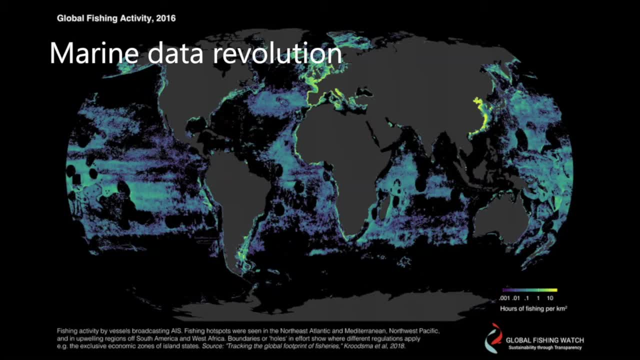 for the year 2016,, which we published, I think, In 2018.. And this is an effort for a whole year, covering about 55% of the global ocean, And it comes from a tracking device called AIS, which stands for Automatic Identification System. 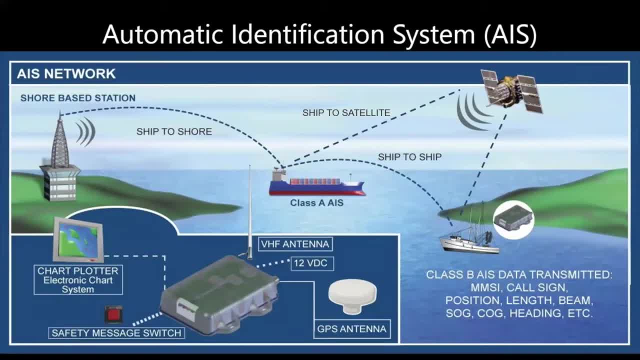 It's a transponder on a vessel that sends information about the vessel, such as type of vessel, position, speed over ground, course and a variety of other information, mainly to other vessels in the first line, because it's a tool for navigational safety. 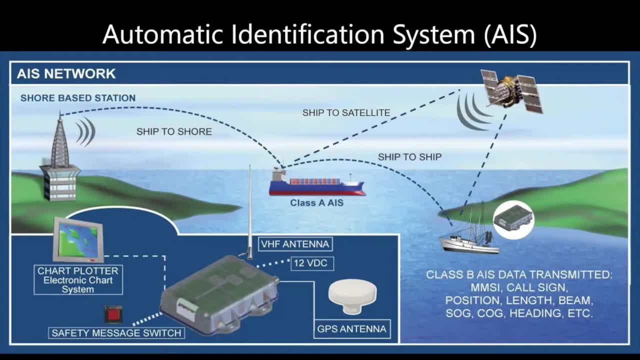 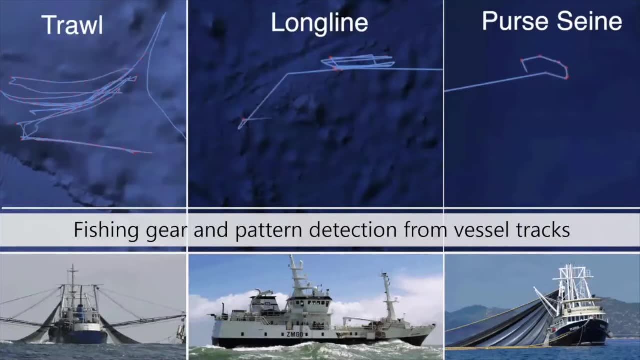 But these signals can also be picked up by satellites or towers And we can use this kind of information, similarly to tagging animals, to follow their tracks and really see what the vessels are doing. And just to give you an example of what this looks like, 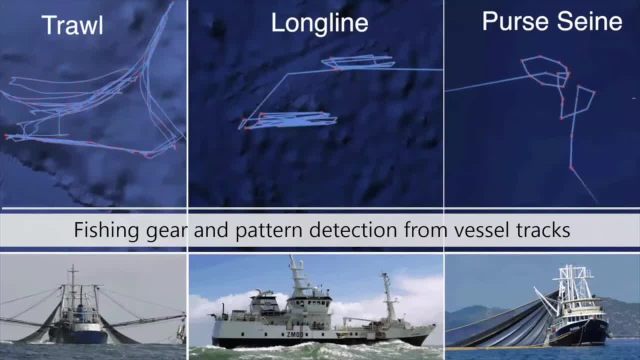 and how we can use these tracks to not only classify what type of vessels- or in this case, what type of fishing vessel with what type of fishing gear it is, but also its activity Activity- mostly, of course, traveling versus fishing. And you can see here for the first panel. 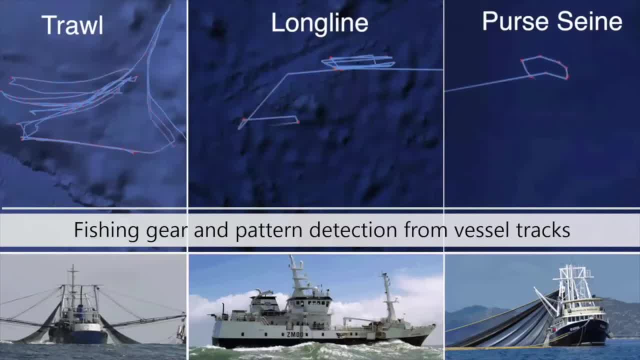 the trawlers have these long swooping patterns when they drag a net through the water column or across the seafloor, And, compared to longliners that set a line, usually at fairly high speeds, the line can be up to 100 kilometers long. 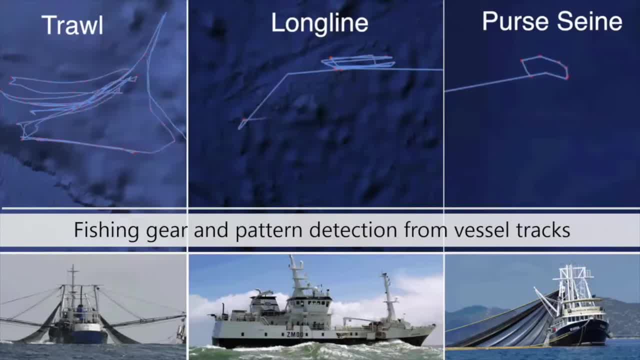 and then retrieve it, so these back and forth patterns develop, compared to purse seiners, who set a net around the trawling fish, such as a mackerel, for example, or a smaller tuna, where these looping patterns develop And then the vessel stays attached to the net. 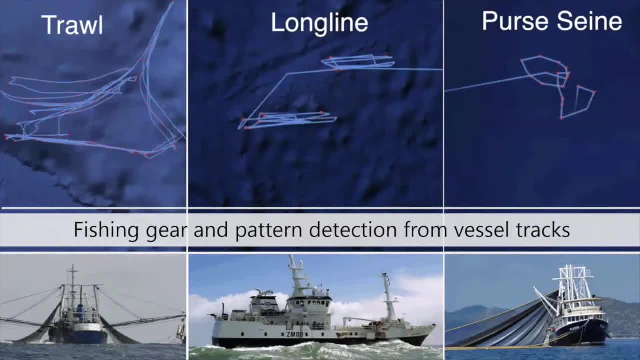 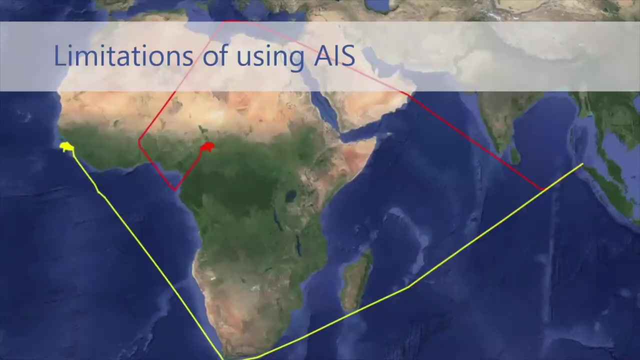 to scoop out the fish. So by training a neural net to automatically classify these patterns, we can now detect fishing effort and classified as seen from the AIS data. Before I dive into some of these studies and data, I would like to highlight some limitations of using AIS. 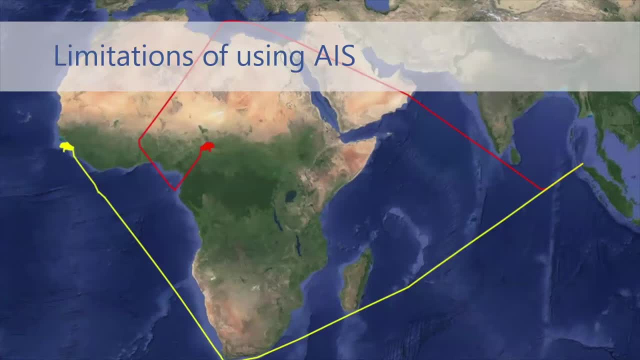 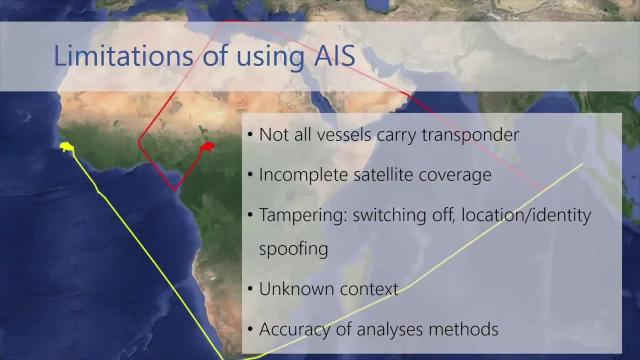 because I think this is important for the wider understanding- what is possible with it. And, firstly, it is very important to know that not all vessels carry AIS, So this is different to the often government-mandated VMS, the Vessel Monitoring System, which is a closed system. 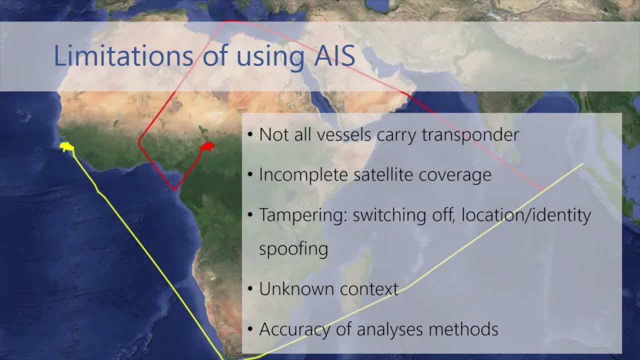 that governments usually use. It's very hard to access this data, with exception of some countries who have chosen, in the name of transparency, to share it. And yeah, we don't really know the exact amount of vessels that carry AIS, because the exact amount of vessels 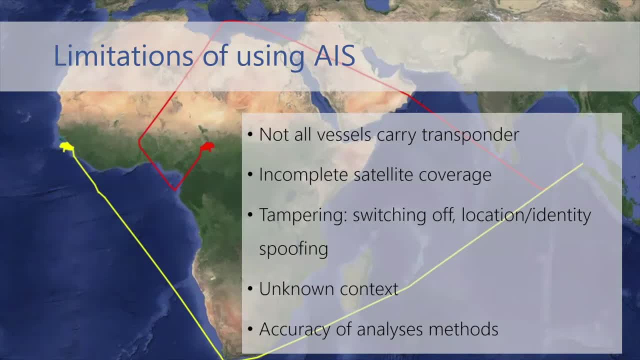 itself is unknown. So we have a rough estimate, which of course varies by size, class. Not so much a problem anymore is the incomplete satellite coverage which has caused some gaps in the data in the past, but it's continuously improving. 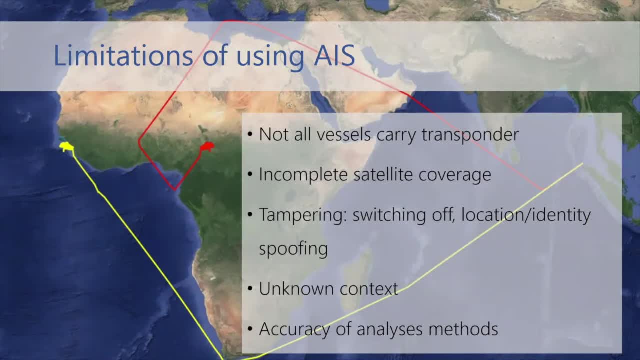 So that is a very good development, But then also something that is of importance to know is that AIS actually can and is tampered with, So the device itself- they can be switched off, or the location or the identity can be spoofed, so falsified. 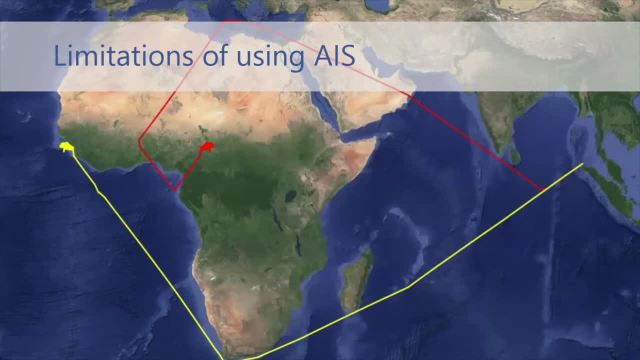 And an example is shown right here. So the track we got from the AIS data was the red one, which looked rather suspicious. So with a bit of fiddling we discovered how they manipulated and flipped the coordinates to get the yellow track, which was the actual AIS data. 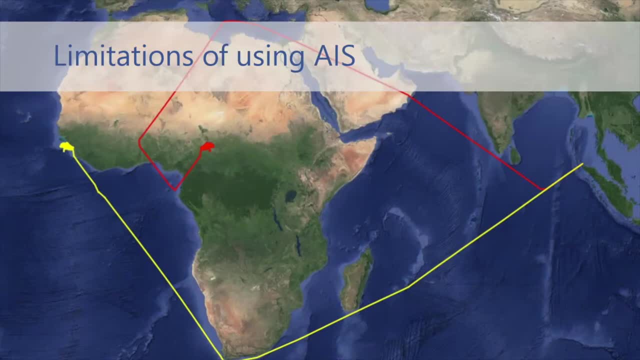 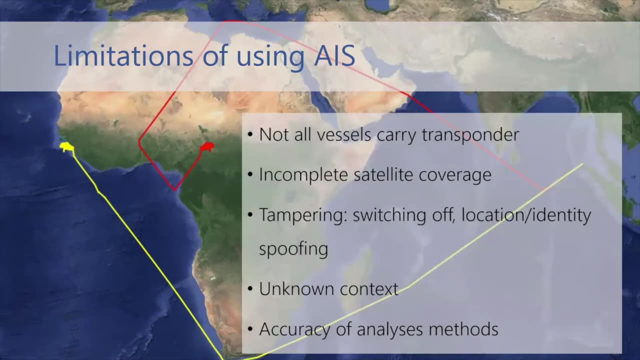 And then we found out that it was the actual track of the vessel which turned out to have a questionable license to fish in that area. So that, I think, also highlights the importance of knowing the context, And AIS data really is best enjoyed with some other data. 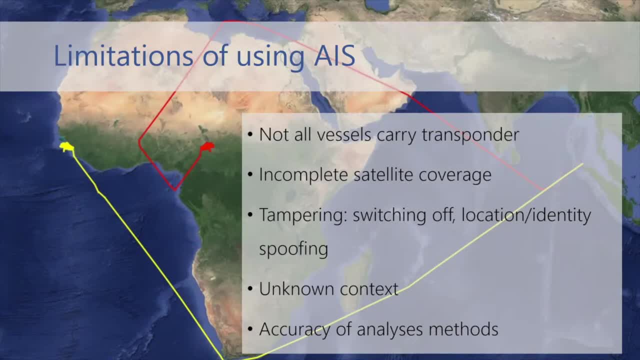 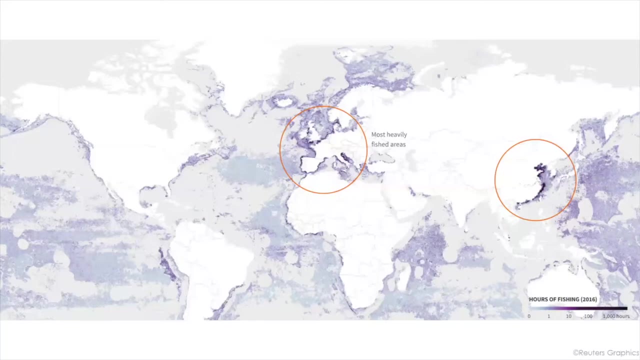 and some context and background knowledge. And of course one has to pay attention to the accuracy of the method of analysis, So to show you what can be done with it, especially in the context of conservation and active management. this is the same data as the map I showed you before. 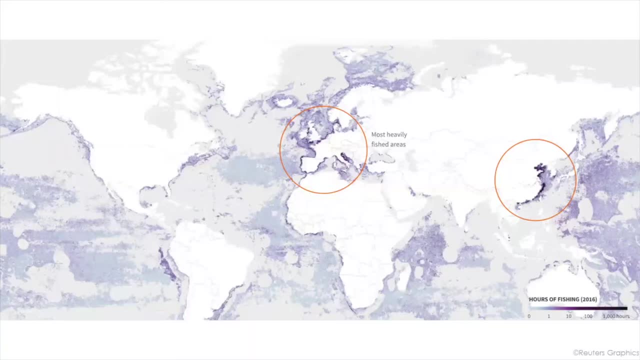 And here we can really see the intensity of fishing and the two biggest fishing hotspots, which are, unsurprisingly, around Europe and China. And with that spread we can also see areas where we either. A don't have data. 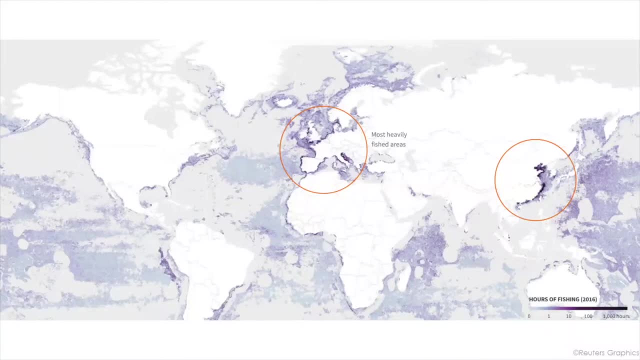 So, for example, the Caribbean and Southeast Asia are big fishers. There are big data gaps, but also then some real gaps. If you look into the Pacific, around the Pacific Islands, these are the exclusive economic zones that seem to be working pretty well. regarding 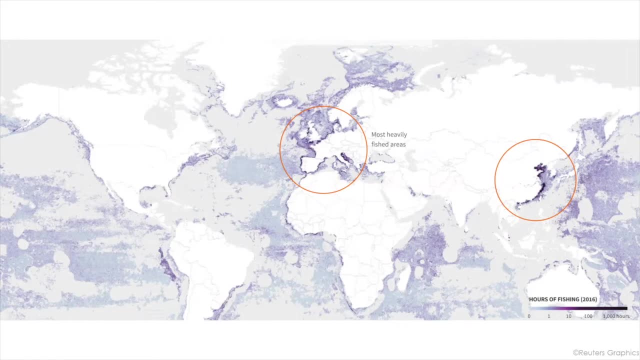 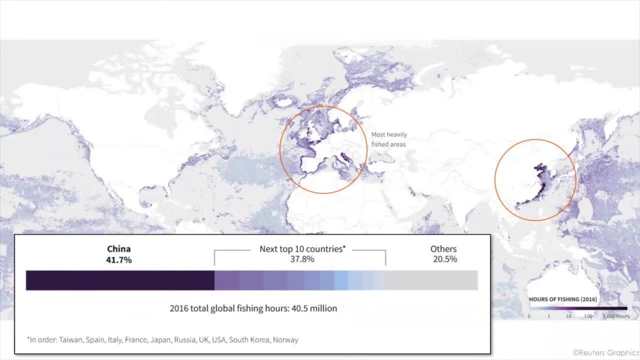 their management, And because we also know the identity and types of the vessels we are observing, we can also see which players are out there, And this was something that personally floored me when we got that result, despite somewhat knowing it, but not the dimensions and extent. 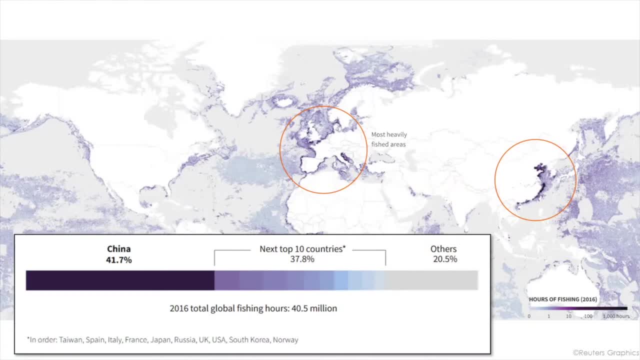 is the amount of fishing China has ramped up in 2016.. So nearly 42% of the fishing effort we observed that year was done by Chinese flag vessels, which is more than the top 10 next fishing countries combined. So, when talking about management and conservation, 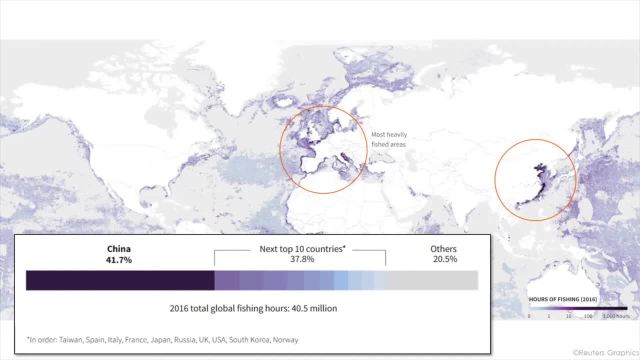 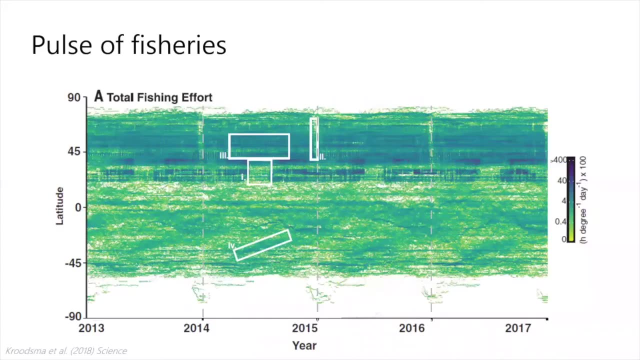 this is really giving a picture of which players and which stakeholders need to be at the table regarding these conversations. And then also, we were very interested to know what is the pulse of fisheries, What makes the fisheries tick as they do? And this really came out of the thought. 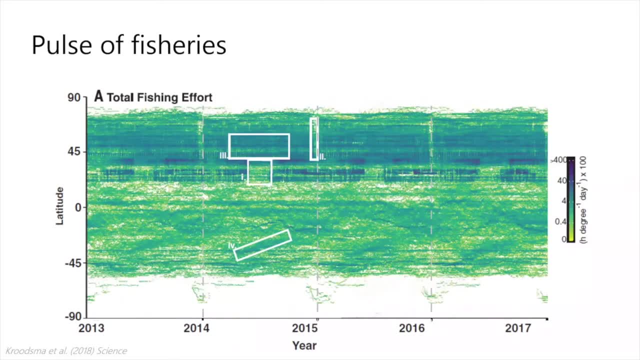 that humans are natural predators And, like other predators, we're driven by natural cycles, for example. But we had a long good look and looked again and again and we could not really find much, So instead we came up with this, which 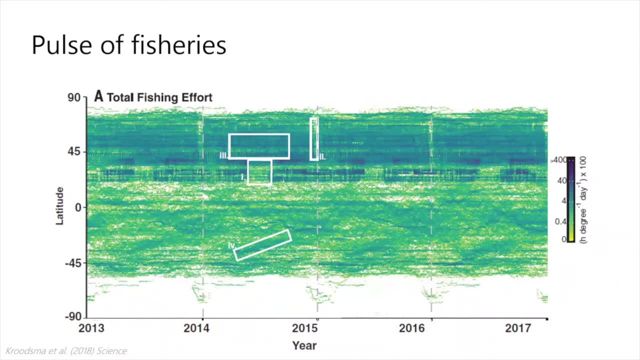 is a bit of an unusual depiction. So to walk you through, on the y-axis you see latitude And on the x-axis you see time. So you basically imagine it. You need to imagine to look down on latitude by time. 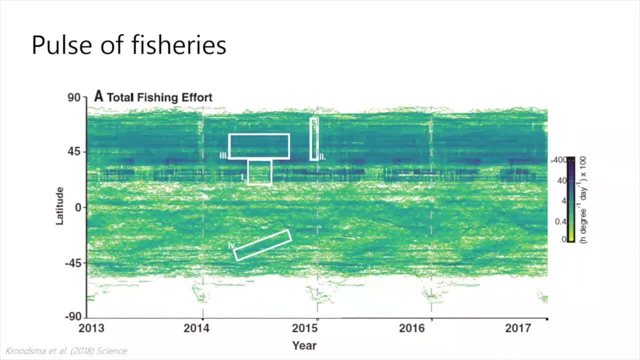 And depicted from yellow, light greenish to dark blue is fishing intensity, And when we plotted this, we at first thought we had some artifacts in the data, but they were too regular. So especially the big gap here in the middle of each year. 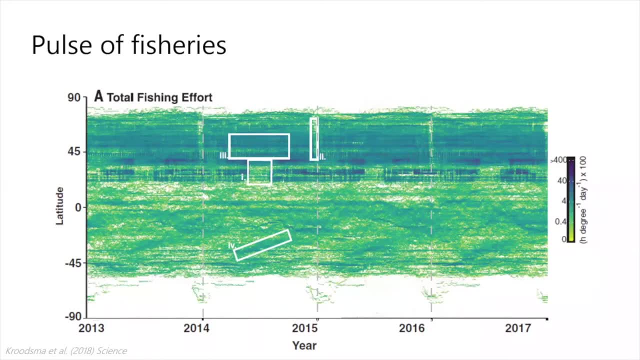 noted with Roman number 1, which, upon close inspection, turned out to be the Chinese fishing moratorium. So every year, So every year, in the middle of the northern summer, China calls back its boats, And because the fleets are so massive, this shows up in the global data. 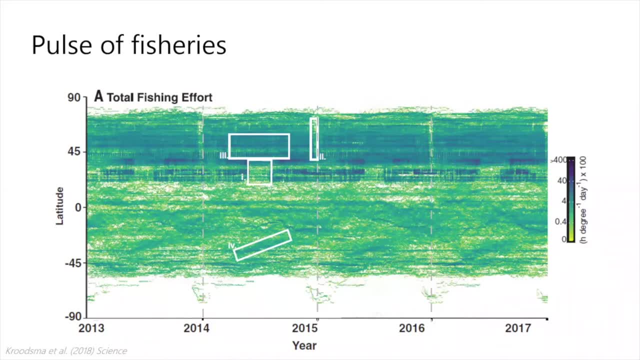 Then, even looking further north, we also saw some patterns, mainly around the end of the year, And this indeed has turned out to be Christmas and New Year's, because fishermen like to be home with their families during that time, So fishing effort is less during that time. 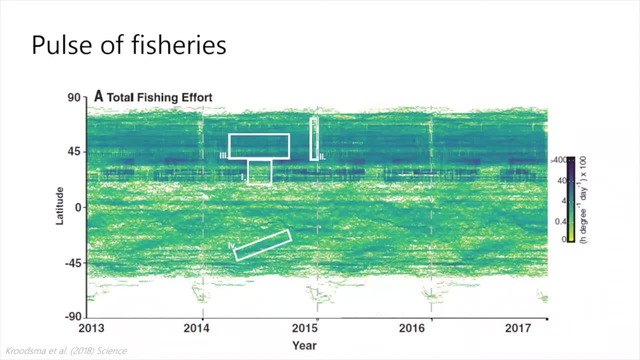 And if you squint a bit, you can see a fine pattern like this, like around the same latitude, which turned out to be the weekends. So a similar thing: fishermen like to be home with their families for the weekends. So the only pattern we really found. 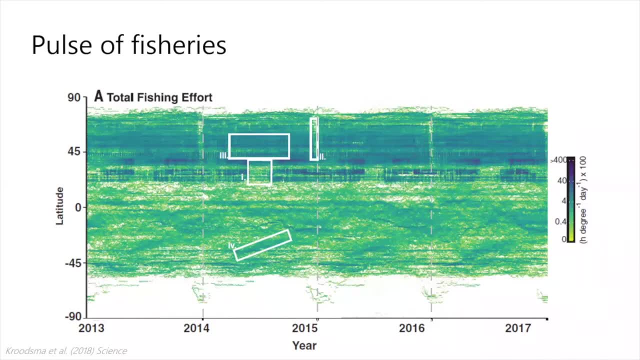 that correlates to natural cycles is denoted by number 4 here, which is the Indian Ocean tuna fleet moving up and down with monsoon times. So this really highlights that we are the technology, and the rapid evolution of technology, of course, has removed us a step from these natural cycles. 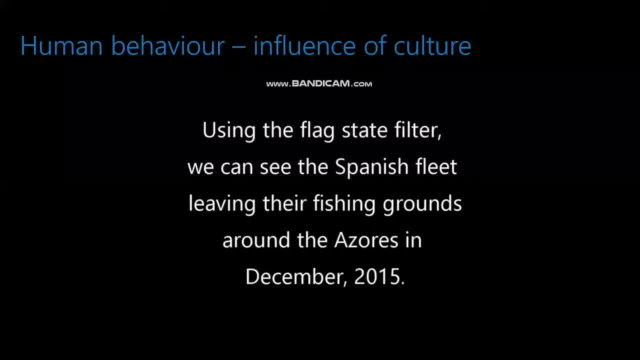 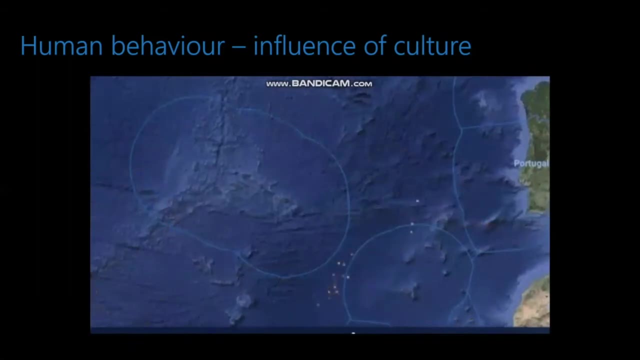 We are really cultural predators now. So the influence of culture is also nicely illustrated if you look at the actual tracks- And I hope this video plays. So this here- what you can see, the little lights are fishing efforts. So this is one of the first versions of the Global Fishing. 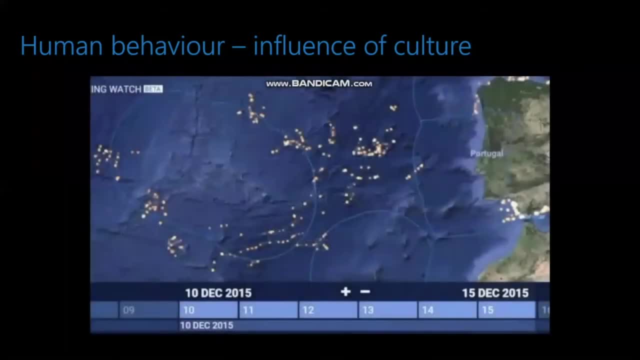 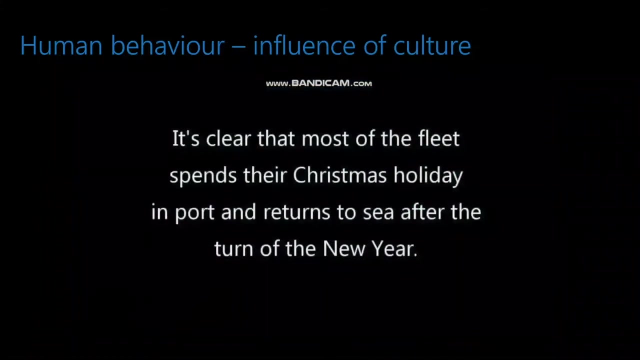 Watch Map And showing around the Azores for some vessels. So you see a time slider. This is approaching Christmas. Vessels are going back to Spain and Portugal And then in the new year they are coming back. So this just highlights basically on the water. 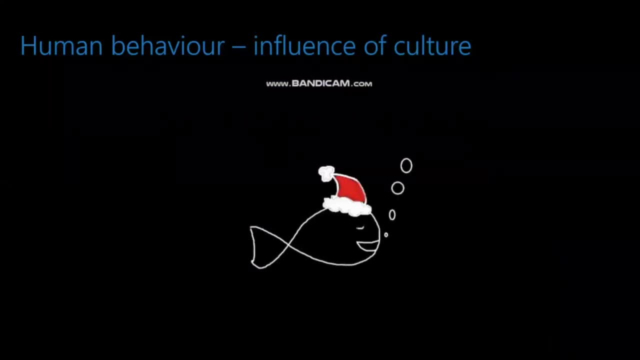 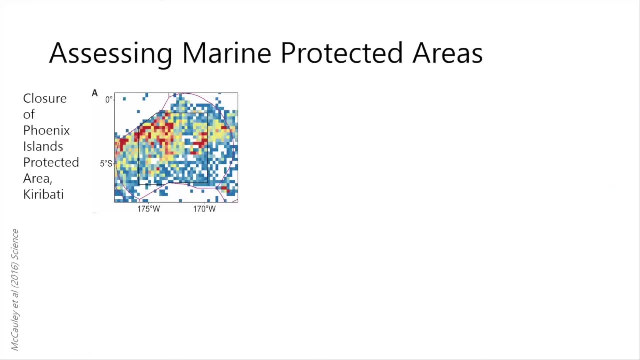 what you could see in the graph before that, And we can also use this data to assess marine protected areas. So The first example I would like to use here is coming from the Phoenix Islands protected area in Kiribati, in the Pacific, which 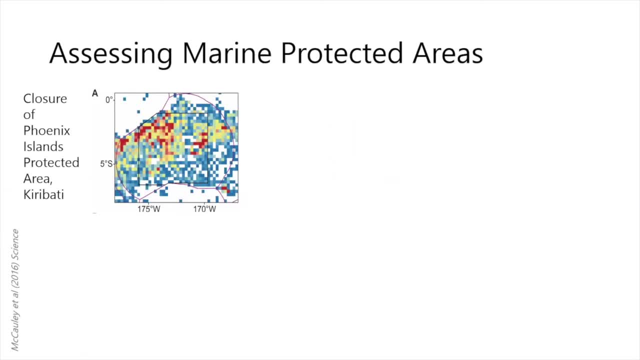 area was closed at the beginning of 2015.. So it had been a protected area before, but had significant fishing effort inside which was licensed, But then it was turned into a no-take area And this is what we saw three months before and three months. 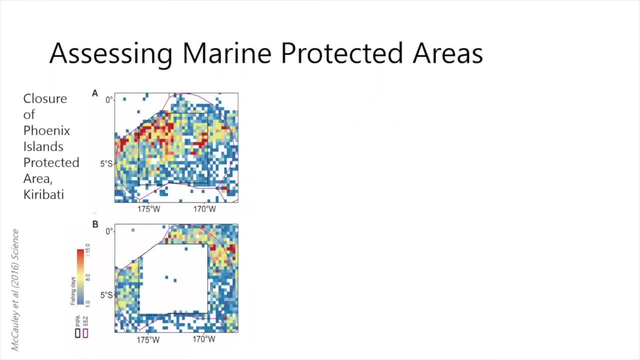 afterwards. So really, This gives us a big, big scale observation and window into seeing the movements of these vessels and also where they went after that And, as often said, the vessels are being displaced. We could not find that following some of these vessels. 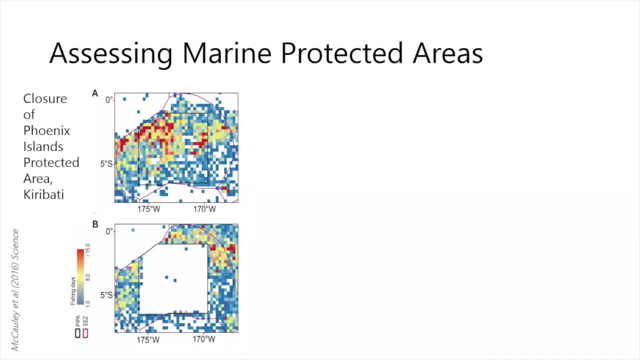 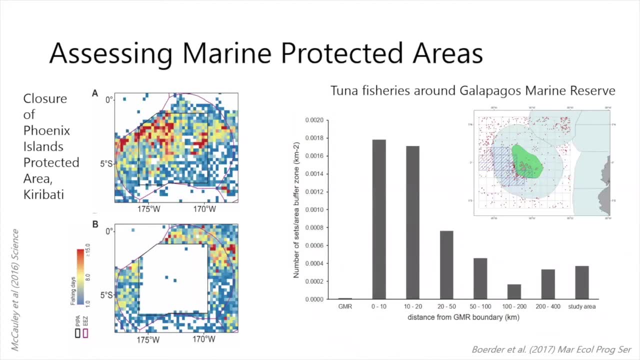 They've dispersed pretty widely following the closure of this protected area. And then we can also learn more about how vessels and how fisheries are really reacting to marine protection. And this is a study we did around the Galapagos Marine Reserve, which is the green avocado shaped. 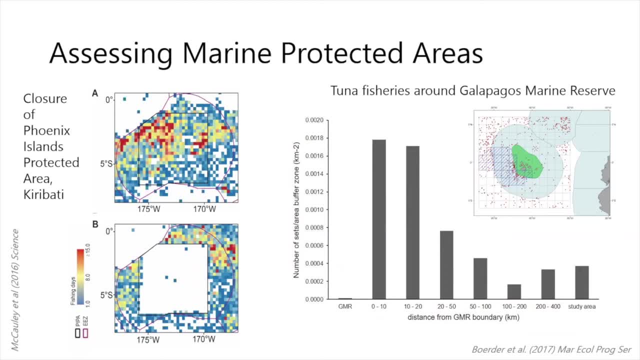 form in the little map And each red dot you can see is a set, a purse zaner set for tuna fisheries, And the grid denotes the study area And by looking at where these sets were, we found that about four times as many sets. 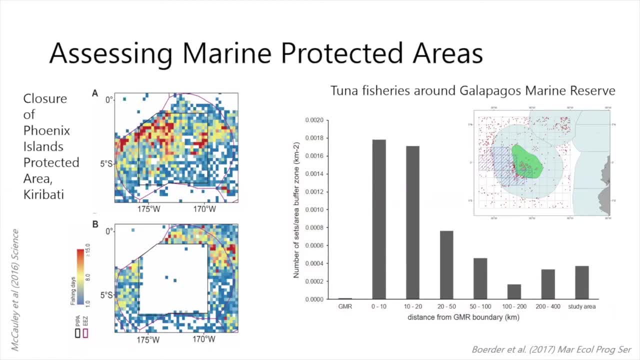 were set within 20 kilometers from the boundary of the Galapagos Marine Reserve compared to the whole study area, And that is mainly in what we call the hotspot to the southwest of the reserve, which is also a really good fishing ground, of course. 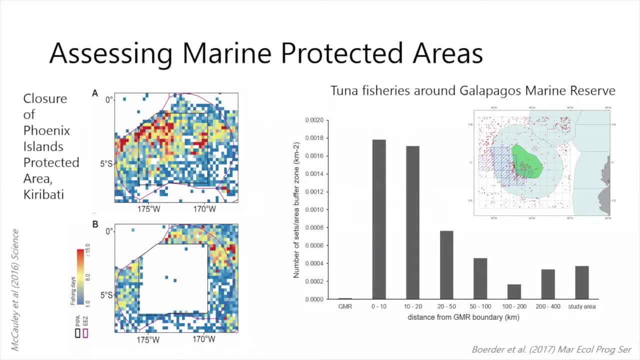 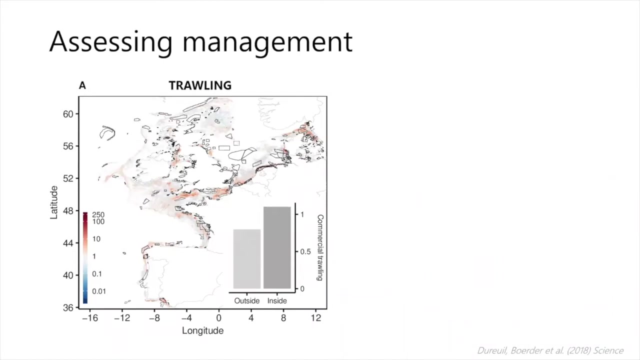 And this kind of data really comes in handy. I don't know if you have heard about plans to expand the Galapagos Marine Reserve and currently figure into design and zoning plans for something like this. And then also an important thing to highlight is that- and I guess that also loops back- 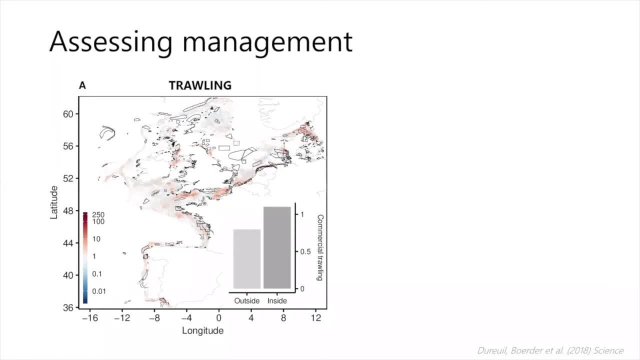 to talking about not only quantity of protected areas, but also quality- that this type of data- because it affords us a big picture, look- enables us to assess management. This is a study we published in 2018, looking at fisheries in European waters shallower than 800. 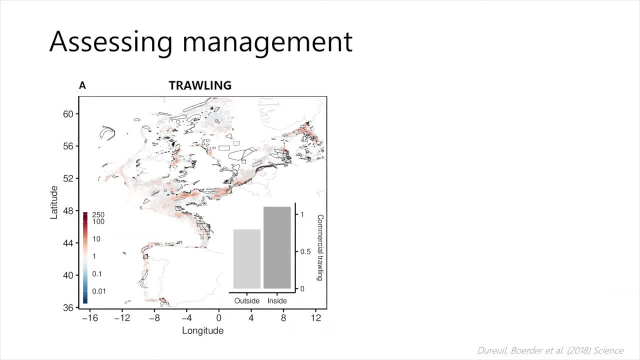 meters, I'd like to note, and the connection to the network of marine protected areas in Europe. So this is over 700 protected areas we included in the study And we found that an average trawling effort in these waters is 1.4 times higher inside marine protected areas. 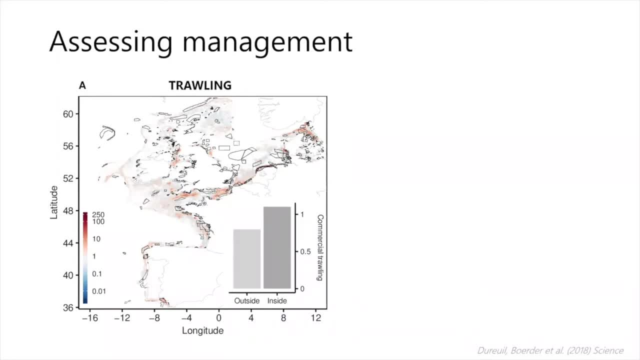 than outside. I would like to note that this is not illegal fishing. It's simply a result of the European Union's policy to manage fisheries separately under separate piece of legislation, And we found that this is a very significant step in managing fisheries in Europe compared to nature conservation. 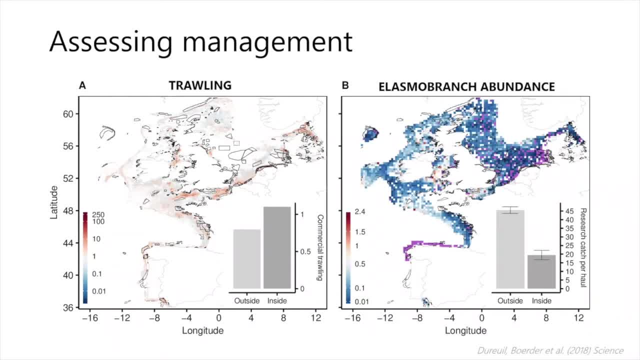 So we compared this to abundance of Europe's most vulnerable groups of species, which are alesmobranchs, so included I think it was 20 different species- and analyzed data from research catches by Hall and found that these alesmobranchs were, on average, 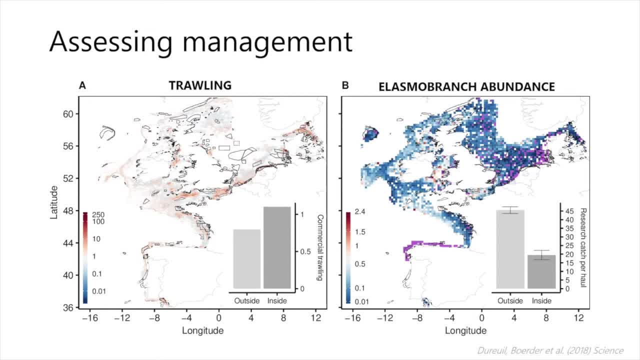 more protected areas than inside, especially the most endangered ones, up to five times more common outside. So, with regards to managing protected areas, I'd like to note that none of these protected areas has been specifically designed for alesmobranchs. 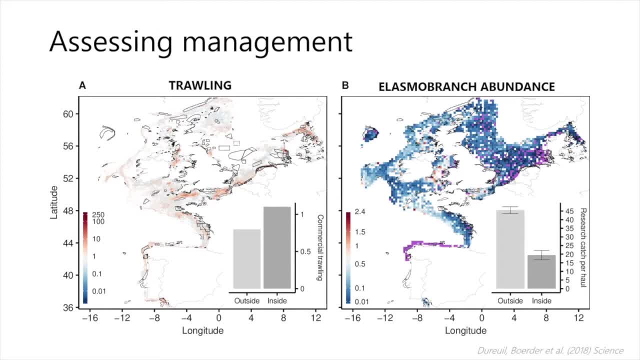 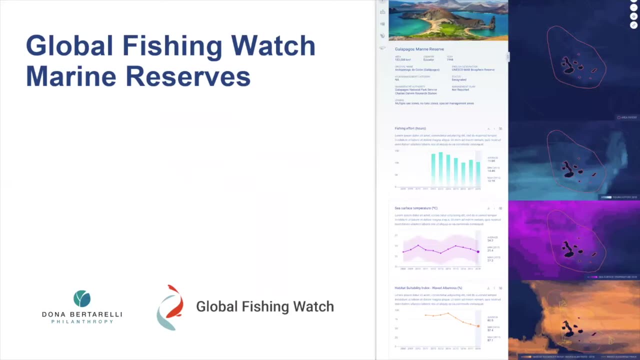 but they represent one of the most vulnerable groups, So the current management seems to be failing this group. So, to change track a bit From the future to the present, to what we can done, and look ahead, I'd like to stress again that we do have the understanding and data. 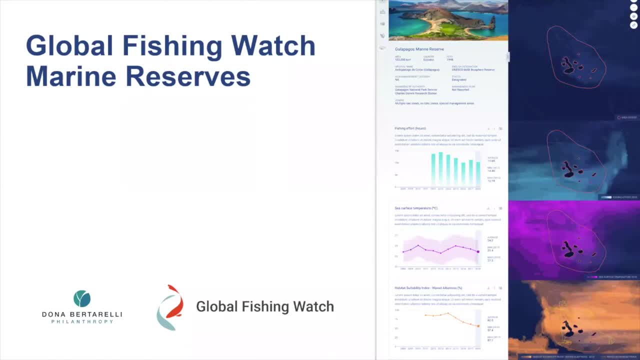 necessary for robust protection and management of biodiversity. We just need to make it happen. We need to especially move from reactive approaches to proactive approaches, However. management, indeed, is often hampered by inadequate information to support decision making. So decisions are being made, but they are often not. 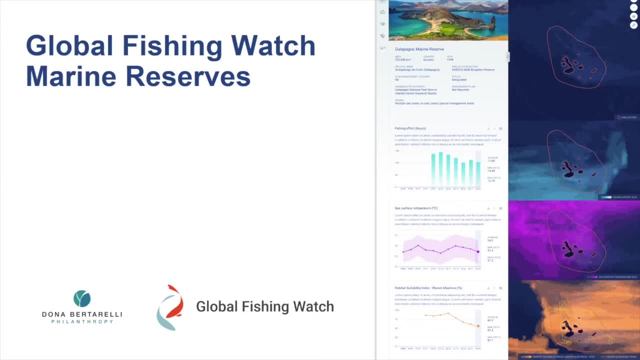 using the best data available, because this data often is inaccessible or not used in the right kind of ways, And this failure really to get the data from those who produce it to those who use it and then implement it leads to lost opportunities to inform management decisions. 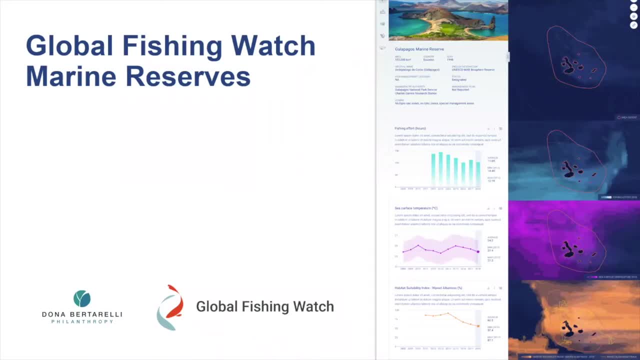 So I'm very, very pleased to be talking about a new project I'm working on in collaboration with Global Fishing Watch, which is a new tool called Global Fishing Watch Marine Reserves that we're going to launch for first looks in May this year. 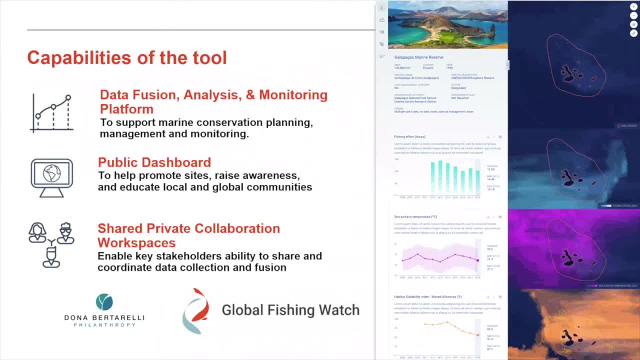 And what it is. it's a free online tool that is a data fusion, analysis and monitoring platform. So, similar to Global Fishing Watch, which we'll be closely coupled to, it's a tool that aims to specifically support marine conservation: planning, management and monitoring. 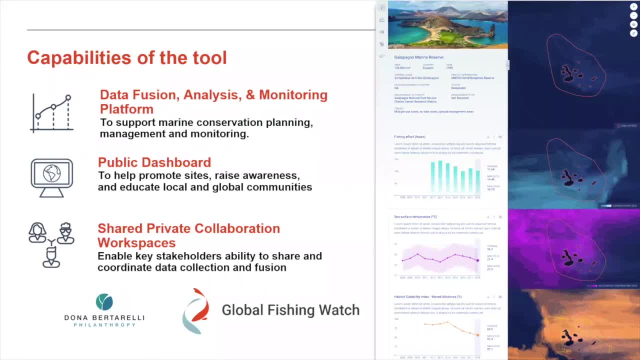 So we are targeting as target audience marine managers, marine plans, spatial planners and, of course, scientists working alongside these topics. There is a public dashboard that everybody can access for free to help promote the sites we're working with, to raise awareness and educate, of course. 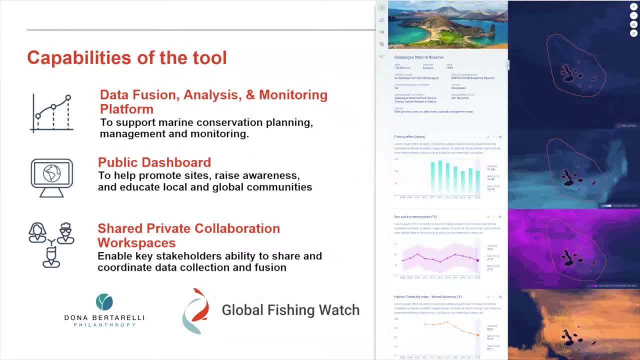 And then there's a range of, or there's the possibility to create private collaboration workspaces that can be shared with teams to really enable dedicated work using the data sets included in the platform But also upload, for example, data that cannot be shared publicly but within the wider team. 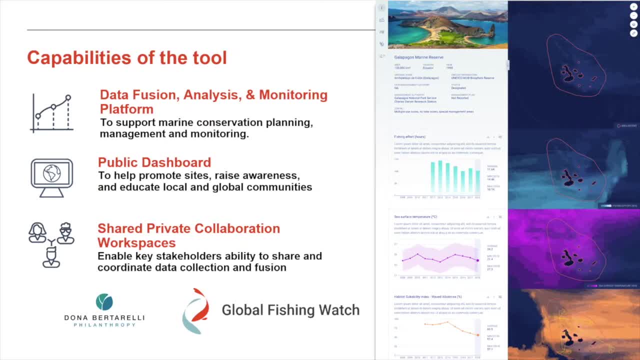 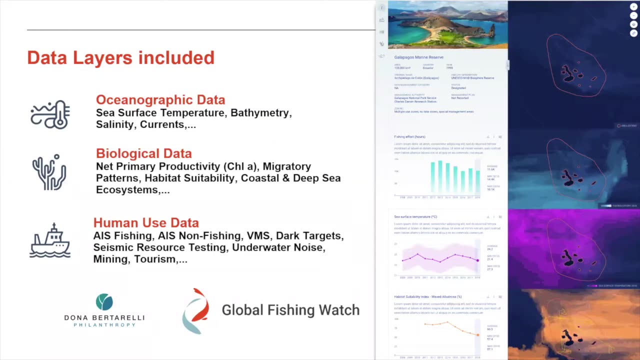 to foster collaborations across countries and institutes and organizations and provide standardized data for these approaches, So, data layers included, really can be divided into the three big buckets, And some tools are already out there that are approaching this, but we're taking this, Thank you. 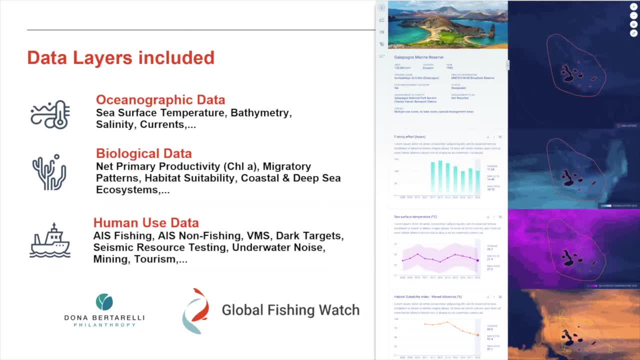 Of course, we are providing the oceanographic data, such as sea surface temperature, bathymetry, salinity and currents, And anyone of you who has ever worked with this type of data might relate to how overwhelming it can be to find the right data set, to access it and also to just like really. 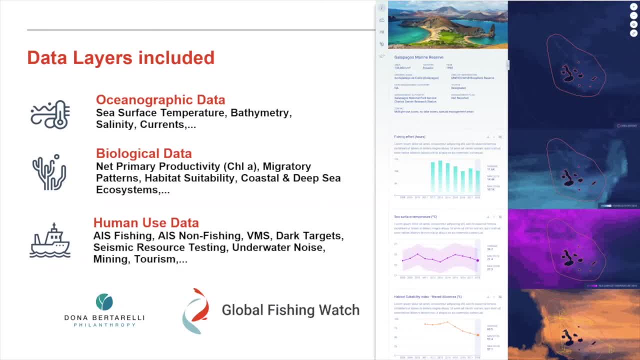 unpack it from file formats I personally had never heard of before starting to work with this type of data. The next step, then, is to really link it, to link the physical properties to the biological. so we're bringing in, of course, chlorophyll like primary. 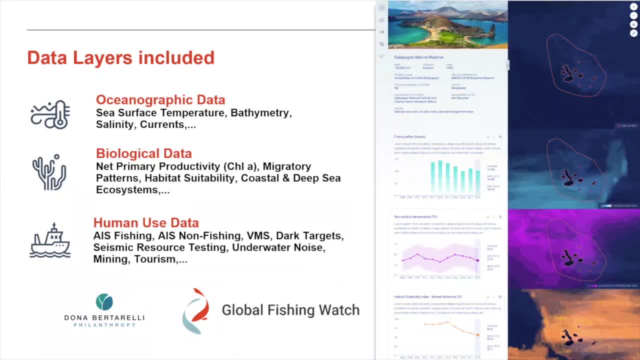 productivity data, but then also go a step further in collaboration with the myco project to bring in data on migratory patterns and migratory connectivity, and then in collaboration with actually the very own gabriel raygondo here on habitat suitability and also, of course, on data. 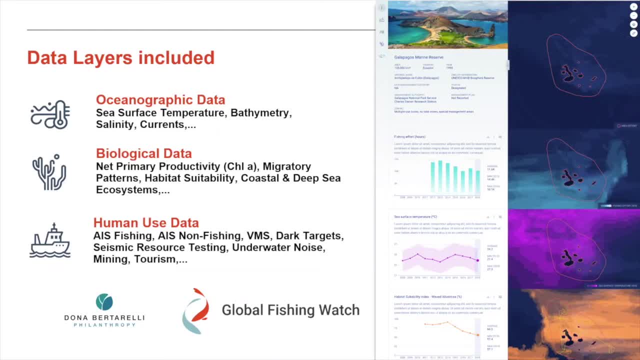 on coastal and deep sea ecosystems and then lastly- and this is the real step where we see the value of this tool- link this to human use data. so the obvious, of course, is the fishing ais data, but then we have a whole big data set on non-fishing vessels. so any shipping and its 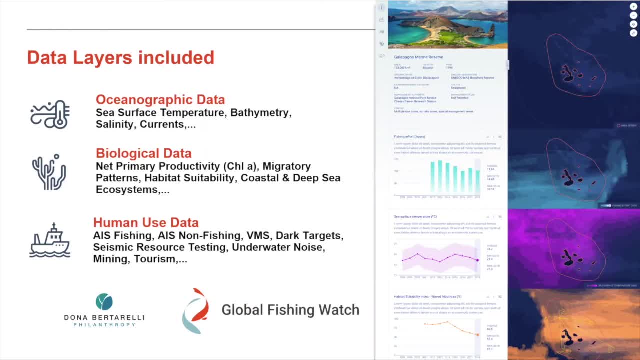 impacts and data sets on vessels that are not appearing on ais. so the vms that gets shared with global fishing watch, dark targets that do not have any transponder and then, of course, the impacts these vessels have. so currently, in collaboration with jasco, we are producing the first global underwater noise map, and this will include of: 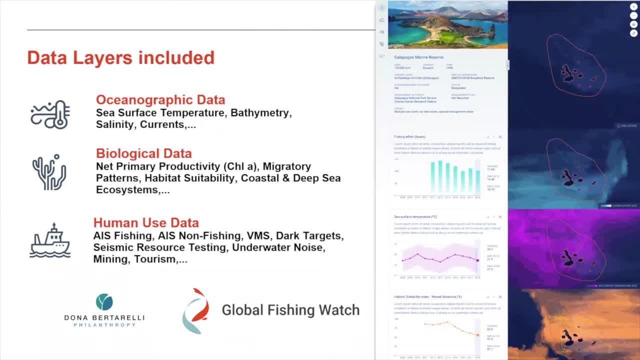 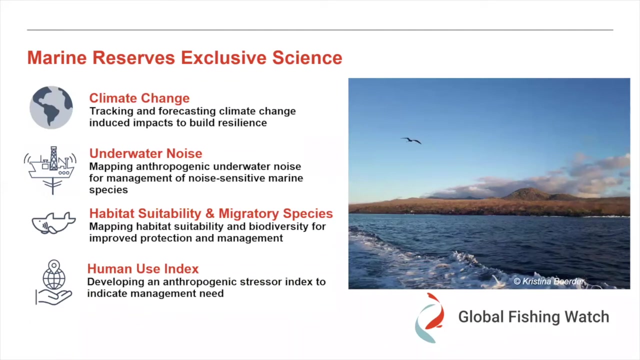 course, a specific information on things that such as seismic testing for for resource extraction and, going beyond the noise, other data sets on human uses such as mining, tourism and anything else that is of interest, and these data really, of course, feed, hopefully, into the work marine managers do and scientists do and to further certain types of work we will have. we have four. 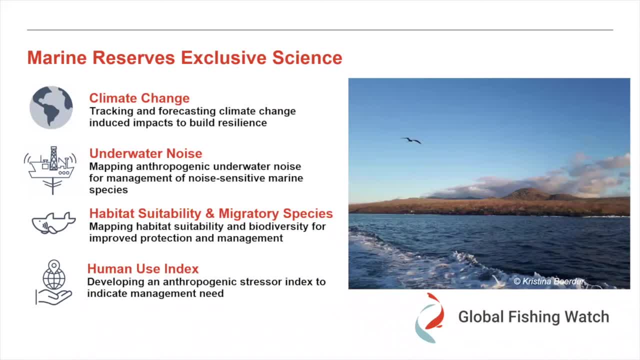 big projects that are signs, that are supporting or generating data for this, for global fishing watch, marine reserve and climate change is one of the biggest ones, of course. so we're currently working on a project to track and forecast climate change in these data sets to see their induced impacts. 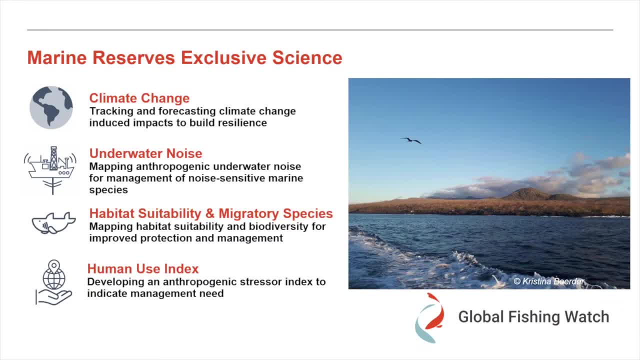 and to help build resilience, for example, by better understanding how climate change data can be incorporated into mpa management. i mentioned the underwater noise that we map the anthropogenic underwater noise, especially for management around noise sensitive species, and i think this is something that is very familiar for anyone on the west coast regarding the work around, for example, the 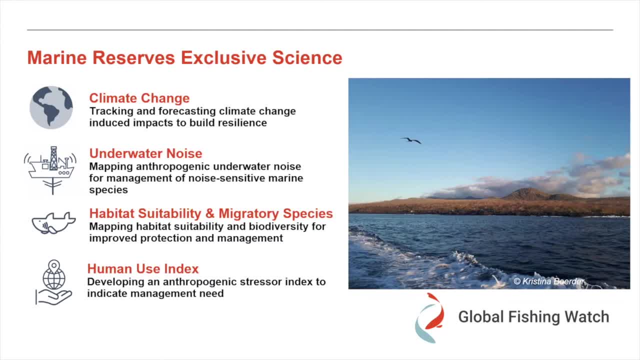 example of the uvc in the south coast, and then, as i just mentioned, in close collaboration with michael and then with with gabriel and william chang's group at uvc, we're looking at migratory species and habitat suitability and how this links to the protected area networks and the spread of. 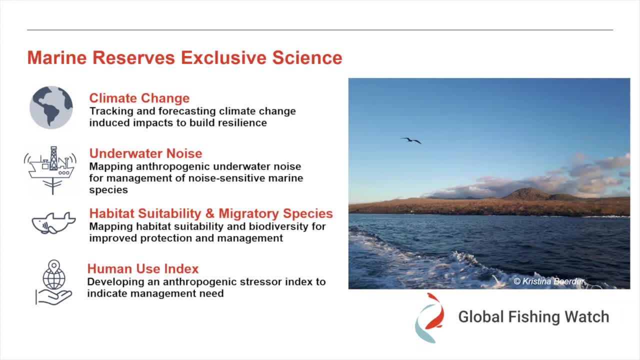 networks across biodiversity gradients, for example, and how it can be figured into management, even looking into how these kind of data sets can be made dynamic to interact with this dynamic map and then even with respect to forecasting this into the future and the climate change And, lastly, to make the human use. 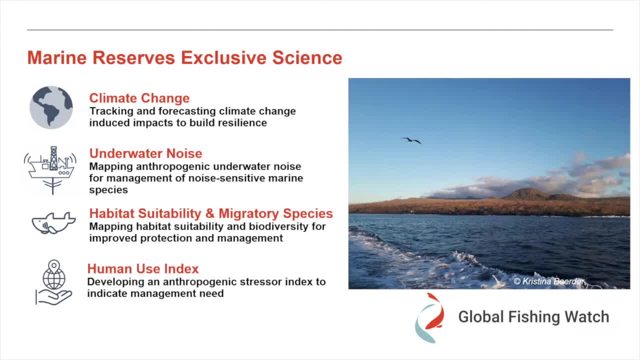 really more tangible for planners and managers. we're developing a human use index that is dynamic. So a lot of you will probably be familiar with the work of Halpern et al regarding the cumulative human impact maps. So, along these lines, but under using really a dynamic, up-to-date data, 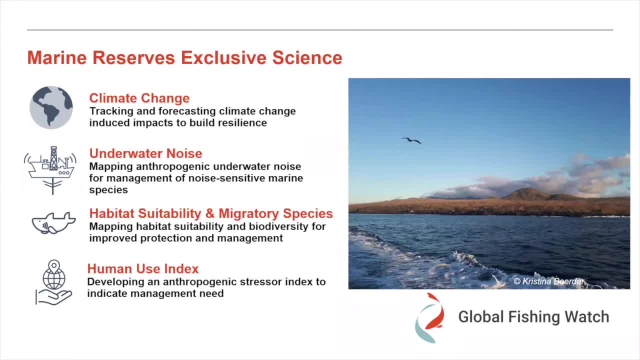 that enables managers to monitor and adjust and react to human stressors in their areas of interest. So just to give you a quick look into what the tool looks like- and I would have loved to do a live demo, but I don't trust the internet- 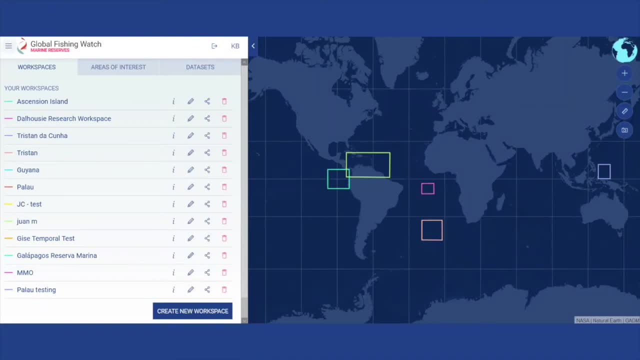 I don't trust the internet enough for that, So I'm showing you some screenshots. So we currently work at five pilot sites that we're expanding this year, which is Galapagos, Guyana, Tristan, Acuna, Ascension and Palau. 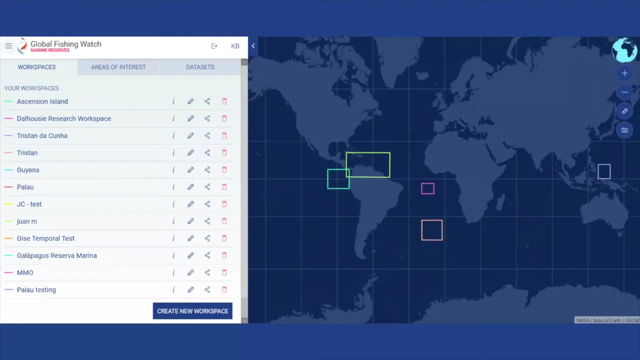 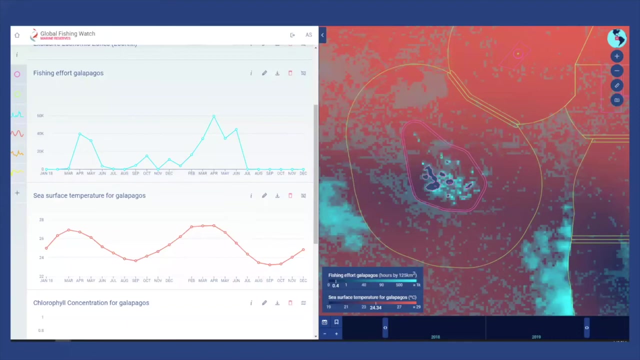 And this is an example here of the workspaces that can be created that can be also shared within teams, and users are able to either click predefined areas or upload or draw areas of interest, And within this, then data sets can be either uploaded or selected for use. 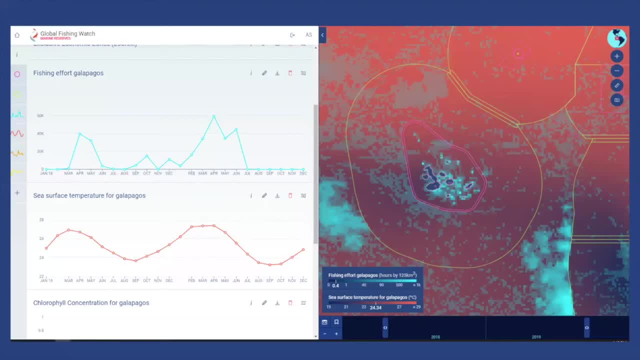 And I've shown here fishing effort in blue and sea surface temperature for the Galapagos Marine Reserve and depicted in pink and the exclusive economic zone in greenish And you can see at the bottom there's a- I don't know if you can see my mouse. 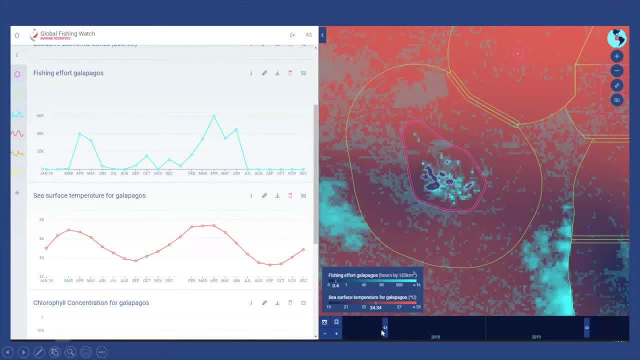 at the bottom there's a time slider So the user has the option to really select the time of interest. It's like a time slider so you can select the area of interest And then, when you mouse over, the values will be shown. 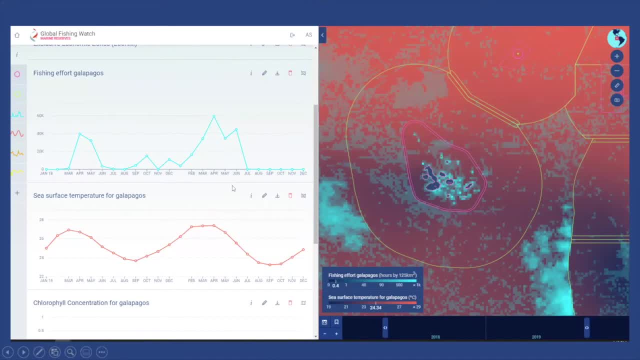 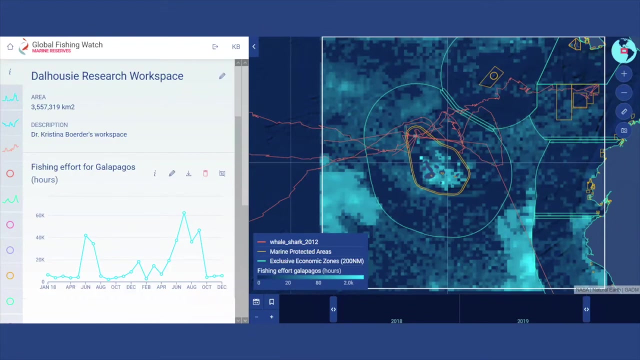 and graphs will be created to give you a quick overview of the development of the respective parameters in the area of interest And that can then be connected to data that can be uploaded into your private workspaces. Here, for example, that might be sensitive data. 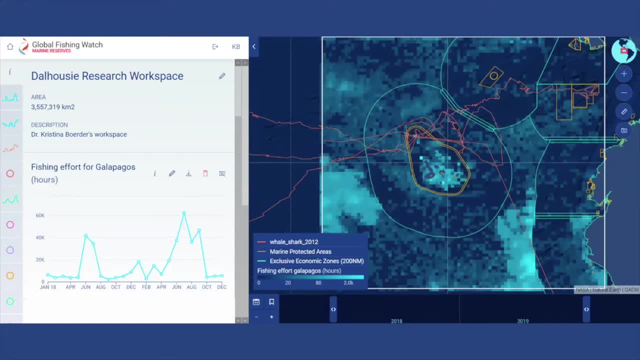 such as whale shark tracks, as shown here in orange- And you can see that the data that we're looking at is from the Galapagos Marine Reserve. And then we used to look at the area use of these species, for example, here shown in blue. 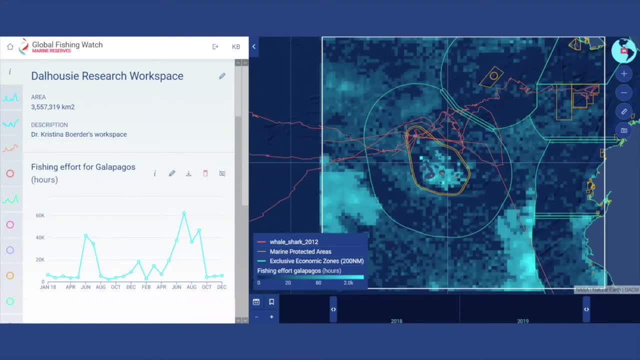 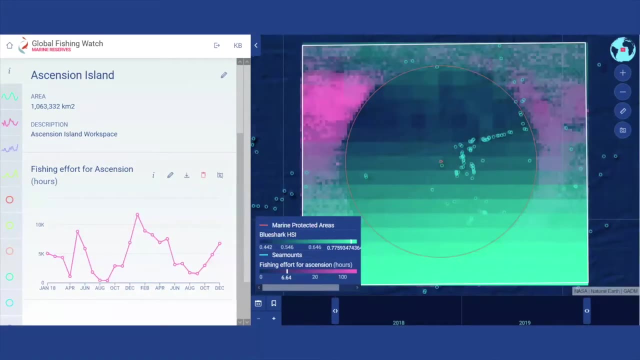 compared to fishing effort over time. And these data sets then also can be downloaded, because they were standardized to the same resolution, and then ideally be used offline in further analysis. To give another example, for example, for the Galapagos Marine Reserve, for example. 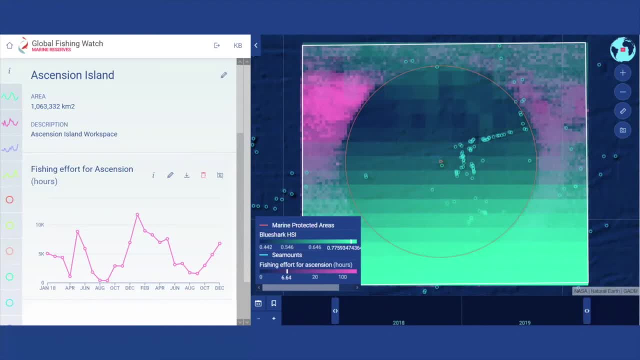 for Ascension Island. So this is the marine protected area in Ascension, and Ascension being this tiny dot at the middle of the circle And the other circles around it depict locations of seamounts And, in green, the Habitat Suitability Index. 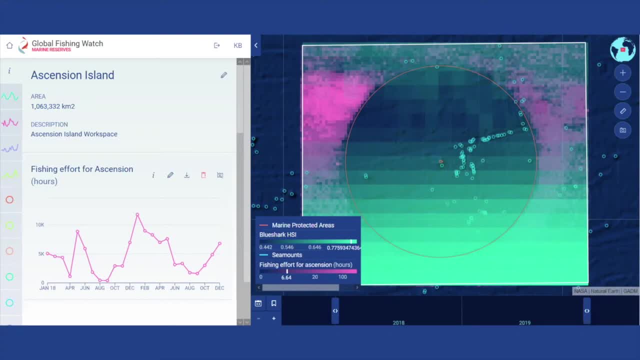 for blue sharks that Gabriel and his colleagues have developed And in pink, the fishing effort around Ascension Island. So again, this can be used for very direct management questions to monitor- not only how over time, of course- how the habitat suitability might change. 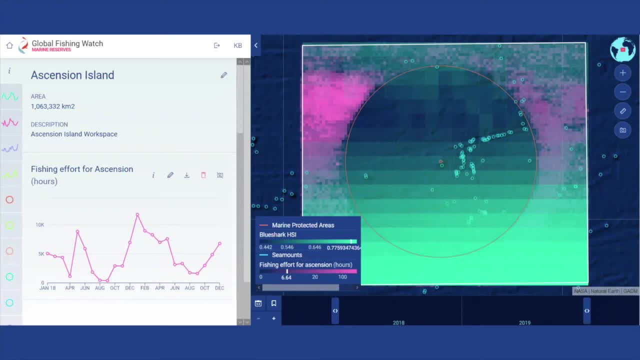 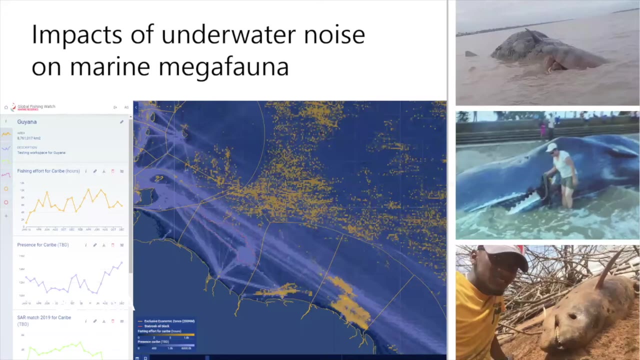 but also how the use, the human use and stresses in this suitable, potentially suitable habitat are developing over time. And to conclude, I'd like to walk you through two examples that we are currently working on. So one is the impacts of underwater noise. 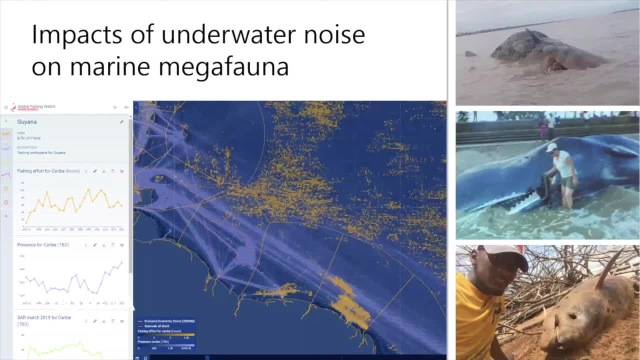 on marine megafauna. This is a collaboration with Guyana, where we are working on a new oil field that has been developed over the last years. It's a bit hard to see in the map. It's depicted in orange right here. 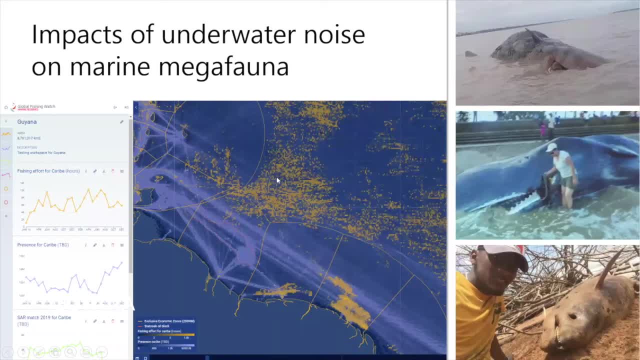 And in this lighter yellow is the fishing effort for the wider Caribbean And in purple the general vessel traffic as seen from AIS. And Guyana and Trinidad and surrounding countries have noticed a reduction of very recent increase of cetacean strandings, especially sperm whales. 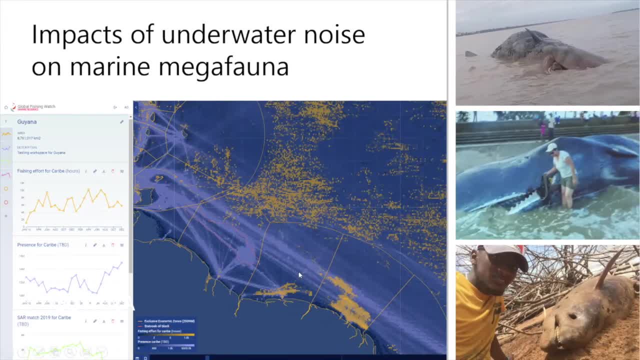 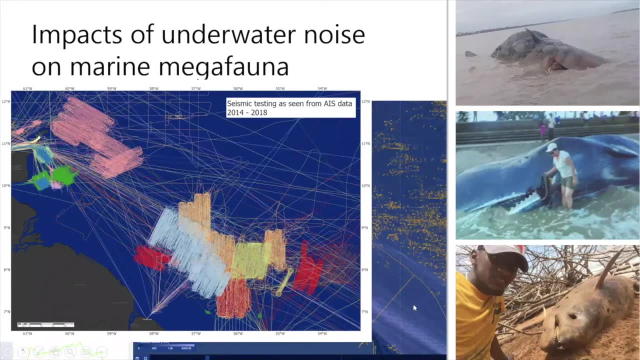 which had not been recorded before to that extent. So they're really interested to see how increased vessel traffic and underwater noise might contribute to that. And just to give you an impression, this is a very hectic map. Hectic because this is seismic testing vessels. 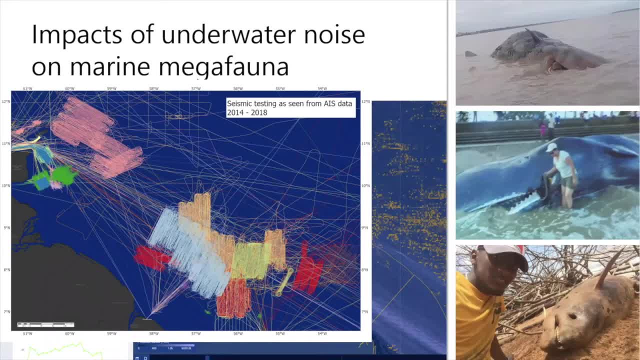 that have been active in the area between 2014 and 2018.. And all these back and forth, very regular patterns are seismic testing patterns And this, of course, makes for an incredibly noisy environment while these testings are going on. And similarly along these lines, 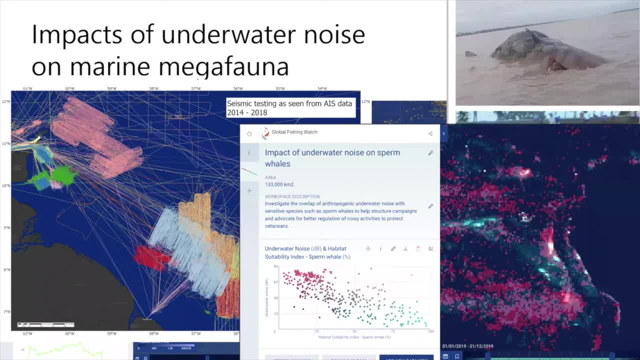 this is partly fake data I'd like to mention to test this type of analysis. We are aiming to create maps and images and knowledge around the soundscape species might be experiencing over their suitable habitat range, In this case for the Eastern Tropical Pacific, for sperm whales. 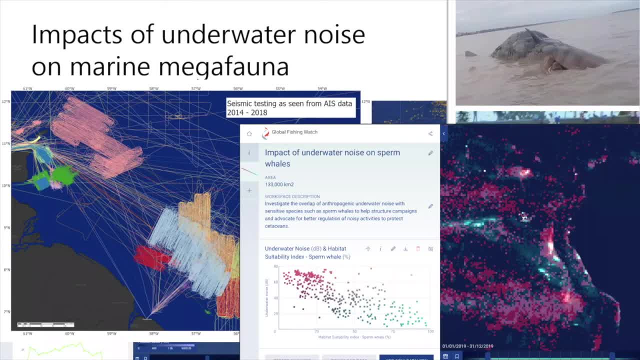 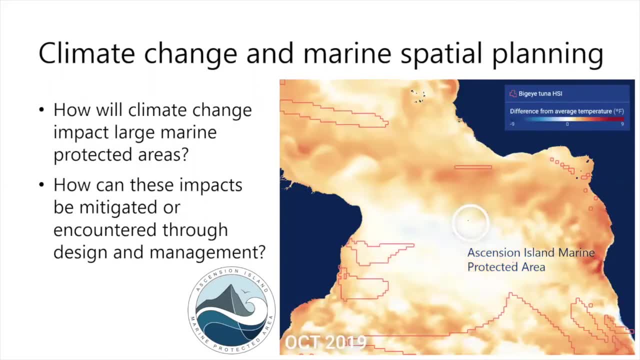 underwater noise versus their habitat suitability index. And lastly, to loop it back to the climate change topic and the marine spatial planning, this is Ascension Island again, And their managers, their managing team, is very interested in better understanding the role Ascension Island has. 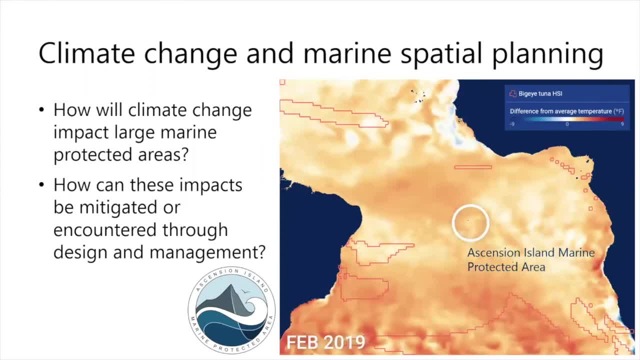 For ocean basin wide management of species of interest- mainly also migratory species of course- and the role the marine protected area plays in that. So in red you can see the habitat suitability for big eye tuna outlined And then the sea surface temperature. 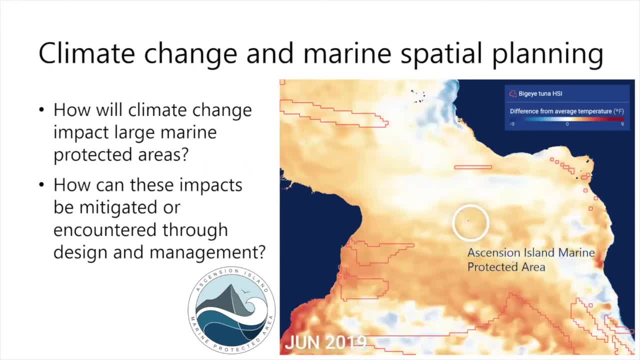 anomalies for the year 2019. moving through this, So really highlighting that in order to make the best use of this data, we need to have dynamic- ideally need to be having dynamic- data and to answer questions on how climate change will impact large marine protected areas. 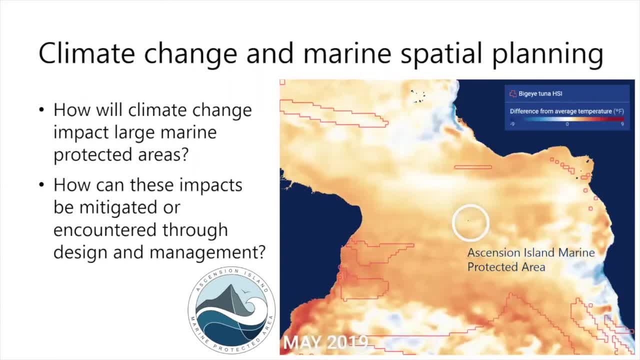 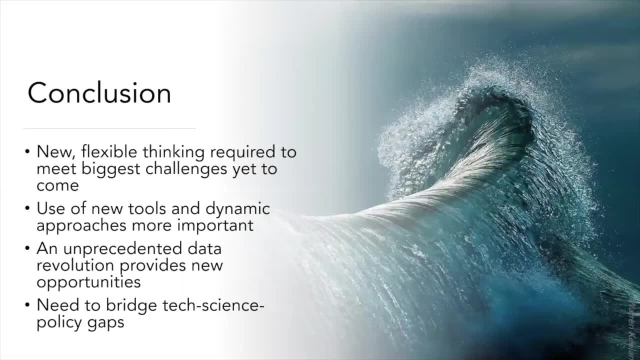 such as Ascension, and how these impacts can be mitigated or encountered, especially through design. and then, of course, the management going ahead. And with that I'd like to conclude that we're in this age of rapid change, but this rapid change, 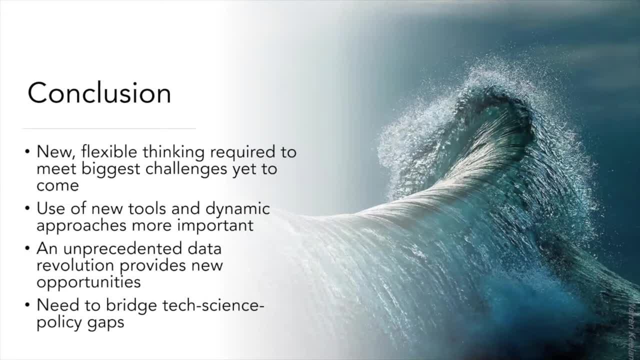 really requires and stimulates a new, flexible way of thinking, because the biggest challenges are rolling right our way, But we are not facing that completely unprepared. We have a range of new tools and dynamic approaches that are becoming increasingly important, And the good thing is that. 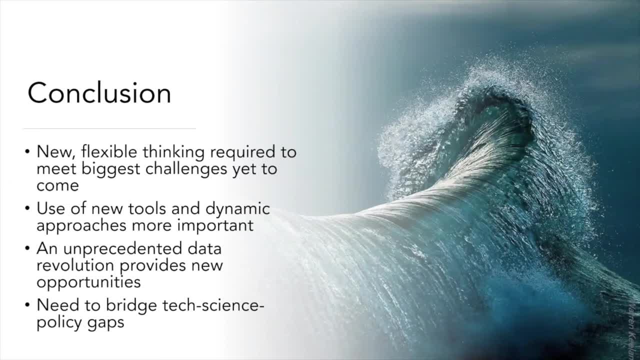 we have an unprecedented data revolution that provides us with the opportunity to meet these straight on. So for this, it is really necessary that we are aware of this and we are really keen to face this and also recognize that for this, we need to bridge the tech science. 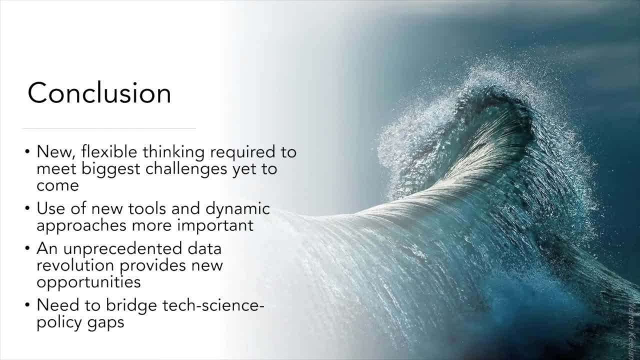 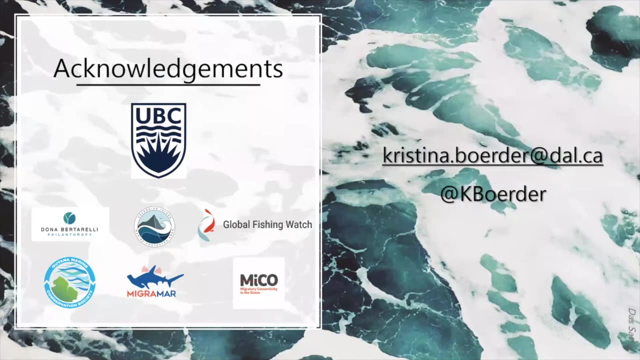 and policy gaps that we currently have, and then really start to implement and work with the data we have, create new data as we need it the most, and then move ahead together. I thank you very much for your attention, especially thank you for inviting me to talk here. 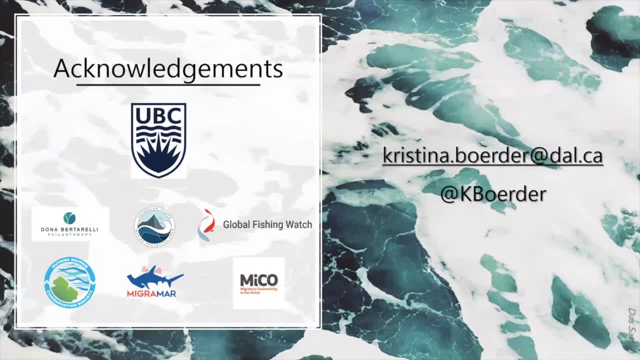 Of course, also to all the collaborators, and I'm happy and looking forward to answering questions. If there's anything you'd like to know, please don't be shy to send me an email or connect with me on Twitter. Thank you so much. 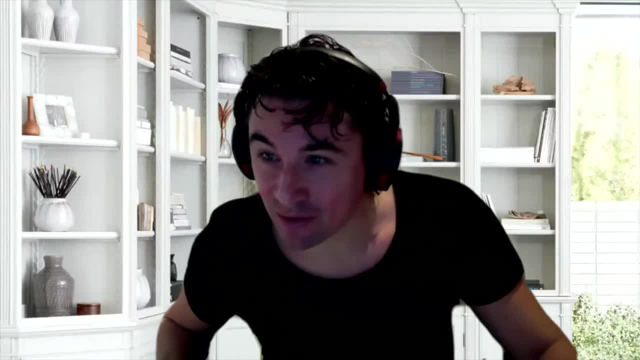 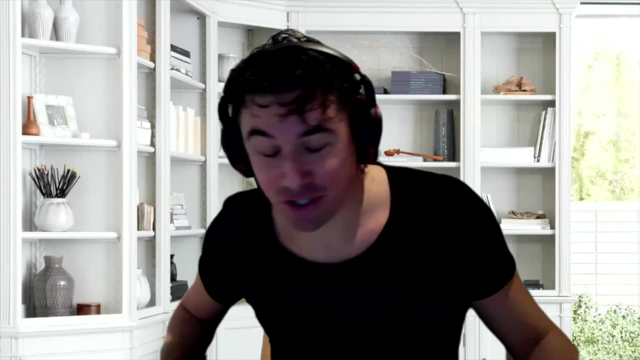 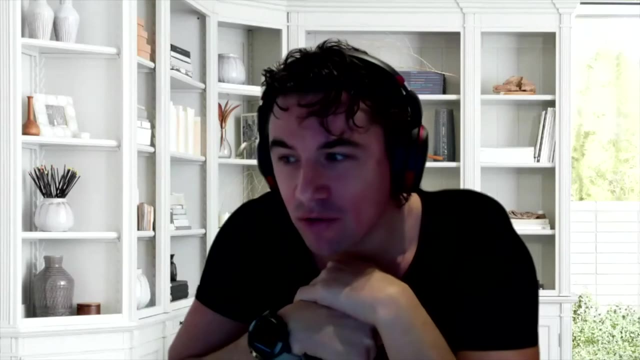 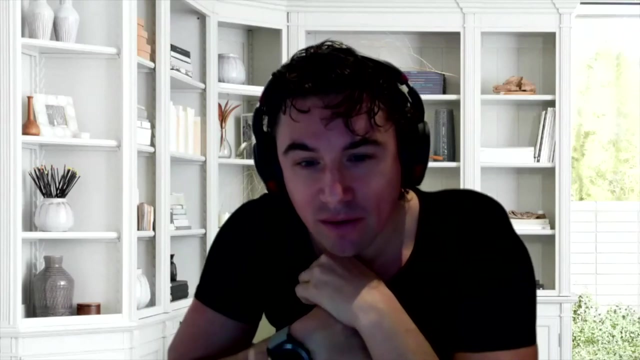 Thank you, Christina. We open now the questions and answers for part of this talk. I'm going to start with a simple one. With all the developing a tool to create potential new areas for MPAs in the world, That's the ultimate goal. 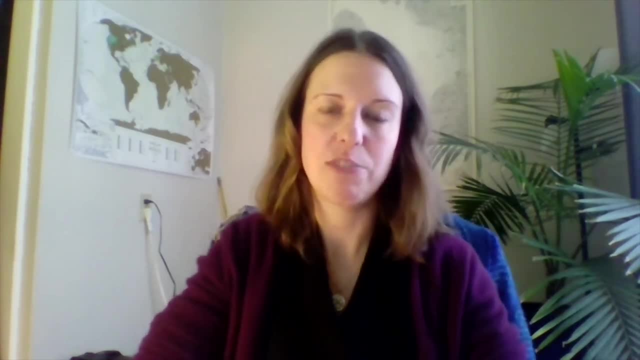 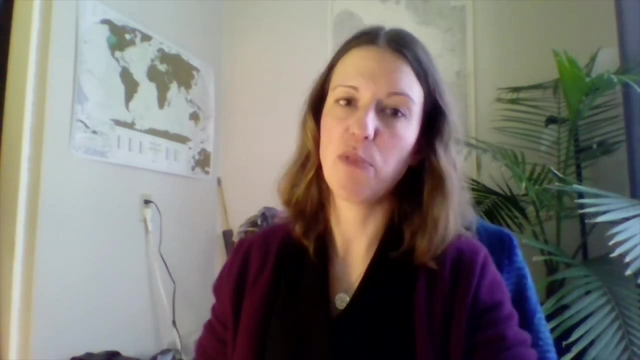 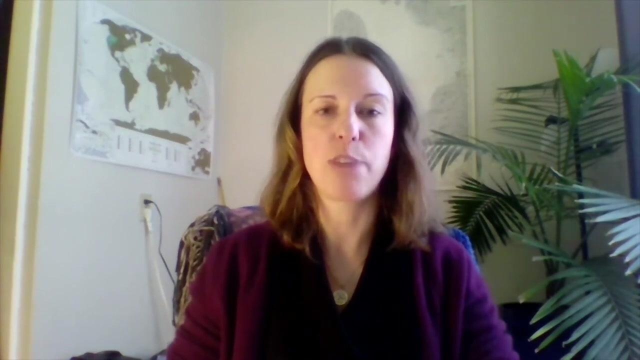 The name, the Marine Reserve, is a bit misleading. right now We really aim at marine spatial planning and to support that, And of course there's a big ongoing debate on where marine protected areas should be cited, What range or what spread one wants across. 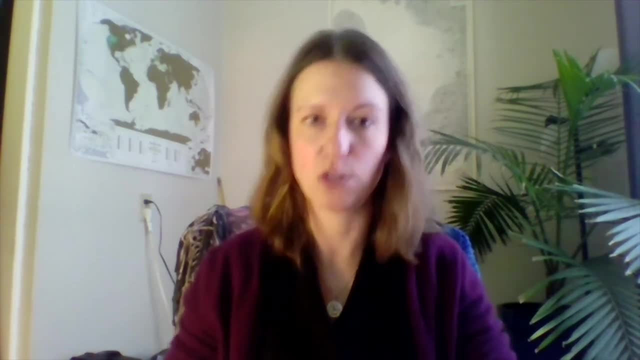 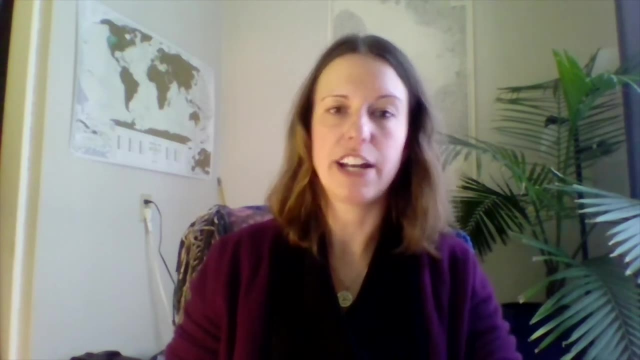 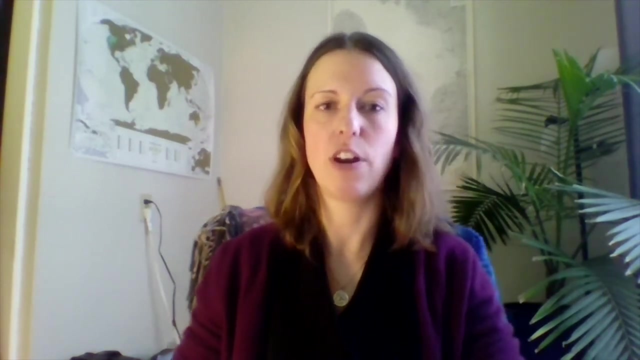 for example, different gradients of human use, or I've shown the examples of different climate scenarios. So we really aim to provide global data on this end and a broad understanding. So this can be work on this can be facilitated and empowered And, as we've seen with other, 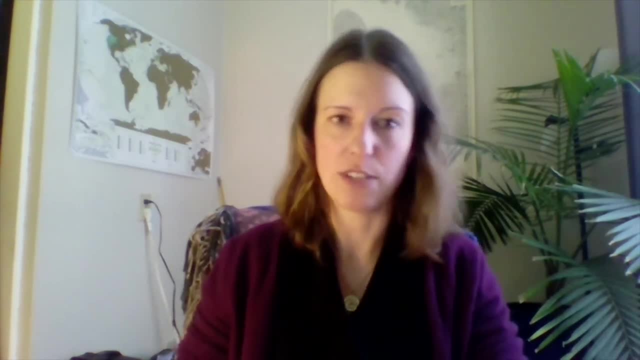 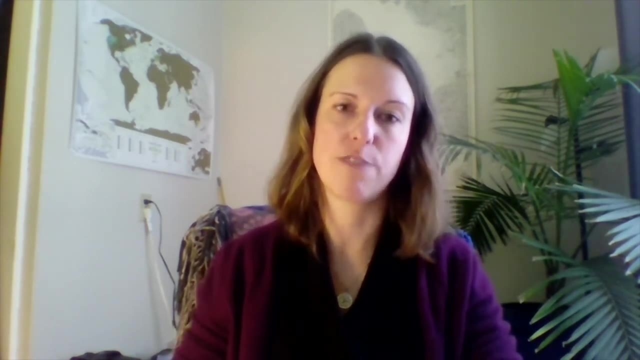 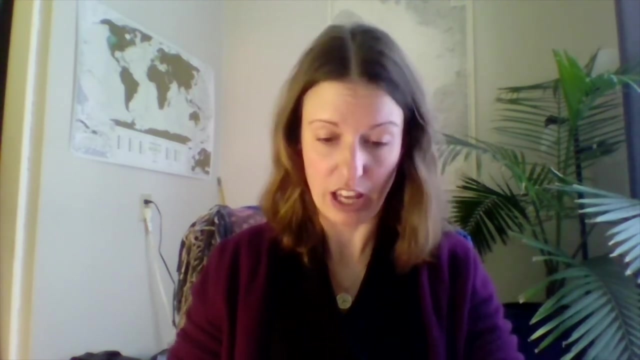 I agree with other objectives in mind we have. we have not really gotten especially where the climate change factor is considered a good spread of where areas are located yet. So, yeah, we really hope this is this kind of that, this kind of work can. 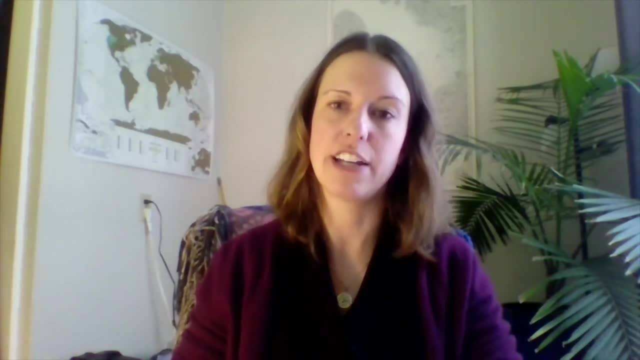 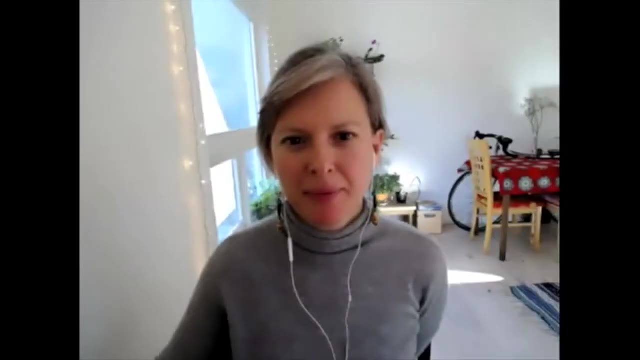 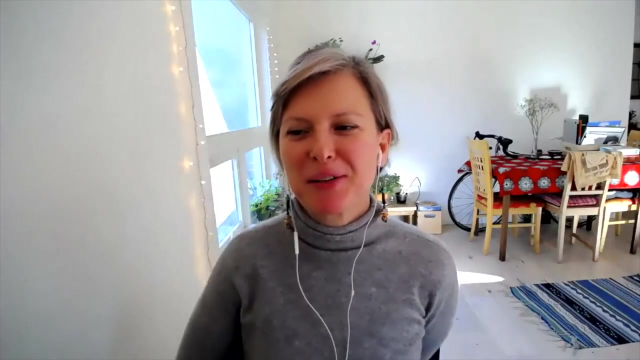 can get more clarity and more more data and add to this discussion. Thank you, Thanks, Christina Whilst. we let other people think of some questions, I'll jump in and ask one as well. I was just curious because I really liked how you 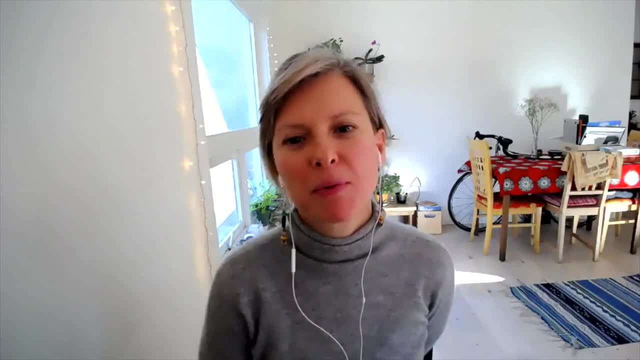 how you introduced the work that you do from you know, going from a reactive to a sort of more proactive approach and also linking the science to the, to the actual action. So I was just curious- and this is perhaps more of like a 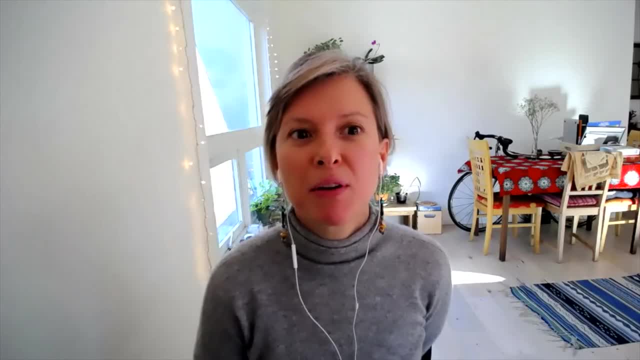 a personal reflection- how the action environment- so let's say policy makers or corporate players- have responded to some of your work. So you know some positive interactions that you've had or some surprising reactions that you have and how those have been communicated to you. 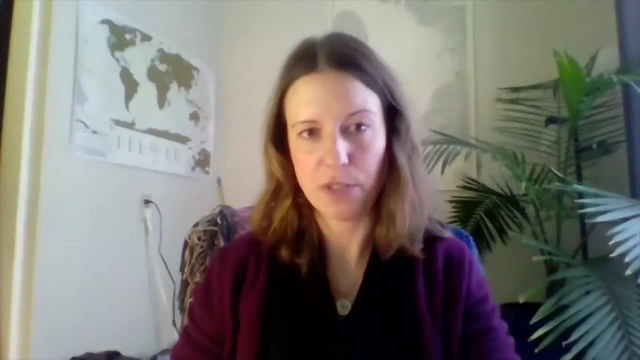 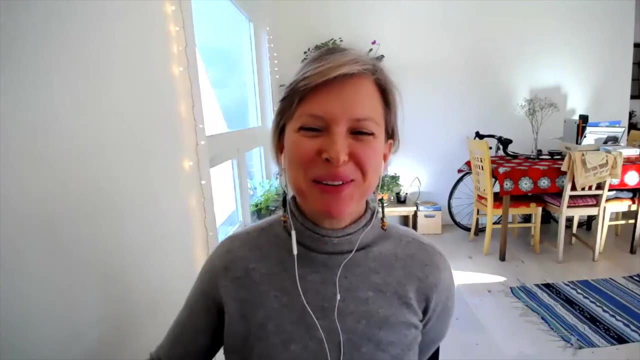 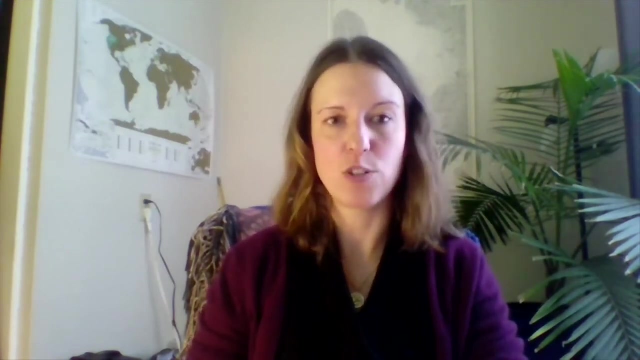 in that environment. So, specifically for policy makers, you said you can pick. you can pick policy makers or you can pick corporate actors, whichever one you want to highlight. I think generally we've gotten very positive responses to an approach like that, because most people 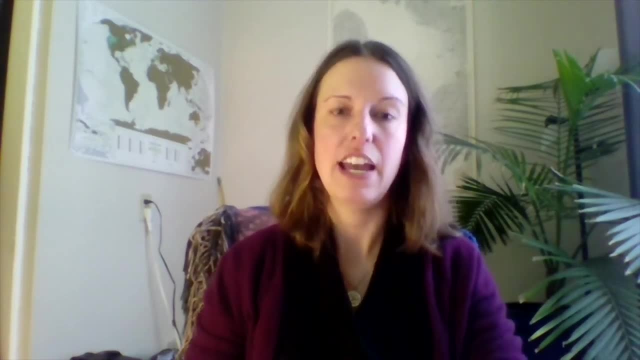 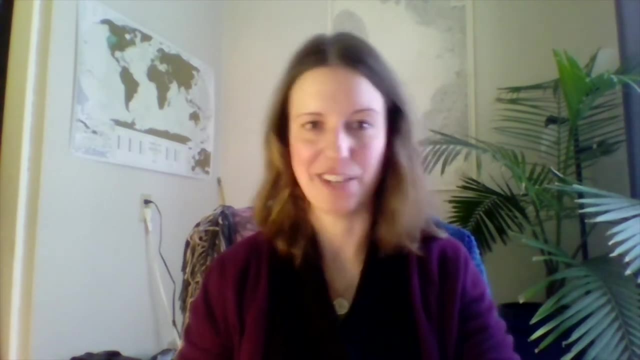 especially people who have worked with this type of data, can really relate to the amount of data that is there, but to the difficulties, if I phrase it like that, to really use it and access it, and how long and how much knowledge it really takes. 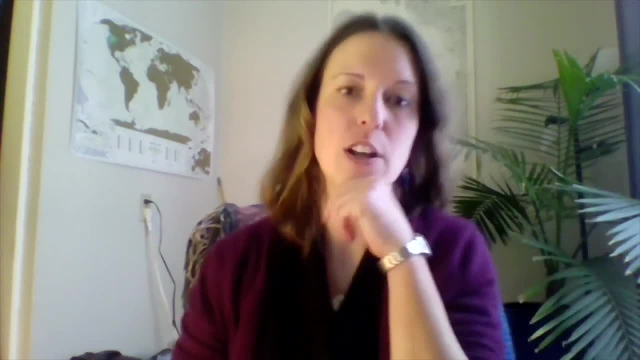 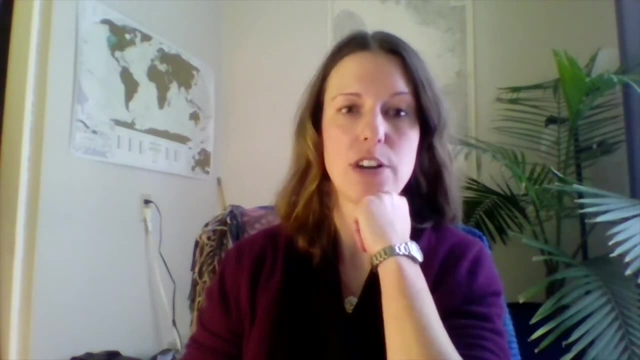 And this is even in areas where there's a lot of access and a lot of training and capability available. So really aim to also empower nations that might not have this kind of training and access, And I think most people have really had really see the type of use this would have. 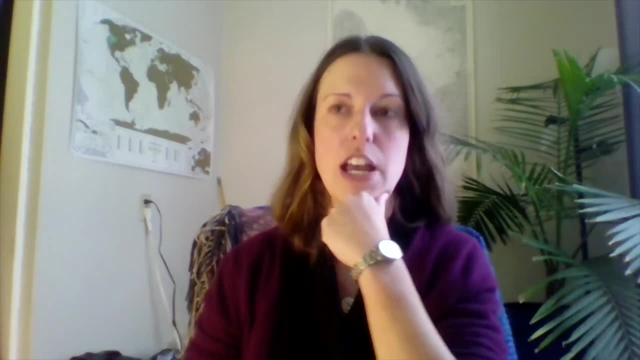 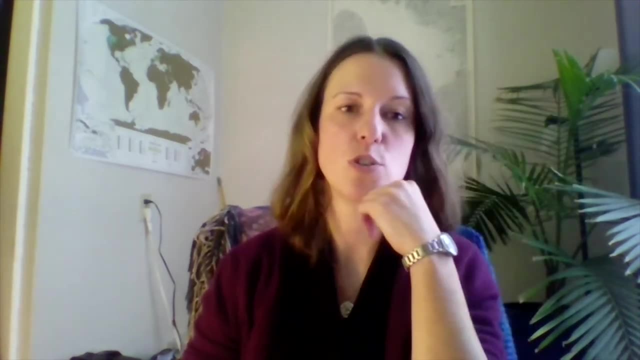 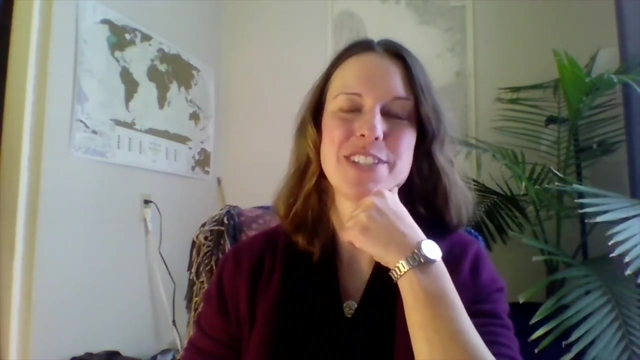 to answer the questions they are struggling with And we've brought together- I think it was- 29 different marine spatial planners and managers, from government down to NGOs- and actually not down to NGOs- And and managers of marine reserves, And when we talked about what goals. 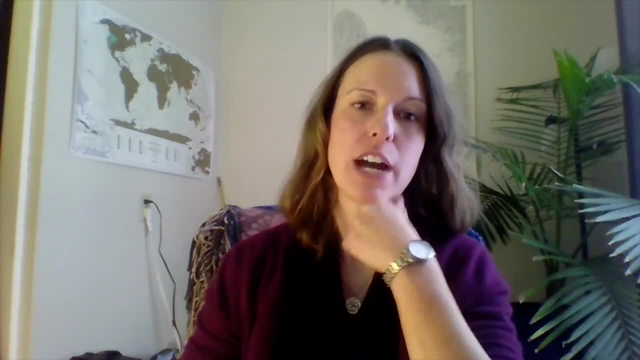 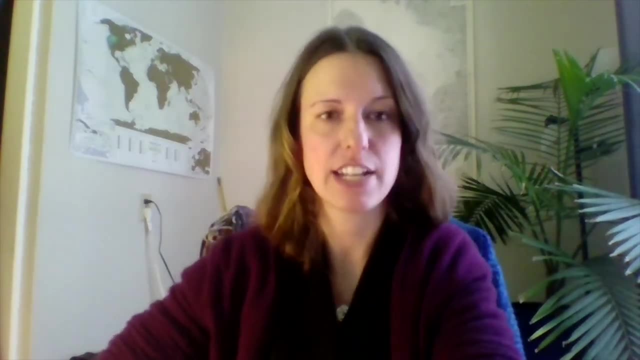 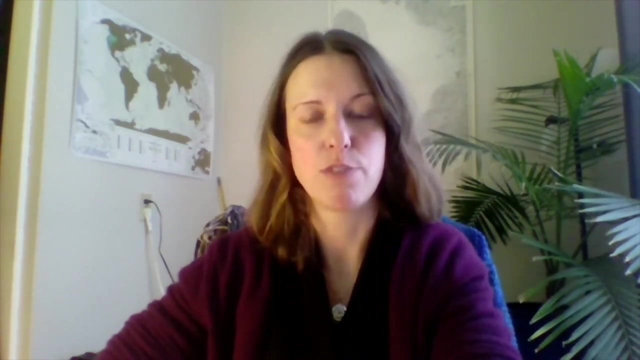 and objectives they had. we were surprised how much they really overlapped and centered around the use of certain types of data sets, For example, the human use, really to understand what are the stresses and pressures out there, to what types of data and types of science they needed. 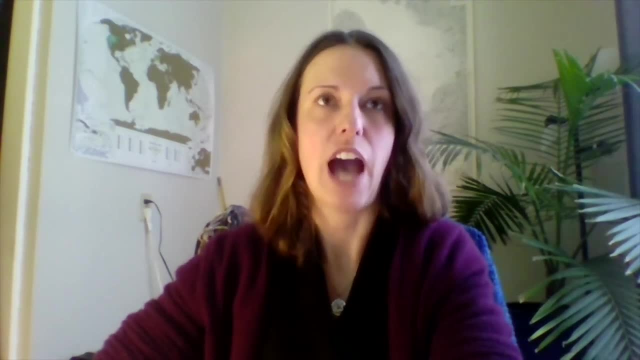 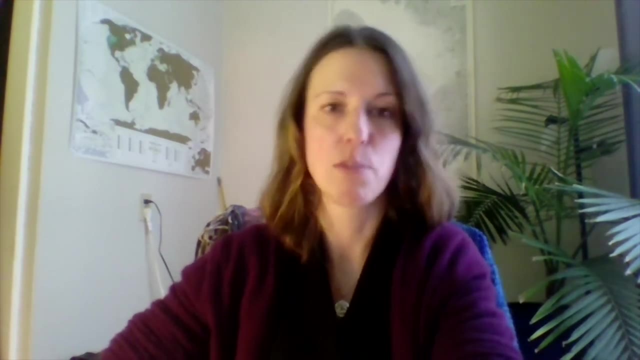 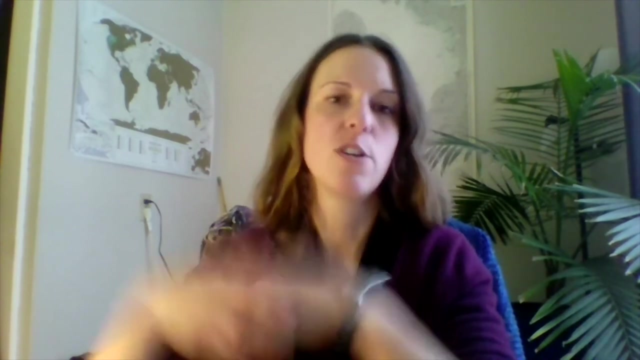 So I'm very positive going forward and I'm looking forward when this is launched and we start to work with more partners to, of course, learn more, because we developed this also really ongoing with the science and the work in the pilot sites to really learn what they need. 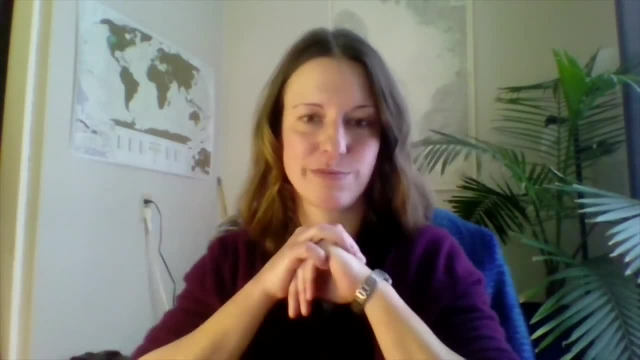 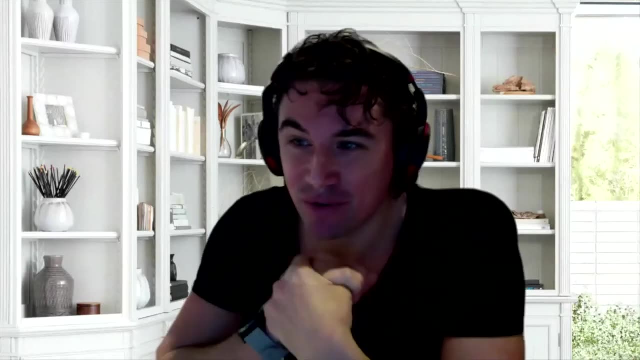 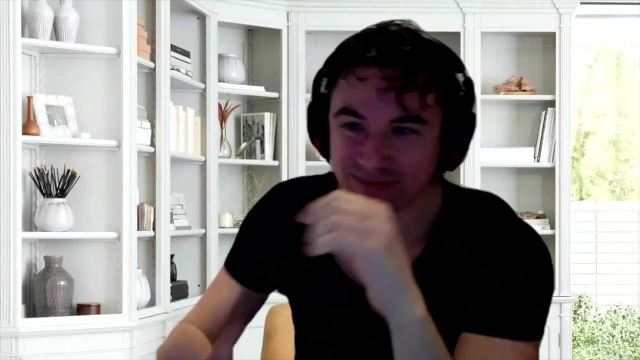 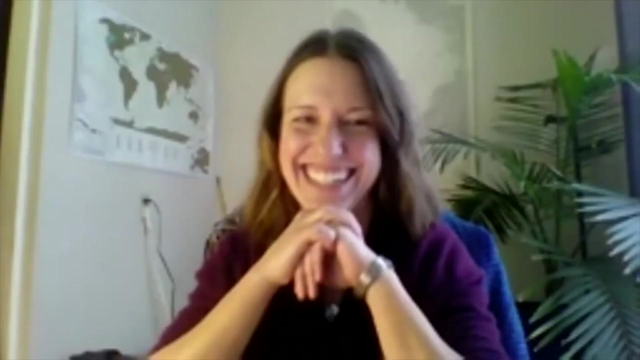 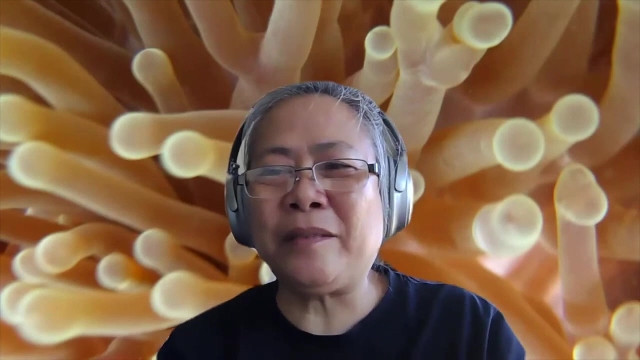 and then incorporate that accordingly. We have a question from Deng Palomares. So, Deng, if you can unmute and put your camera on And unmute, Okay, So, hi, Christina, I was a little bit confused. I sort of like missed the slides on the biomass models. 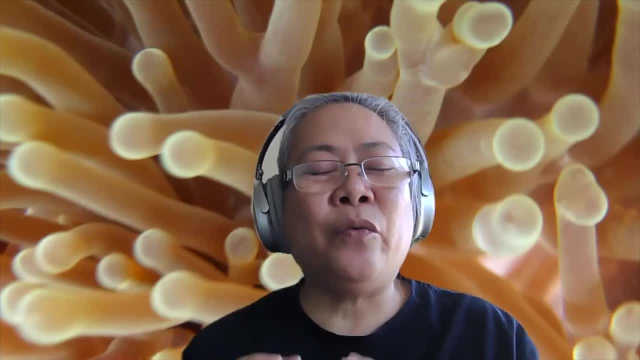 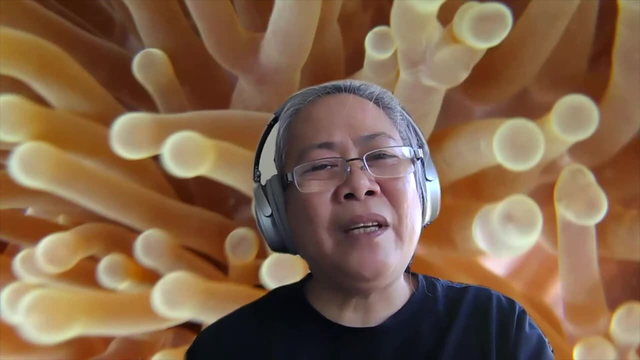 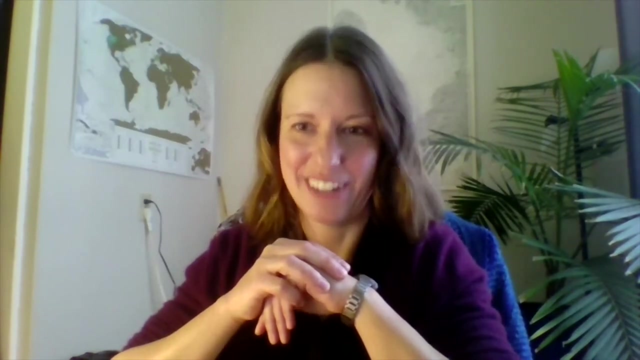 and I was a little bit confused about what kind of data went into estimating those models. So, can you, can you specify them again please? So I was. I would like to say I was not involved in that type of work. I know about these modeling projects. 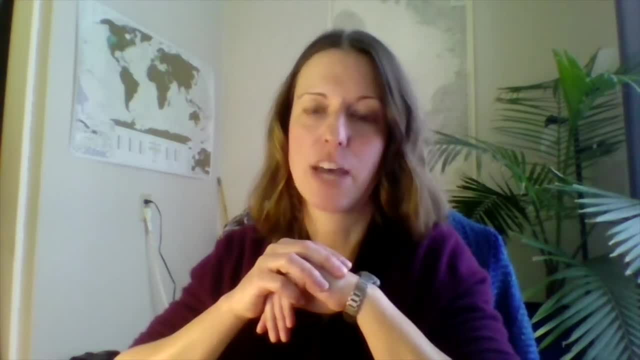 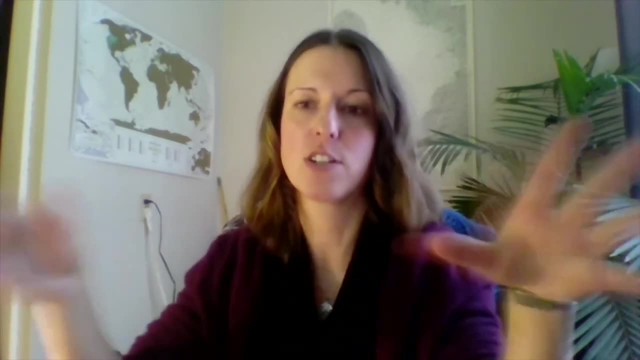 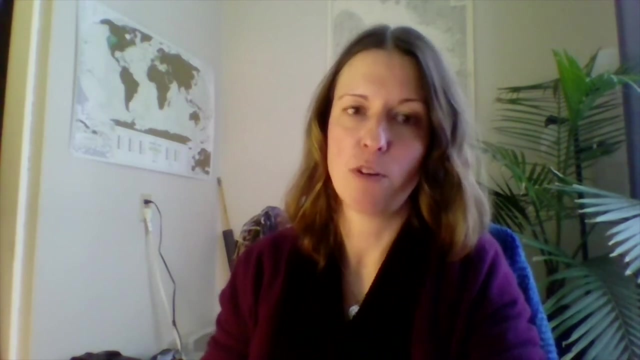 Most of them are taking different types of models coming out of the CMIP project into account, modeling on or combining a range of different models to find the best best fit of these models And specifically for the NAFO model that I showed the types of fisheries, catch and landings data. 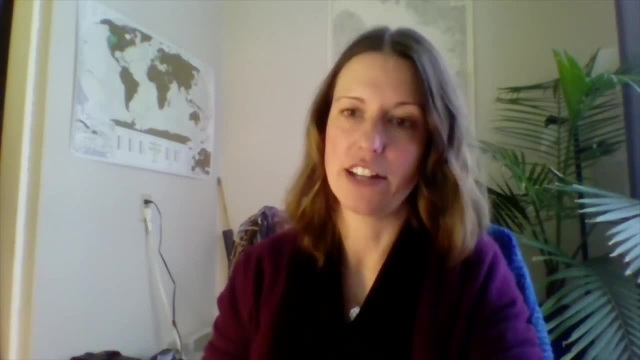 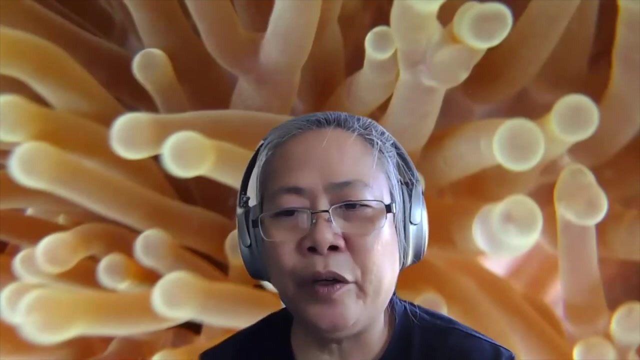 was included for that and then forecasted Under these different scenarios using these, this ensemble of models. But for further information I would direct you to those publications. Okay, So so if I understood correctly, they were models from assessments, correct? 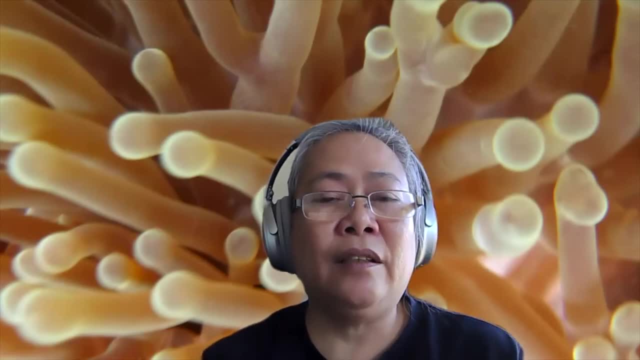 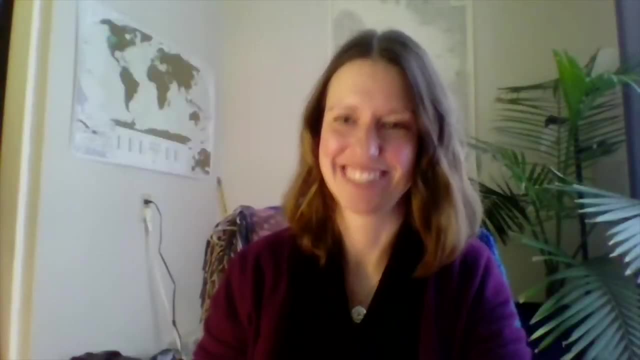 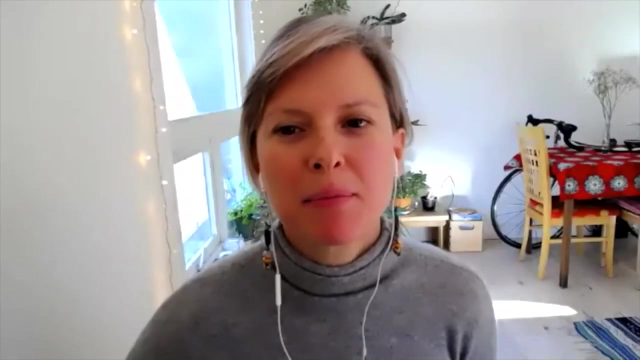 Like predictions of biomass, using references, say population references. That's how I remember it from those publications. Yes, Thank you, And Leonid Petrov, I will go to you next, but I just wanted to quickly. Christina Salome brought up that it would be great. 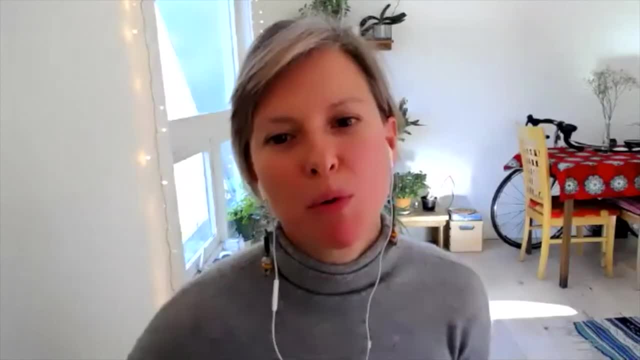 if you could share the link to the Galapagos report please, So we can figure out a way to do that. But just there was interest in the Galapagos report that you mentioned, The publication itself. Maybe I'll let her follow this up with you directly. 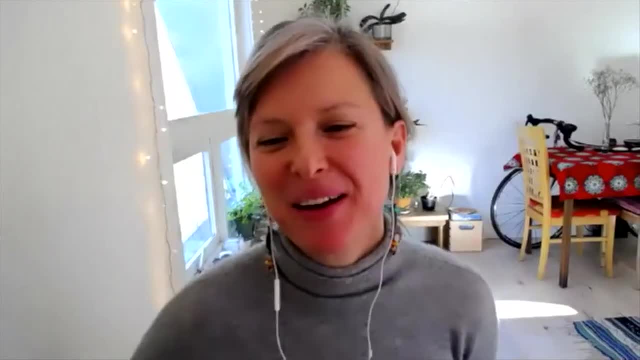 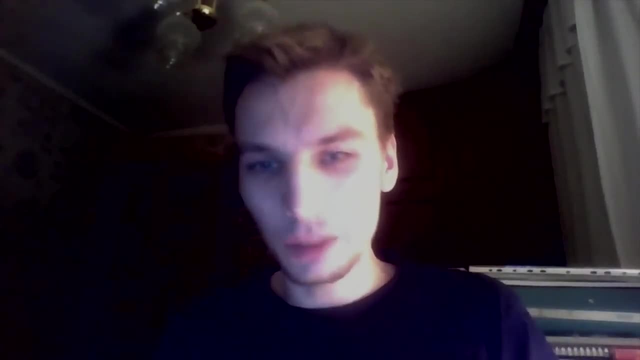 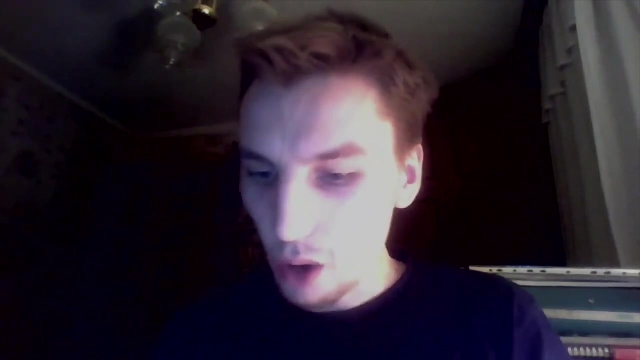 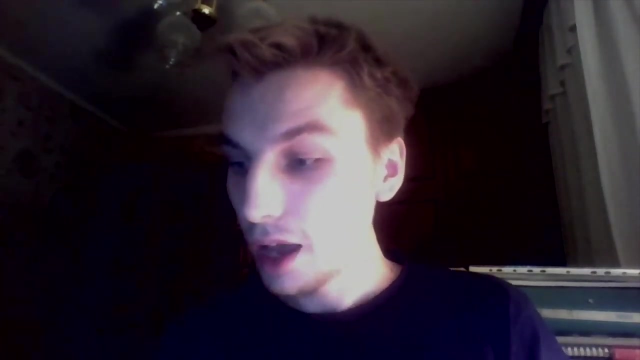 Sorry. So, Leonid, if you wanted to. Good afternoon. Thank you very much, Christina, for your interesting report. I would like to ask about noise pollution and its influence on the marine species. I'm right that the most vulnerable species are the most large? 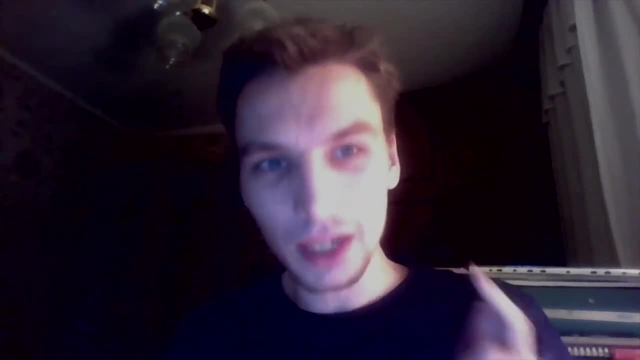 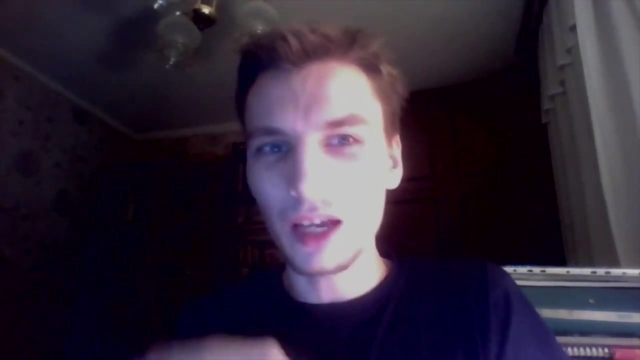 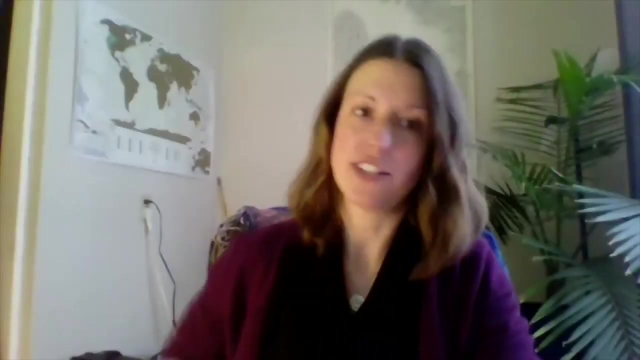 the most big in their size, species such as big mammals, As you mentioned. as you mentioned sperm, sorry sharks and other big species. I'm sorry, Thank you. Yes, they are certainly the obvious focus because, of course, the strandings- 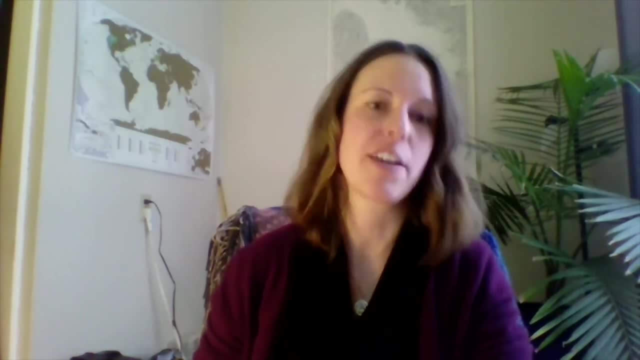 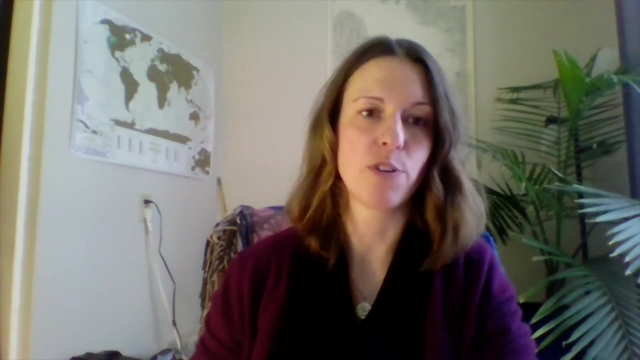 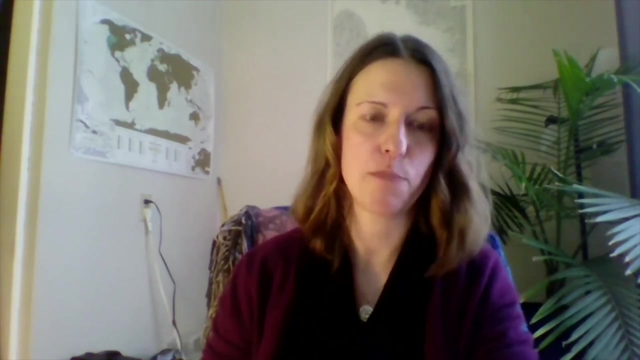 create a lot of attention and they are charismatic megafauna really. so people are concerned and they can be impacted by different types of noise. even if it's like, for example, louder than usual background noise, that can impact their echolocations, their hunting. 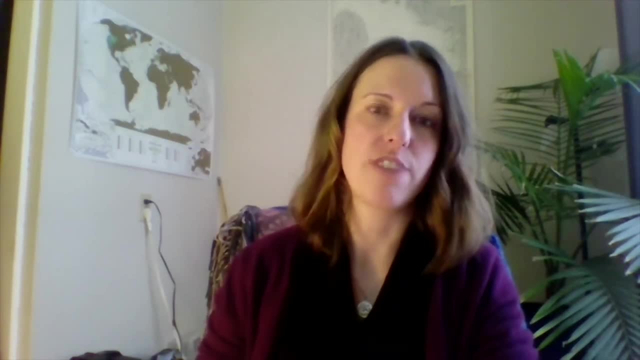 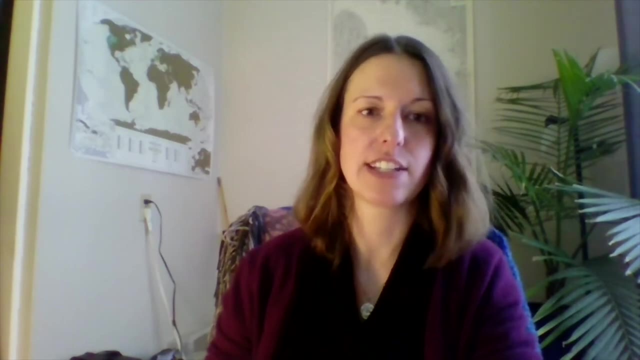 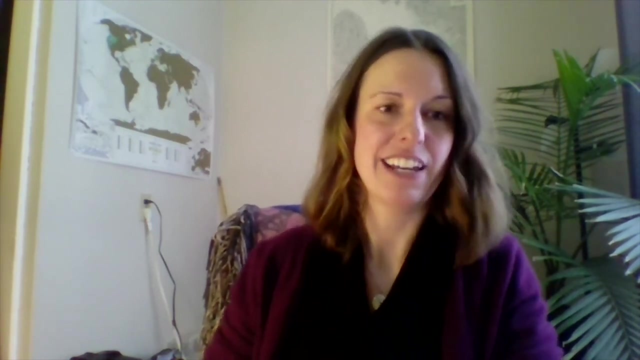 even result in strandings. to, of course, very direct impacts of high impact noises, such as the seismic testing which exceeds levels. I've read a comparison of for humans standing next to a starting airplane that really causes brain injuries, ruptured eardrums. 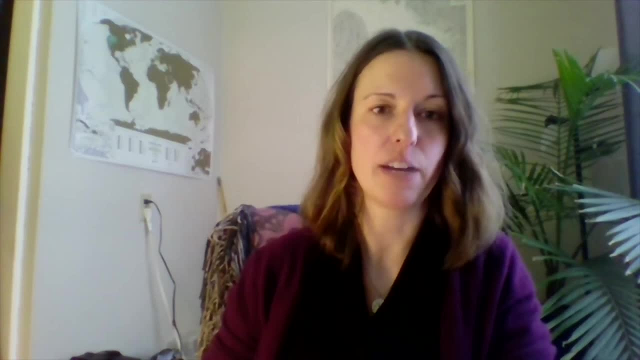 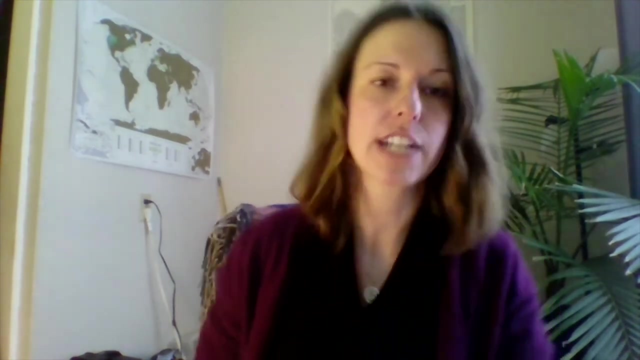 bleedings, not only for really cetaceans but also, as studies have found out, to fish, of course, down to the level of really harming plankton. So we're really at the beginning and I'm not an expert in ocean acoustics, but it's. 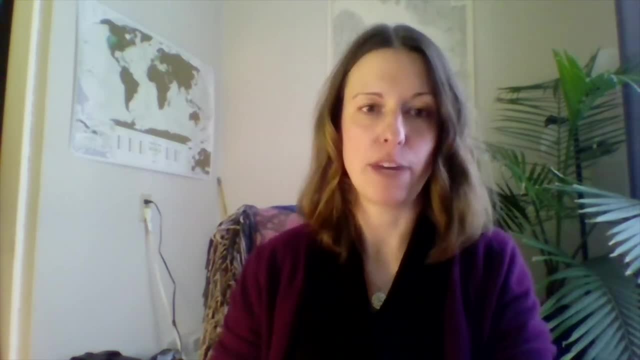 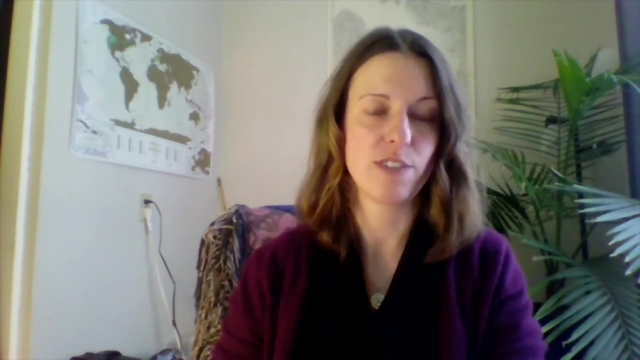 incredibly complex topic and involves incredibly complex modeling, but really, if we're talking about better protection and human impacts, this is certainly a dimension that has been largely- to my opinion, largely- neglected so far in conservation, and I'm really excited to see this as more and more of a focus. 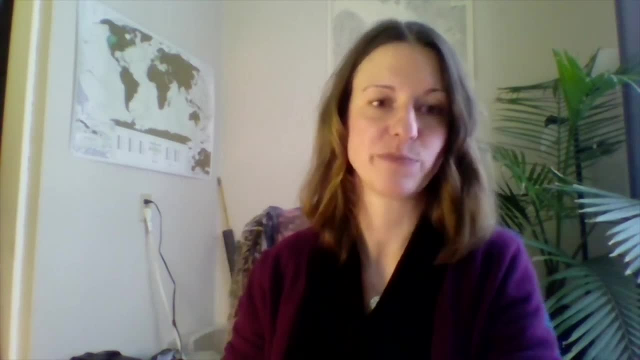 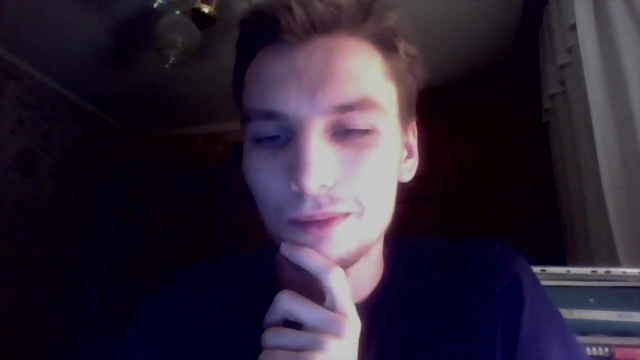 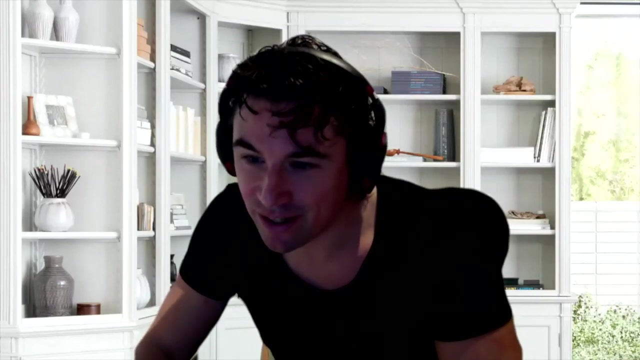 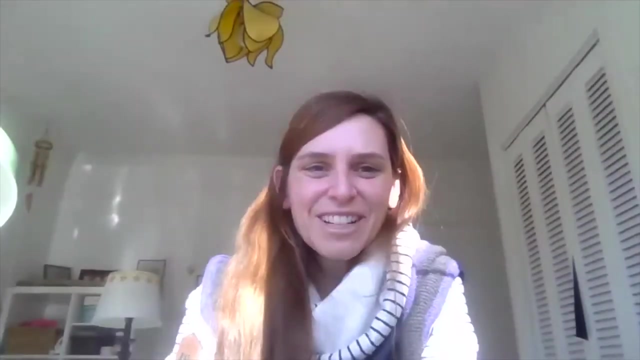 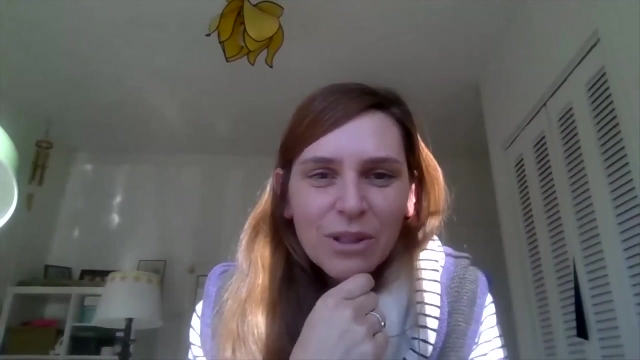 of campaigns and research. really, Thank you. Thank you. I think the next question is from Andrea. So, Andrea, if you can unmute and ask your question. Hi, Christina, That was a really interesting talk and before I ask my actual question on the topic of noise pollution, I imagine that to be really hard to quantify, since noise travels so far. Are there even areas in the ocean that are silent, or is it just a noise spectrum across the oceans? As I say, I'm not an expert on that, but having seen how this is being modeled, I don't. 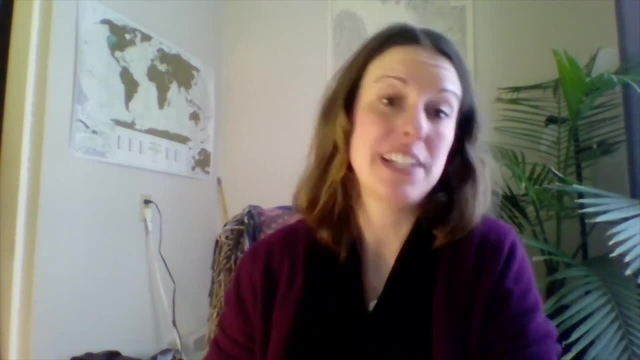 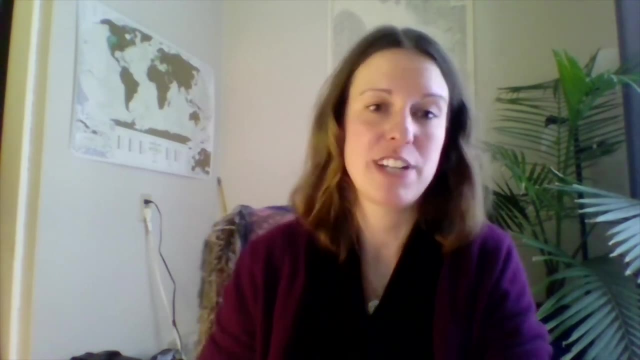 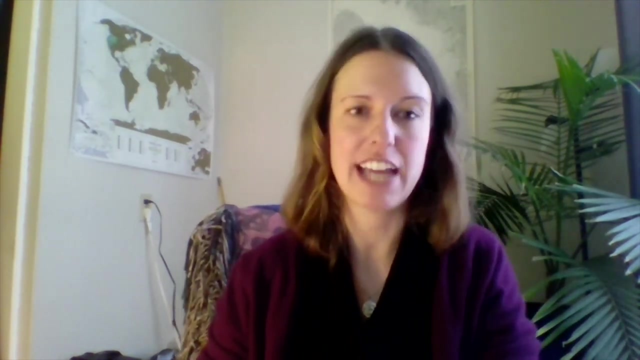 think any area really is ever quiet because there's maybe the deep sea, I don't know- but there's a lot of like ambient noise and natural noises that fish make, that different types of processes make. So the really really comprehensive models really take into account things like, of course, water movement. 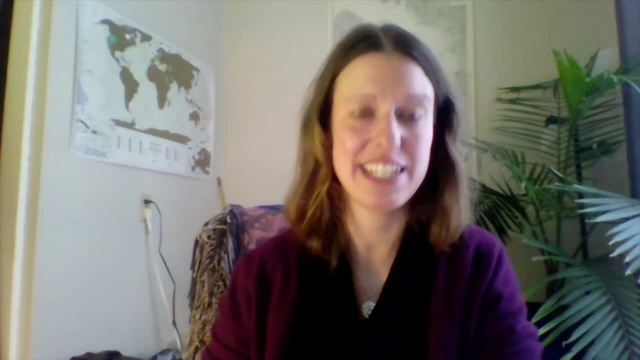 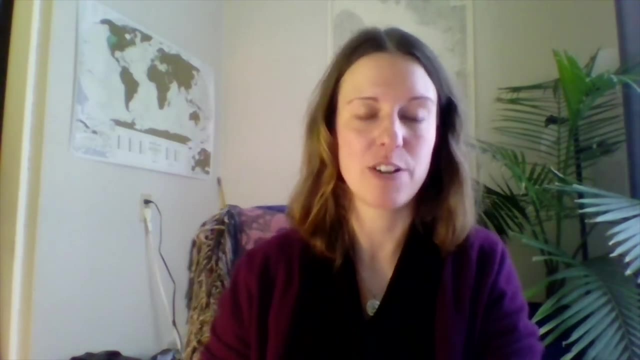 currents, density, temperature, waves, wind, even rain on water surfaces makes noise. So, and on top of all this ambient noise, of course, ships coming through or any types of testing and equipment use underwater makes even more noise. So it's an incredibly complex field and I feel 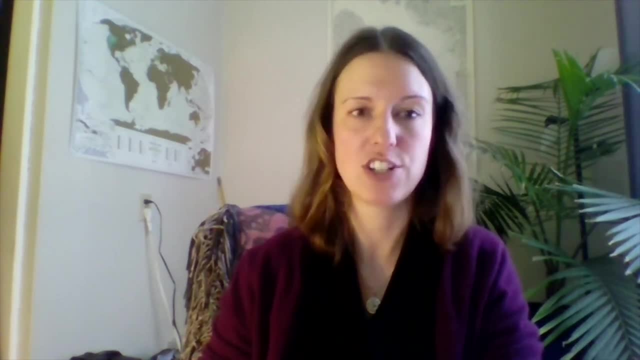 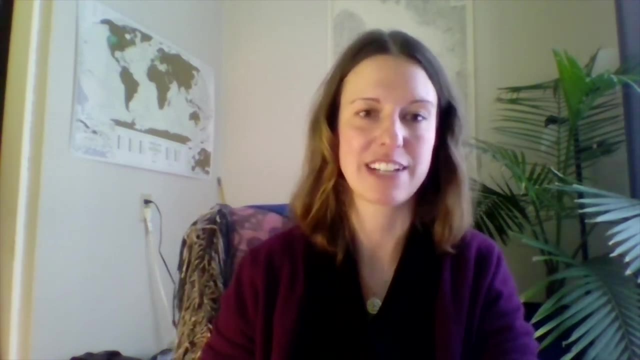 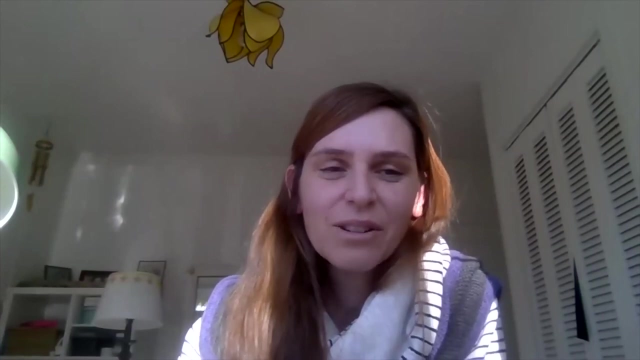 we're really trying to contribute some broad knowledge that we hope people then take into the areas of expertise and run with and and deepen on these kind of things. Okay, thanks. And then my actual question was if aquaculture was taken into account as a 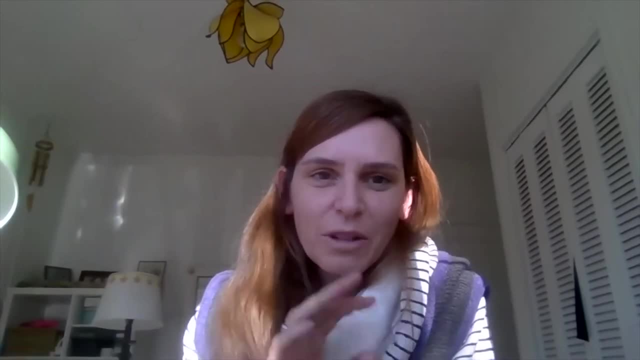 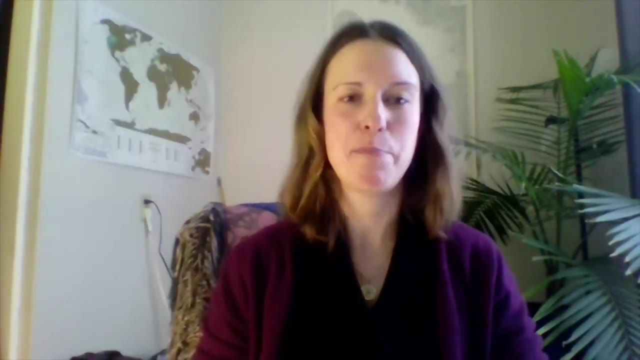 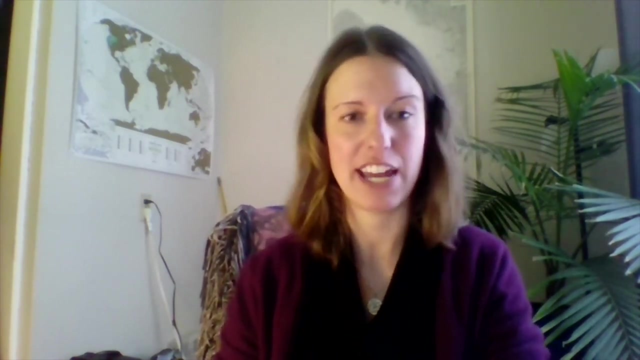 human stressor, especially in those last models of the global fishing wash that you were showing? Yes, very good question. certainly we have a big folder called aquaculture, but so far, with the pilot sites we have, it has not come up. We expect this to change as we take new. 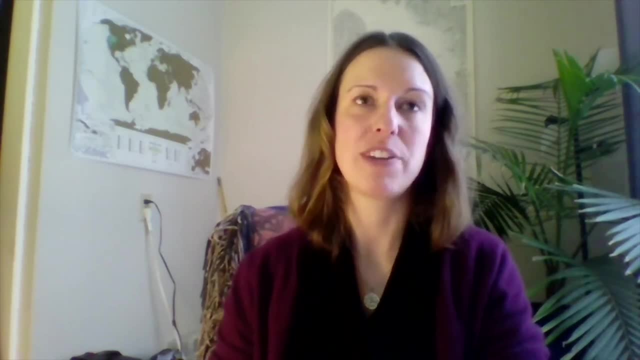 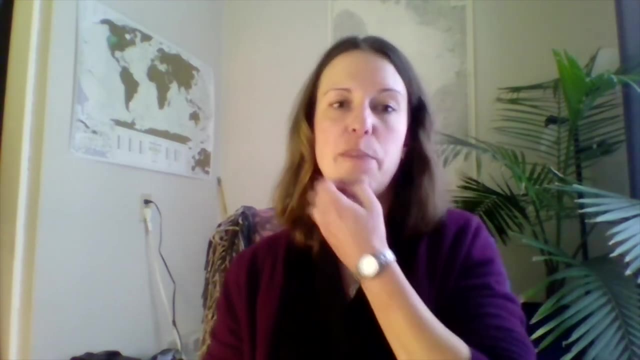 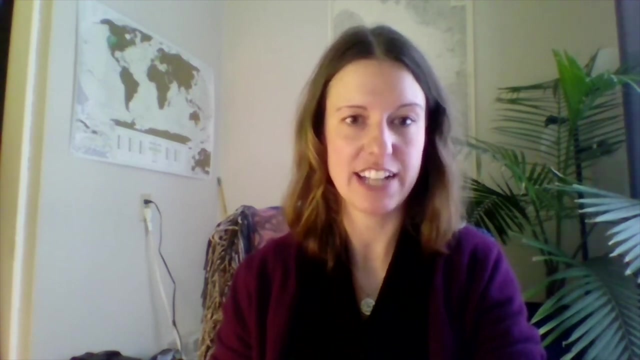 pilot sites. So with that, we'll be doing some digging into how available data is on aquaculture sites. We're thinking about trying to use a proxy. which are the vessels going to aquaculture sites to use this as a location if we don't have? 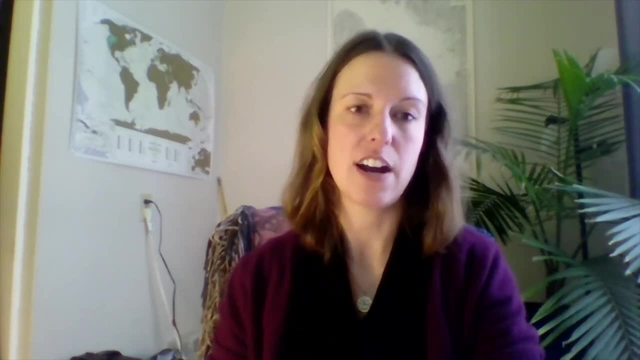 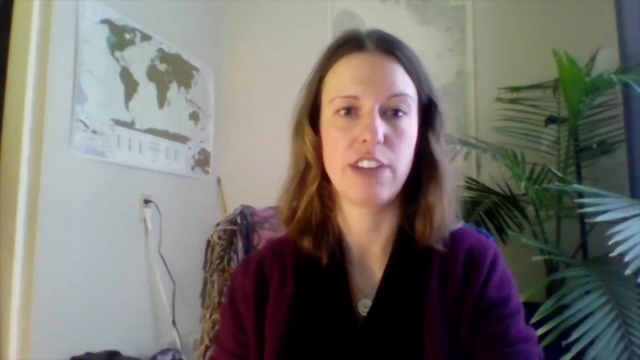 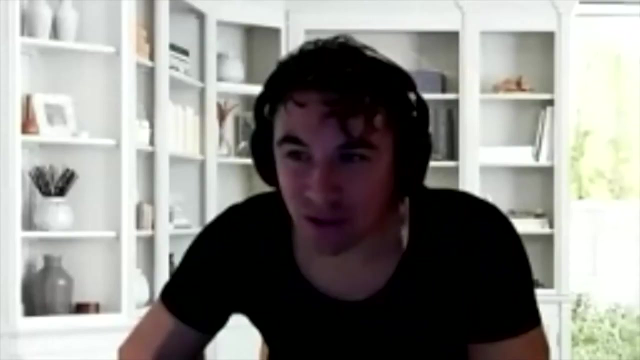 data on where these actual sites are, to at least show that there's human activity in these areas. But it's certainly going to be one of the areas of discussion. Cool, Thank you. The next question is from William Cheng. So, William, if you can unmute and put your video? 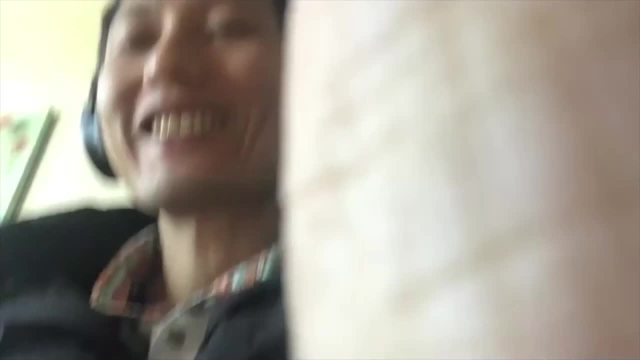 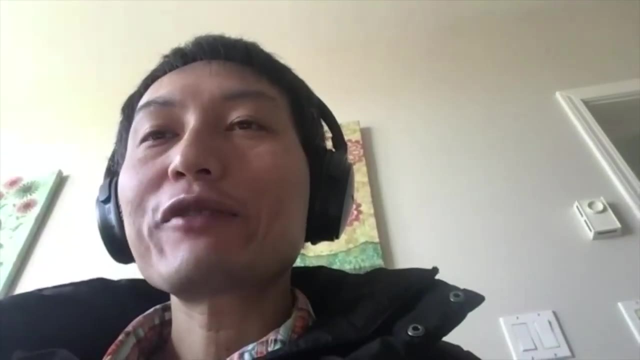 Hello, hi, Christina, It's great to hear your talk. It was a very excellent talk. Thanks very much. I have a question. So you have done all these amazing scientific studies, and a lot of it are very policy relevant, And so I just want to. 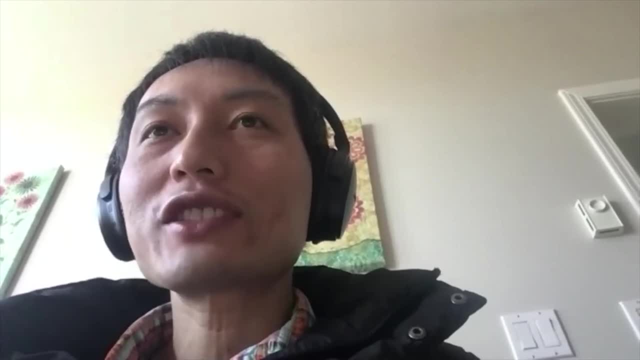 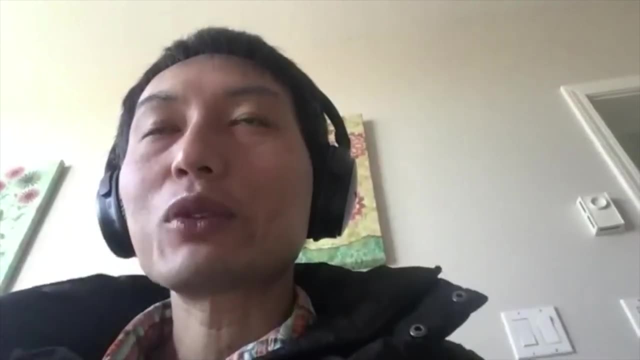 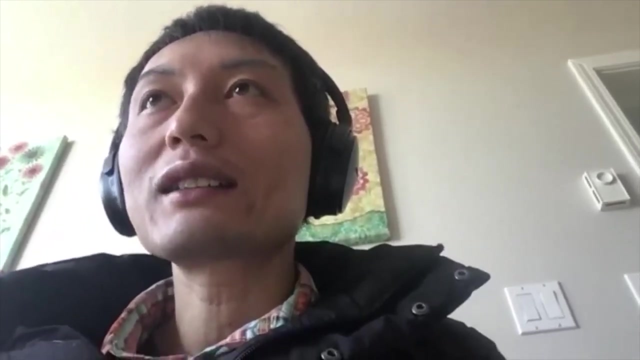 ask whether you can share your experience with us of what strategies that you think work best in making sure that all these amazing scientific work can help with supporting policy discussions and that there is policy makers would understand the science and then be and also use the tools that are available in those. 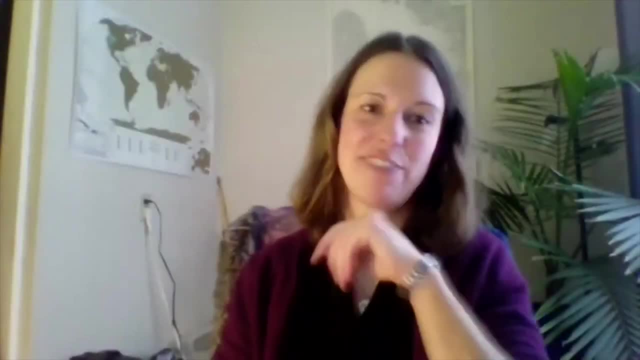 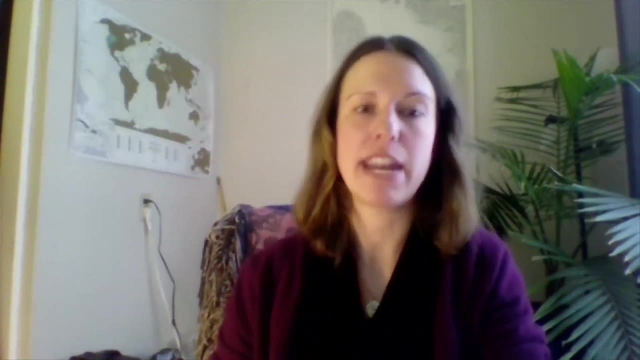 discussion forum. Thanks very much. Excellent question. Right on the money with that. This is something we really also want to, or actually, that mainly motivated the creation and the work on this tool is to facilitate the access to the outputs of the scientific work, because I think it's. 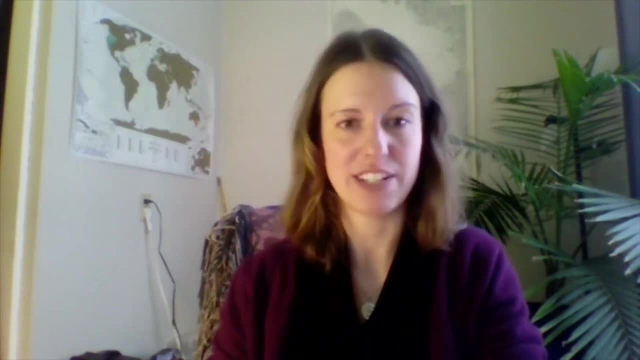 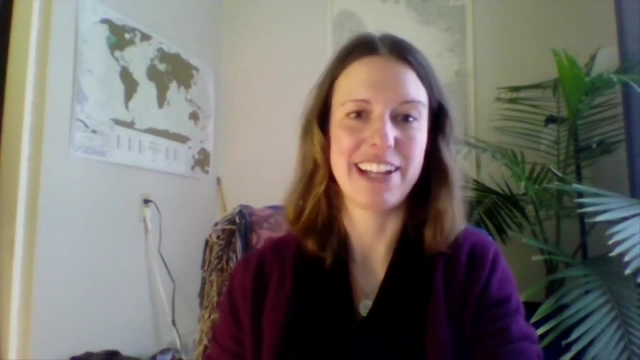 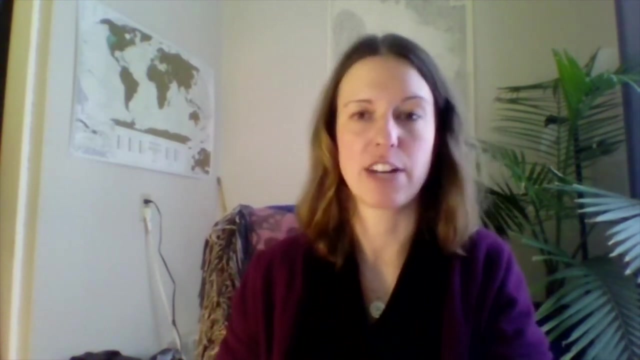 as said, it is understandable that managers who have no background in the field, necessarily, or even policy makers, are slightly overwhelmed, I would say, when they get presented with model outputs or the complexity of it, and then, of course, the uncertainties that are connected, and we really try to 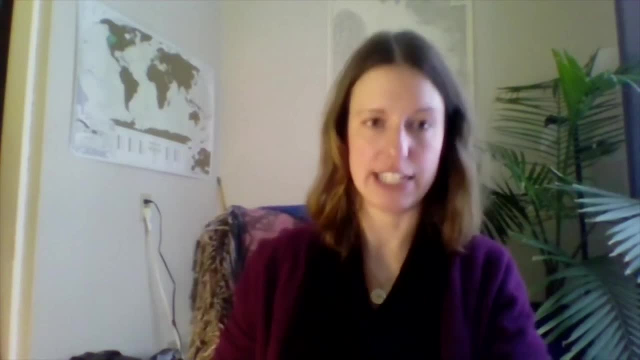 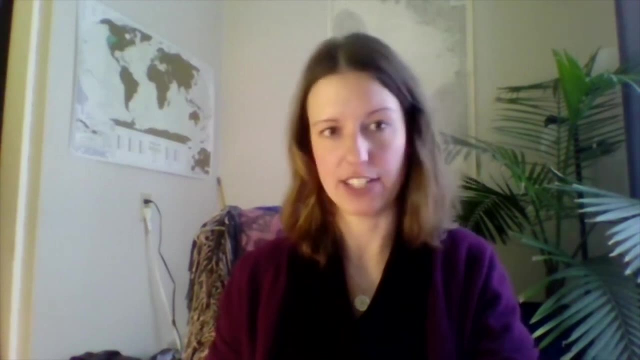 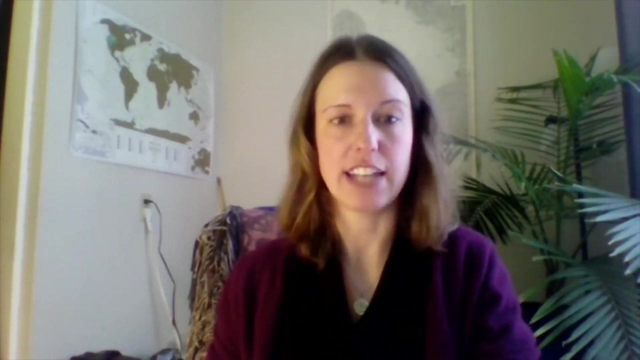 make this more approachable by having this tool that is very direct in its use and presents what a lot of the managers, and often policy makers, need, which is a lot of the research that is being done in the field, and then really, when that kind of stage 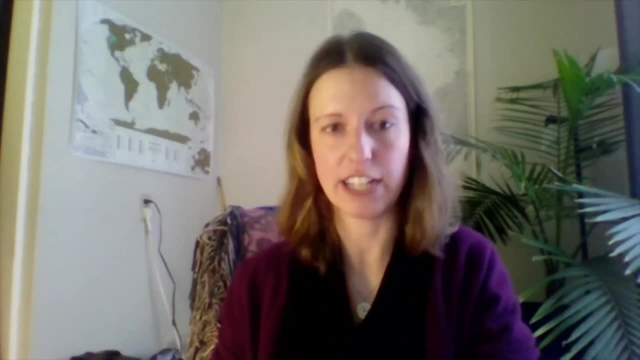 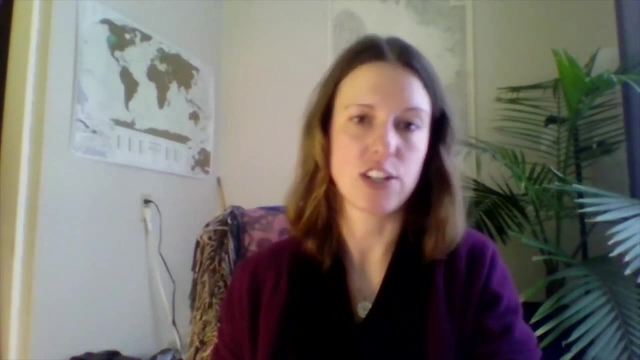 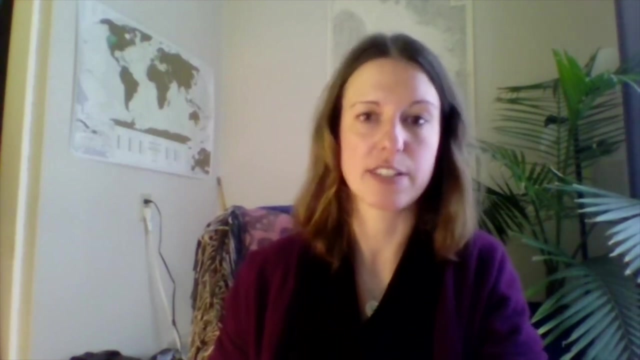 is set to be able to be reaching out, and we will have a separate page where, of course, the data sets and the accompanying publications are linked, but also aim at providing this as a platform for understandable science communication and I think this is really the key- that, for example, the 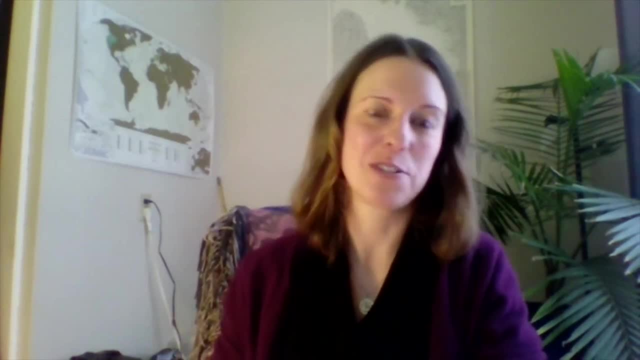 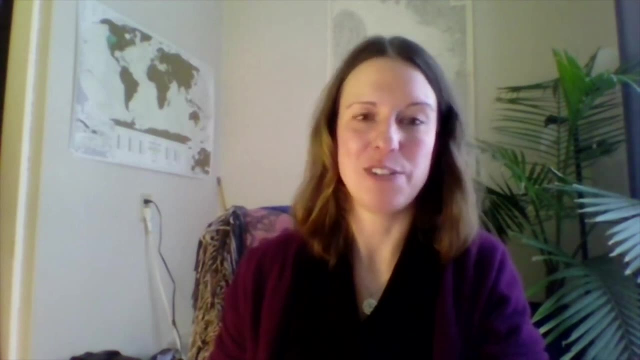 research that we are working on is a great thing, but it's like when I talk to my grandma, for example, about it, it doesn't mean anything to her. so but when I say, like this is really used by managers to understand how species move in and out, potentially. 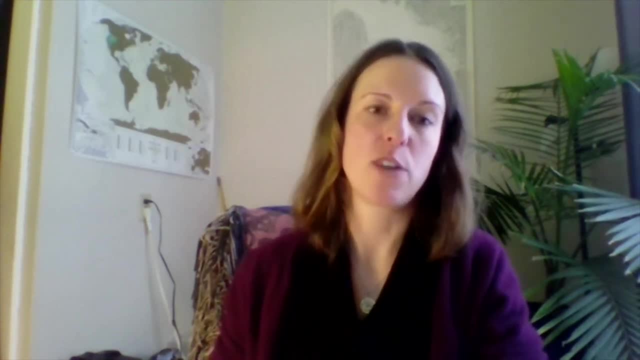 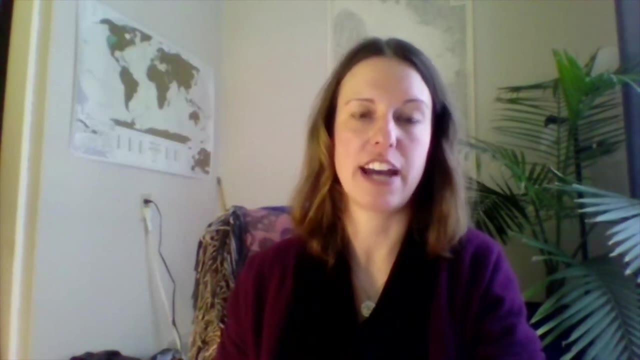 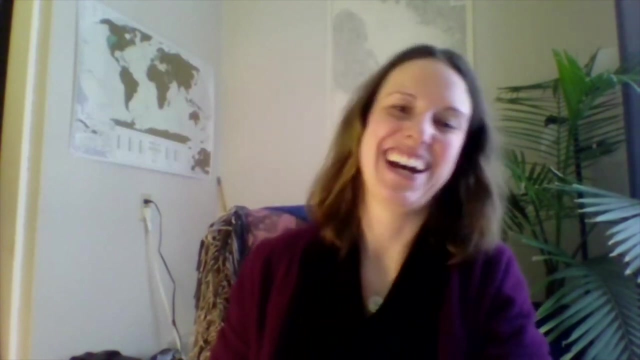 in the future and how they need to look out for them. this, of course, makes a whole different sense and really the application. this is why we focused on the application that I see transports the science here, and we hope we can develop, with partners like yourself, a strong platform to really 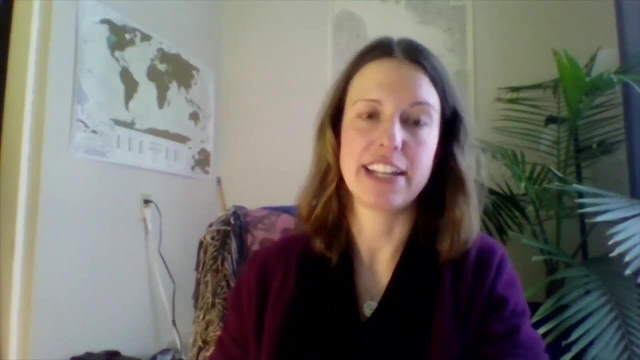 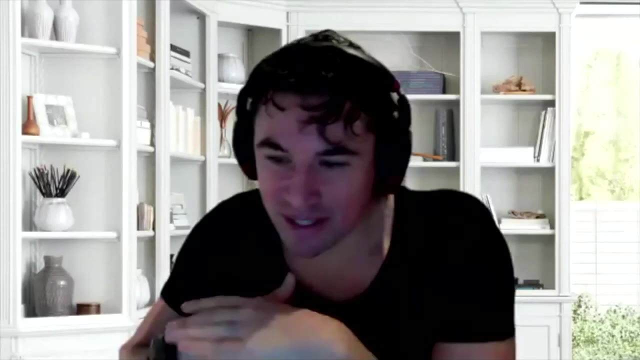 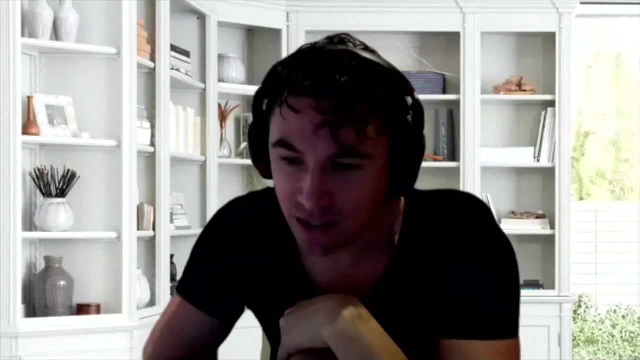 bring out that science and have it applied and then, through these applications, tell the stories of that. Thanks very much, Christina. Thank you, Christina. There is some suggestion from Emily Tukai from France, who just asked quickly: do you know the European portal for marine? 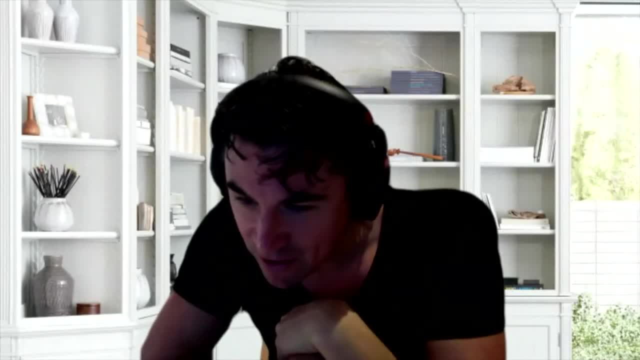 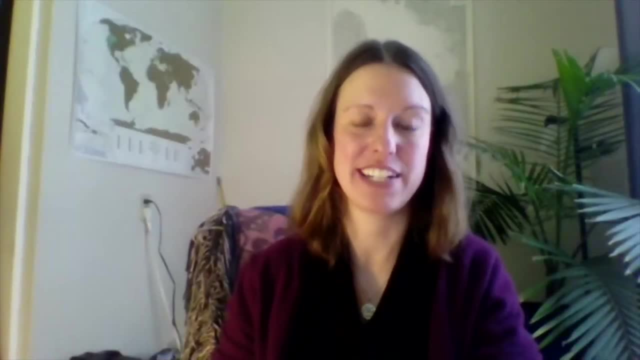 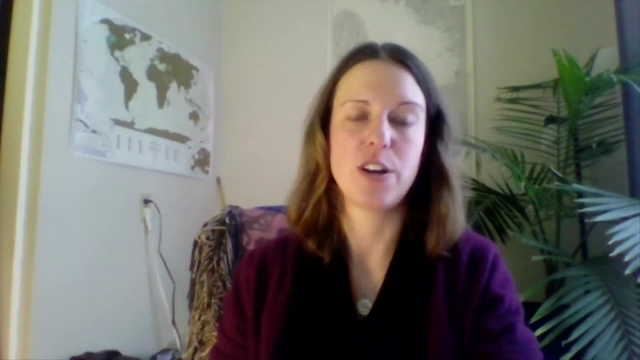 data called EMODNET N-C-M-E-N S. I do. yes. The Europeans are really exemplary regarding data transparency and data sharing and, of course, NOAA and the DFO, to a certain degree, are also doing good jobs at that, so we're really trying to.